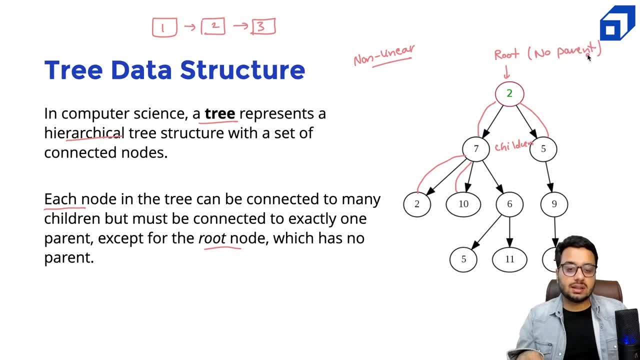 no parent Rest all the nodes. they have 1 parent right Now. because of this property. there will be an interesting observation. Suppose you are creating a tree in which you are going to have n nodes. okay, For example, I have 3 nodes here, So how many edges you will have Except? 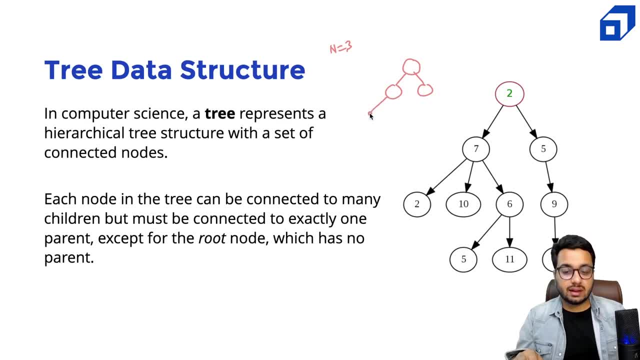 for the root node, for every node that you will have that you will add, there will be an edge. So there will be, of course, n-1 edges in the tree, right In any tree that you are going to create, irrespective of is it a binary tree or not. each node that 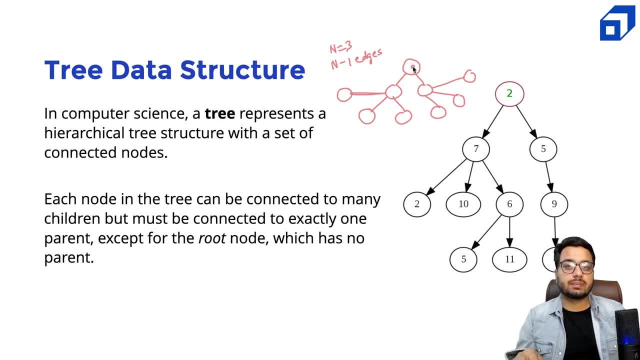 you add will add an edge in the tree except the root node. okay, So root node does not add any edge in the tree except the root node. If there are n nodes in the tree- there are- there would be n-1 edges. okay, Because root node has no parent. rest all the nodes that. 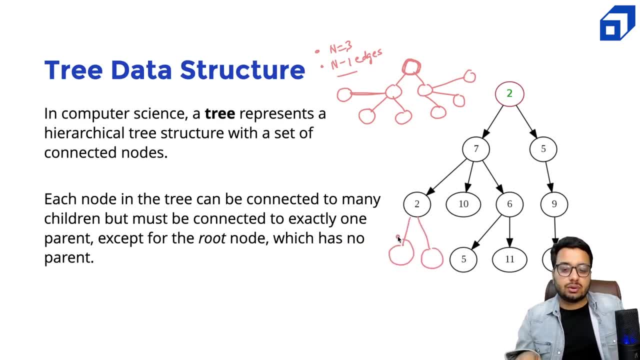 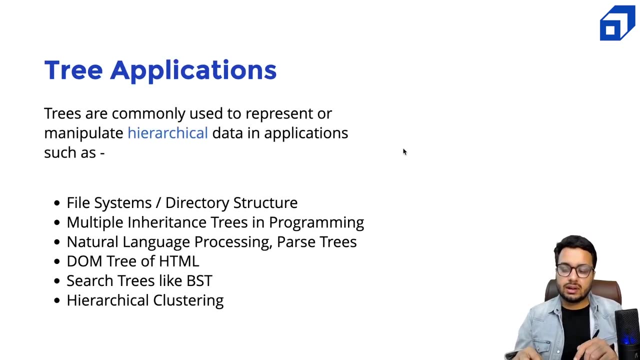 you add, They must be connected to a parent through an edge right. So this is an interesting observation, you can note. So in every tree there will be n nodes and there would be n-1 edges in the tree right. That is tree data structure. Now let us talk about where this 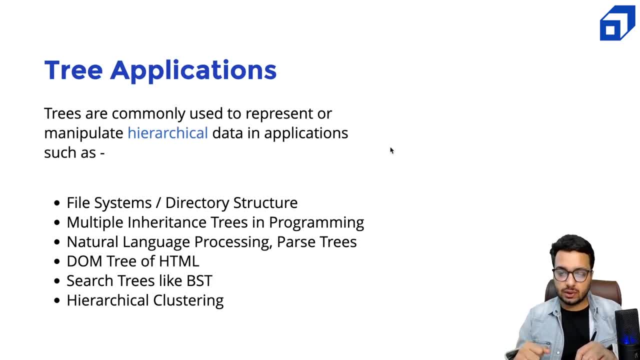 data structure can be used, how it can be helpful in computer science. okay, Basically, trees are used to represent or manipulate hierarchical data in applications such as file systems or directory structure. right, So all of you have worked with a file system before. So what happens in a file system? you say, okay, I have my PC In this. I have. 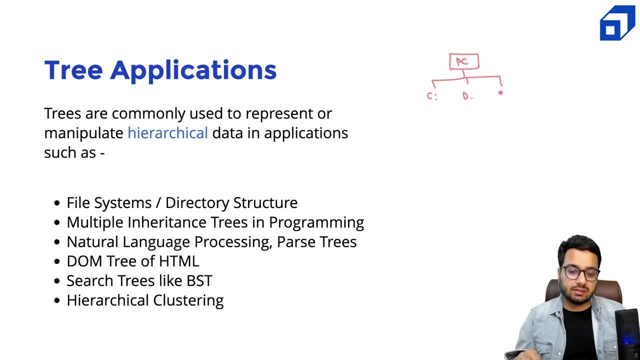 certain drives, T drive, D drive, E drive, and then inside this I have folders F1, F2, F3, F4, and here also I have folders. then I have subfolders, right, Maybe I have photos. 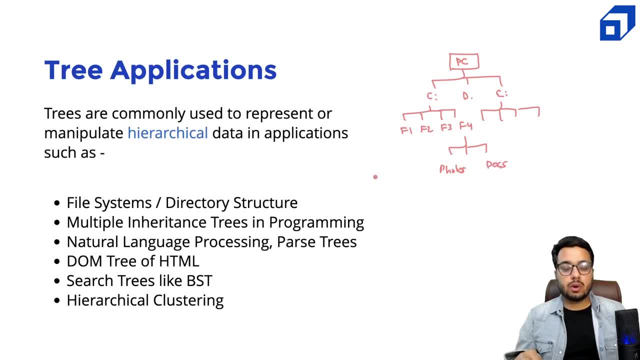 here. maybe I have some documents here right Now. we often do operations like that: okay, I want to move these photos from here to here, right? So what is going to happen? You are not going to copy this data. you are going to say, okay. 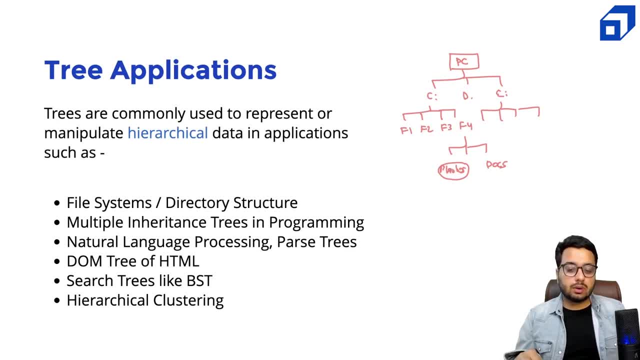 I will cut and paste. So if you simply want to move these photos from here to here, what do you need to do? You do not need to copy this information to some other part of the disk. You only need to change the reference. right. That, okay earlier, this reference. 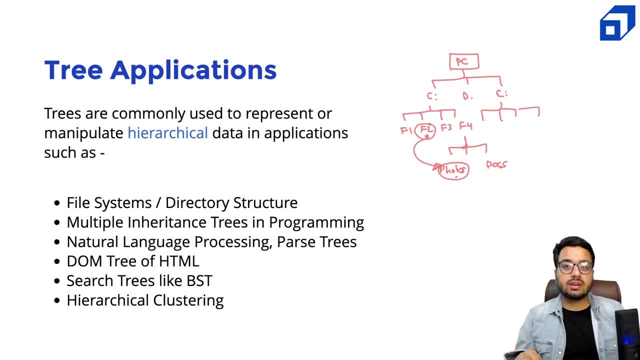 was stored by F4, now this reference is stored by F2.. Basically, the links right, The links to the folders and subfolders right. They can be easily changed if the data structure is implemented using a tree right. This is: 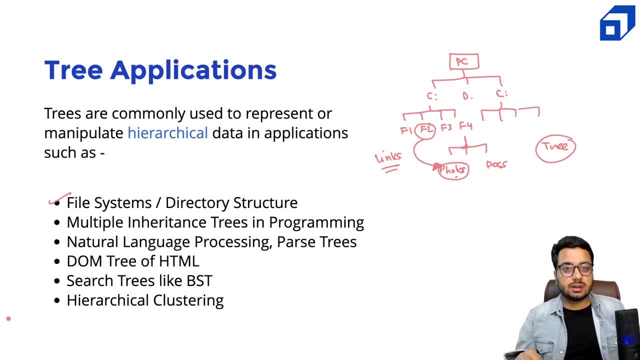 something we will discuss. right File system is a good example of a tree data structure. right, Multiple inheritance trees in programming. So this is used when you are using object-oriented programming concepts and you have a class C which is going to inherit from a class A. 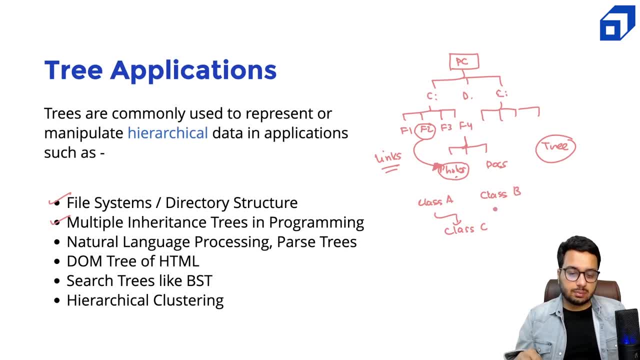 it is also going to inherit some methods from class B, right? So this is not exactly a tree, I would say, because this node, this is inheriting from two different classes. Irrespective of that fact, basically the trees are internally used. 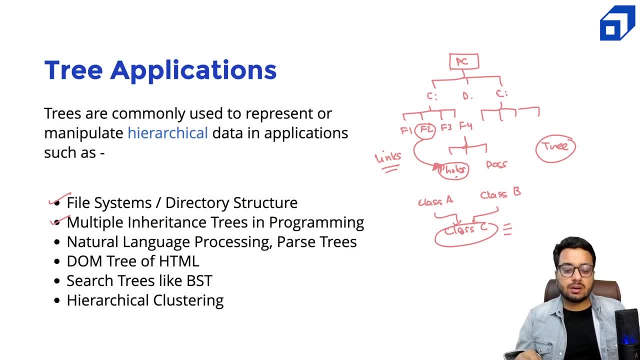 by the compilers to see what methods would be part of the class that you have implemented using inheritance. okay, Then again in natural language processing, basically whenever you have a sentence- for example, I am going for a party right Now- this sentence can be broken down into certain components. 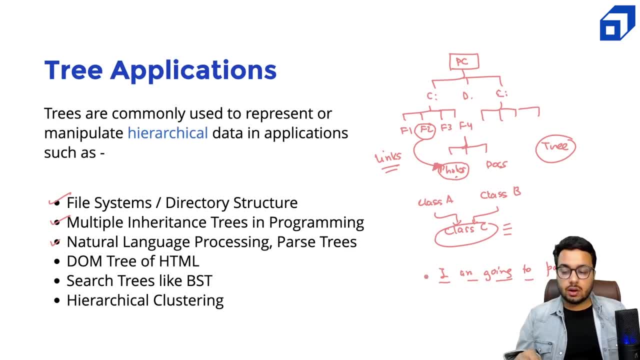 Maybe you have a verb, maybe you have a subject, maybe you have a predicate or you have even for language parsers, okay. So what are your parsers? Whenever you write code, it goes through a language parser so that compiler can figure out if there is any error in the 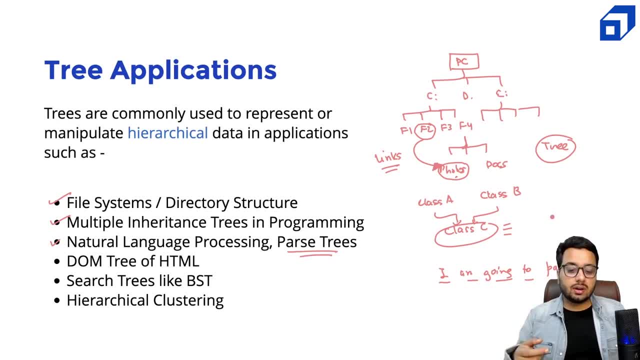 code, is it? it is having the correct syntax or not? So they are. So again, form a parse tree of that code, right? So again, it's an interesting concept that you will learn in compilers, right Again, they're used a lot in understanding of the. 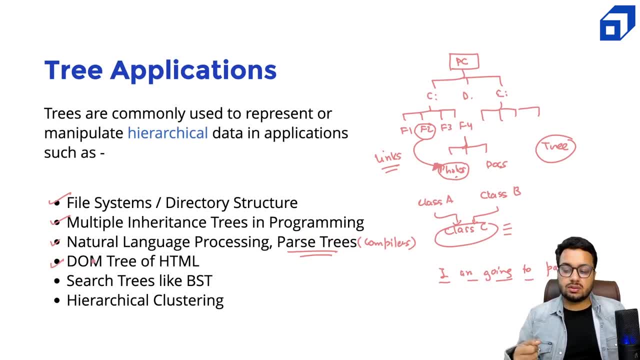 language. okay. Then in HTML there is a DOM tree. So whenever you open up a website, right, you see there is a HTML code. right Inside HTML code there are a lot of tags. there is head, there is body. right Inside body there is a paragraph, there is a div there. 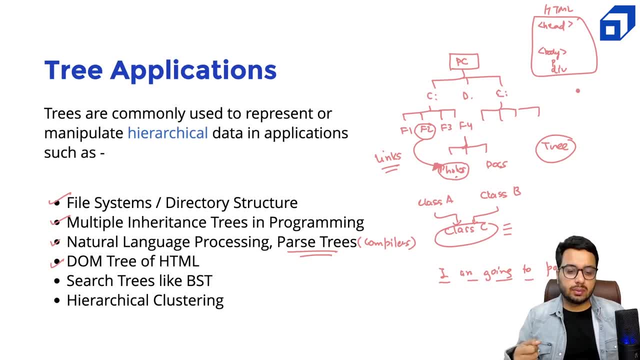 is an image, right. If you look carefully, this whole document forms a DOM tree. So inside DOM tree you have head, you have body right. Then you have certain elements, you have div, you have paragraph. here you might have image, you might have some text it. what is happening? 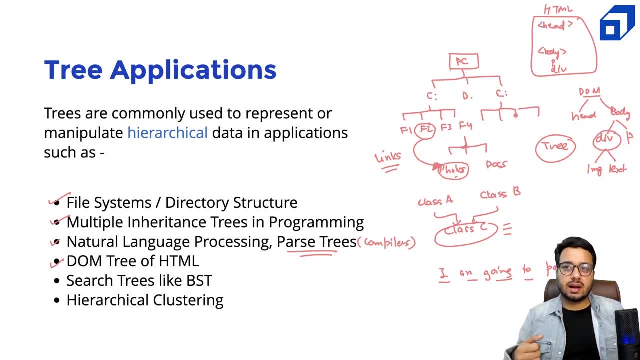 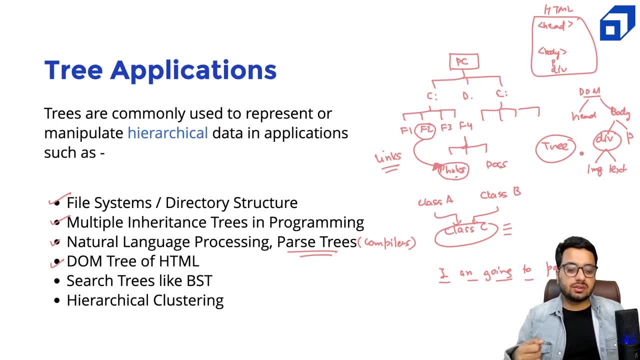 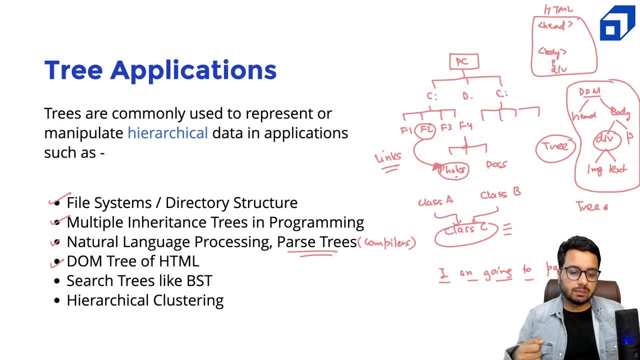 this DOM tree. it is a tree of objects. okay, It is a tree of objects in your web browser. Again, it's behind the scenes. it is doing some kind of search operation on this tree and it is trying to manipulate this tree Right, For example, you scroll your webpage. 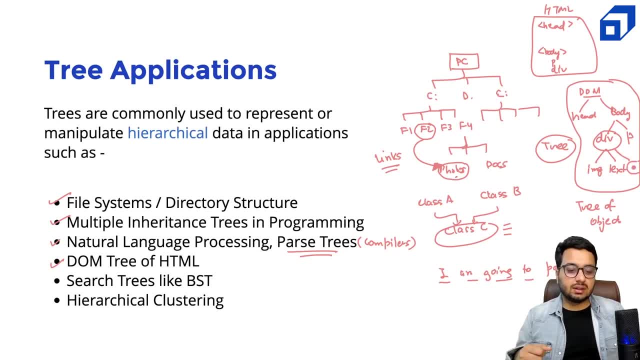 and a new item is added from the bottom. so maybe it is adding something in in the list, right? so your tree is getting modified, right then, of course, there are trees which are used in search operations, like binary search tree. there are trees which are used to implement data structure, like map. 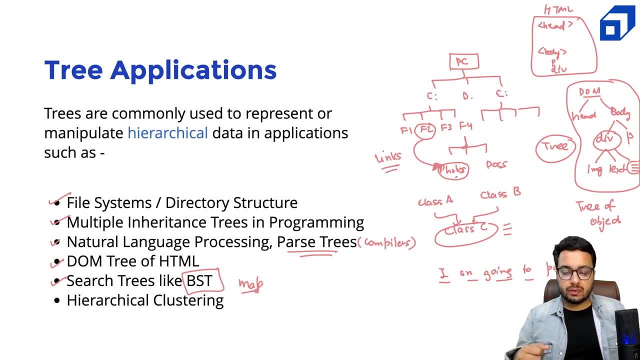 self-balancing trees. okay, so they are used to perform faster searches and keeping data ordered. we will talk about vsts in the coming class. in machine learning, there is a concept called as hierarchical clustering, so it is a part of a clustering technique. okay, where i want to group? 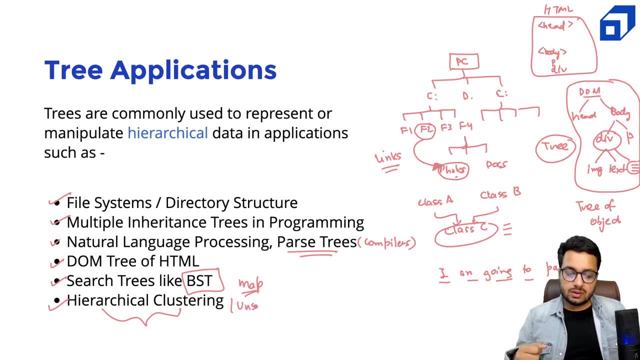 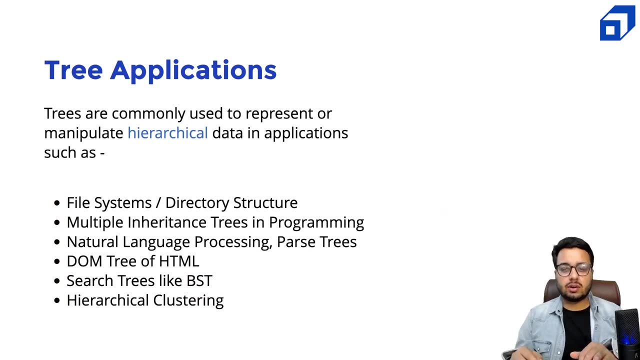 together similar items. so it comes under a part of unsupervised learning. so there also, the tree data sector is used, right. so you, we see lot of applications are there and that becomes very important for us to understand uh, the tree data sector. so in this video we will be uh talking. 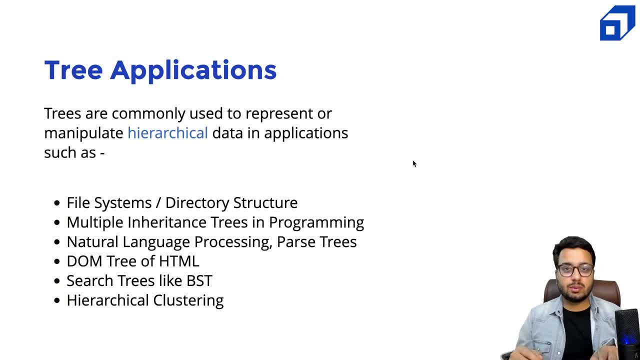 more about binary trees in general, because that they are the most common ones- uh, that are used in the machine learning. so we will talk about the tree data sector in this video. we will be talking more about binary trees in general because that they are the most common ones- uh that are. 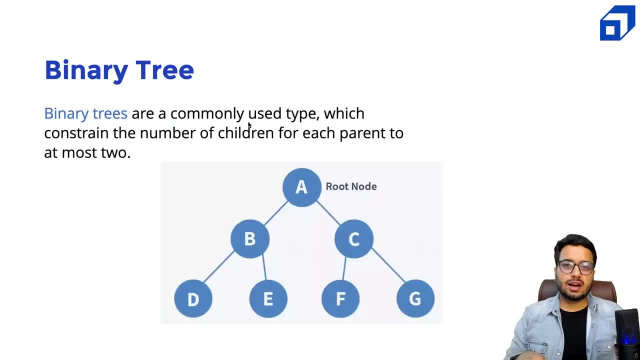 widely used. okay, so let us start with binary trees. so let us start by understanding what is a binary tree. so, as i discussed, it is the most commonly used uh tree structure, uh, in which you can have at max two children. okay, so it constrains the number of children for each parent to at most. 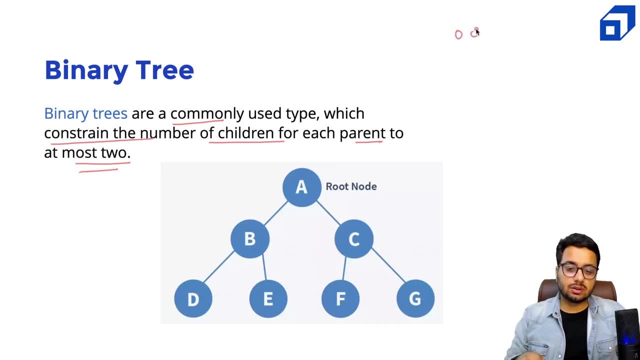 two. that means a node can have zero children. for example in this case the nodes d, e, f, g. they don't have any children. they are also called as leaf nodes, the nodes which don't have any children. they are called as leaf nodes. node can also have. 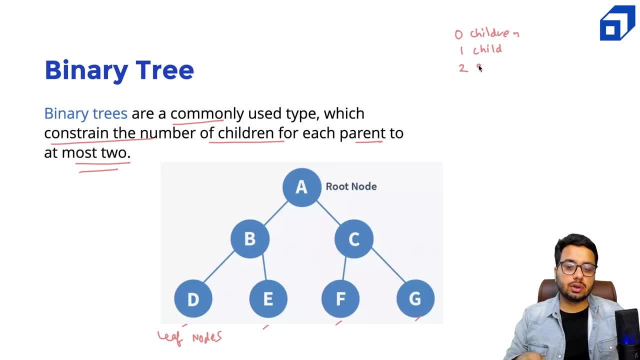 one child right. or it can have two children- right. it cannot have more than two children. for example, if i draw a few structures, you have to tell me whether it is a binary tree or not. is it a binary tree? the answer is yes. each node has zero child. one child or two children, right, okay, is this a binary? 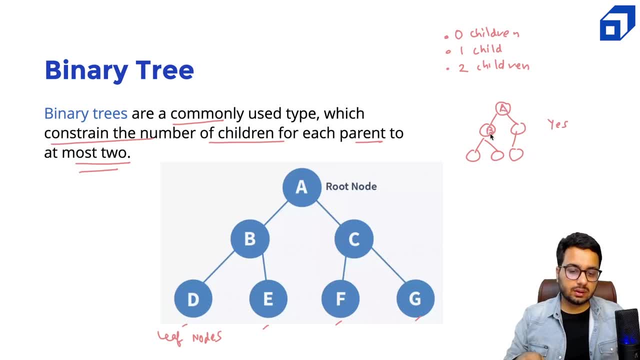 tree? the answer is yes. is it a binary tree? the answer is yes. is it a binary tree? the answer is yes. so this node, the node c, it has one child. a and b, they have two children. and d, e, f, they have, they don't have any children. hence, in this case, we have three leaf nodes. so this is again an example of a. 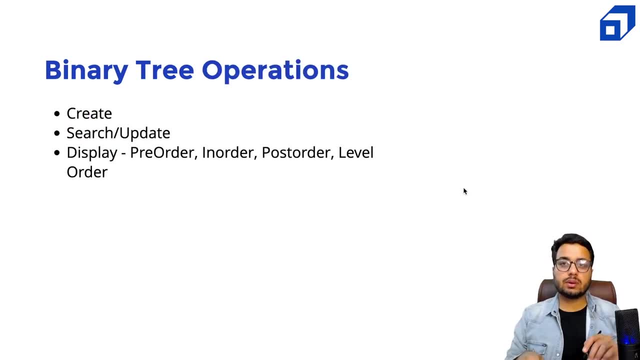 binary tree right now. what we are going to learn in this tutorial? we are going to learn about different operations. how do we create a binary tree? how does the node structure look like? how do we perform search or update operation on a binary tree? how do we display a binary tree? and there are. 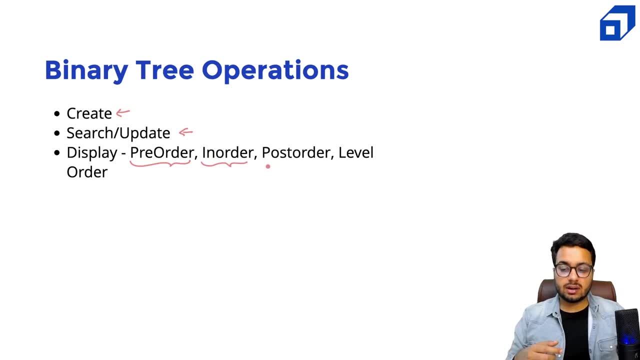 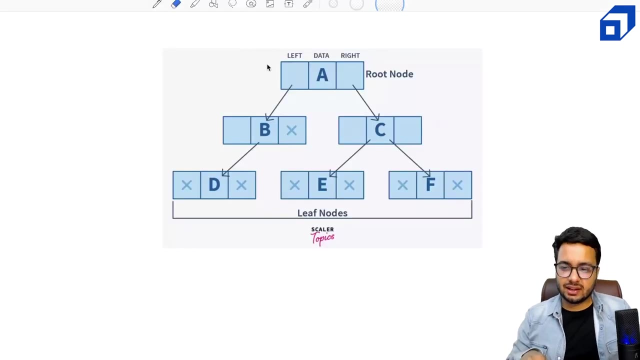 four popular ways to do it: pre-ordered reversal in order traversal, post-order traversal, level order traversal. okay, so we are going to look at all those, all these things, one by one, and we'll be starting with, uh, creation of tree. first, let's begin with that. let us talk about creating. 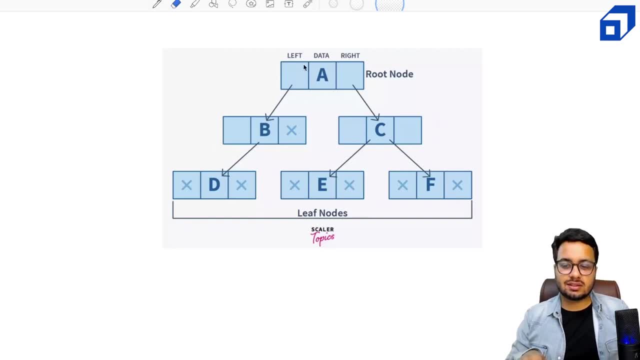 the tree. so first of all, we need to understand the structure of the node that is going to be considerate to create a tree. whatever you want to create a tree is going to create the tree right. so in this tree, if you look carefully, there are so many nodes. 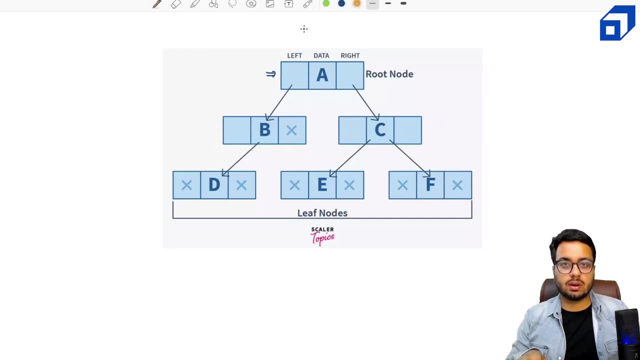 and this box represents one particular node. okay, that is the root node, right? so i have the root node. now, what is this root node going to contain, or any node going to contain? it is going to store three things. one is your data, one is the address of the left node, one is the address of the right. 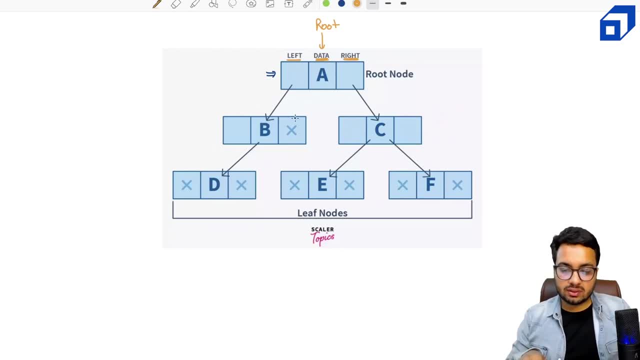 node. okay, in java we also call it as reference. right now. suppose this object b, it is created at some memory address, let's say 250, right, this is the location of b in the heap where it is created. so a is left- is going to store 250. let's say this is created at some location- 380, so a is. 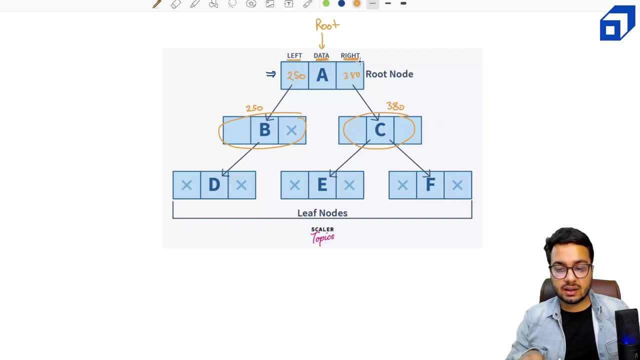 right is going to store 380. right, a itself is created at some some location, let's say 400, the root is going to store 400. okay, so root is not a node. root is just a reference to the root node. okay, so root variable is holding the address of. 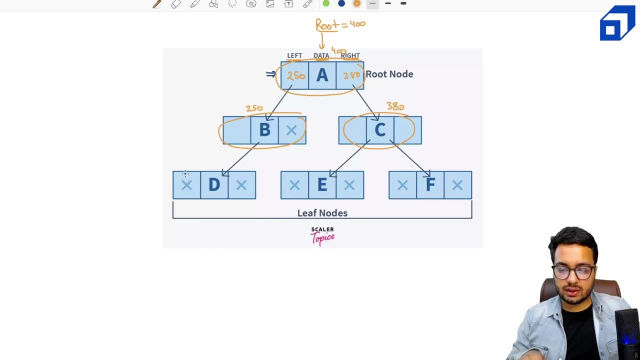 the root node right now. b is left, is referring to d, so d is created at some location, let's say 560. so here we will have 560. now d is left and right. they are, they are null. they don't refer to anyone because d is a leaf node right, so d is a leaf node. e is a leaf node. f is also a leaf node, so 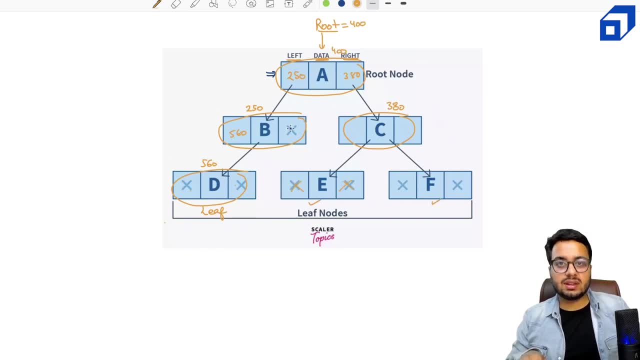 they are left and right, they are null. now, b is a node with a single child right, because it does not have any right child. hence this value is also null. and here i will store the address of e, here i will store the address of f, right. so i hope you are understanding the structure of the node. 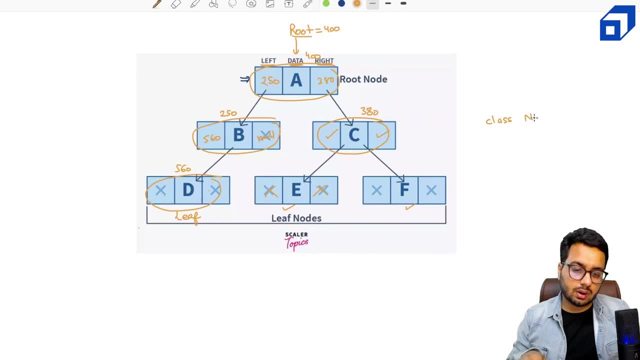 so i need to implement a class called node, in which i will have three things. one is my integer data. data can take any type. just to keep it simple, i'm taking it as a integer. one will be my node left- reference of the next left node- and node right. 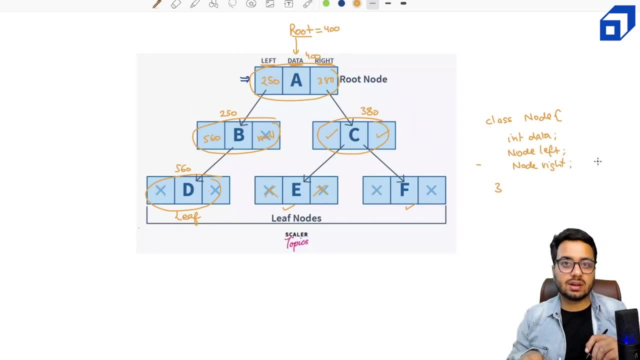 reference of the next left node and node right. reference of the next left node and node right reference to the right node. if the left and right node does not exist, then i will set this value to null. right now let us see in the code how can i implement this node class. let us go to intellij. 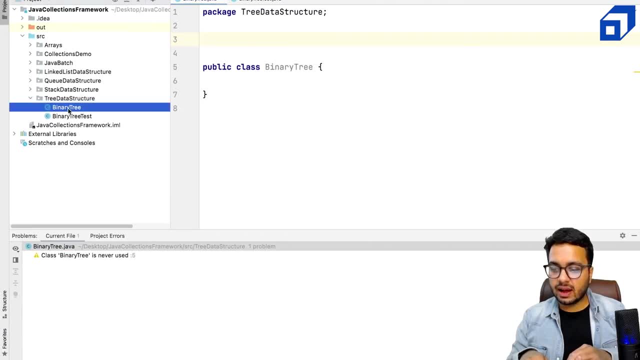 now i am going to implement the tree data structure. i have a class called binary tree. i have a class called binary tree test. both are empty classes as of now. in order to build binary tree class, i need to define that. what is node? right? so node will have three things. one is my data. 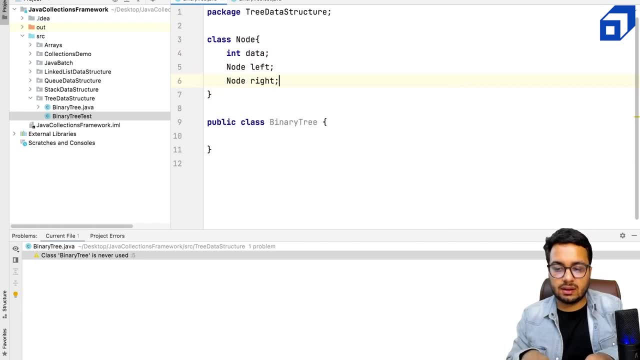 one is my left and one is my right. apart from it, i also need to give a constructor here that whenever a new node is constructed, what data it should take, that is okay, data i will know, but at the time of construction of new node i do not know what node will go into the left, what node? 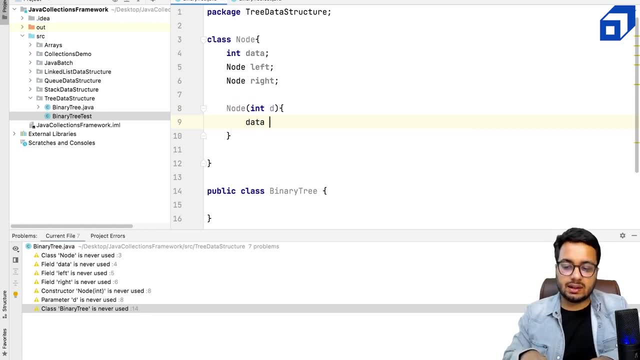 will go into the right. so i will simply say that my data this is equal to d and left and right. they will be set to null by default. so whenever you are creating a new node, you do not know the left and right node. you do not know the left and right node. you do not know the left and right. 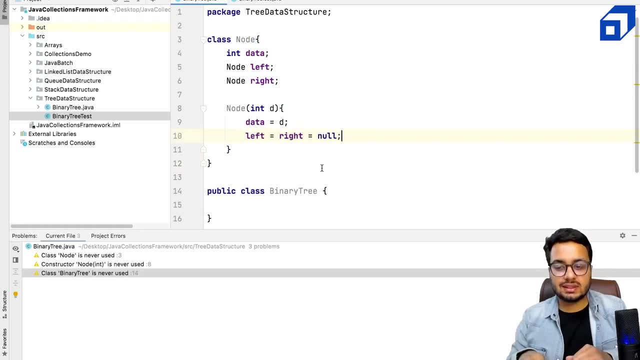 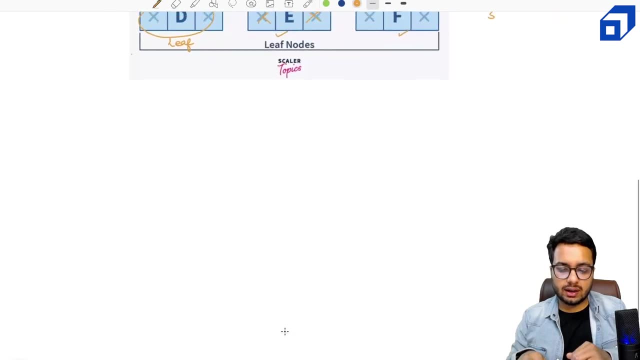 right nodes, so these will be set later. right now comes the binary tree class. now suppose we want to create a tree like this. okay, or let me take up another example in which I have numeric data. I can say: okay, let me create a tree like this, one connected with two, and then it is connected with. 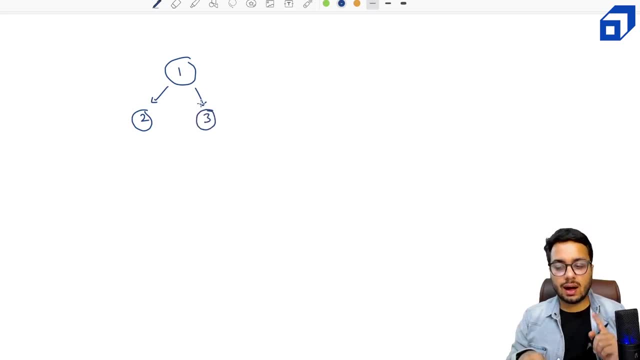 three, right, let's say very simple tree, three nodes. now how you will read this tree. the first thing is: how do I read this tree? right? so the first input I will get is the root node. okay, user will enter one. I will say: fine, input is one. let me read this: create a node called a root node and root node is: 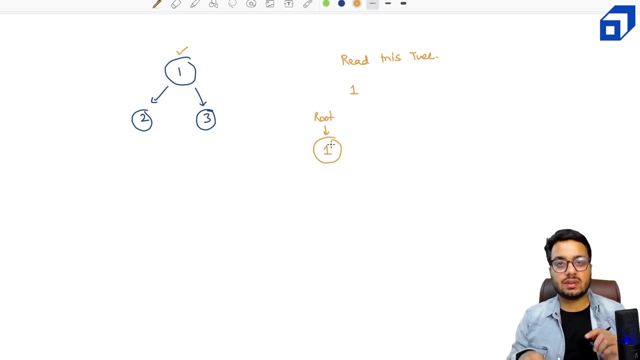 going to point to this node right and in the left of this. I will again read from the user right. the user says okay, fine, the next node is two. I'll say fine, I'll create a node called two. I will attach it in the left of one like this: okay, and now what is the next one? I 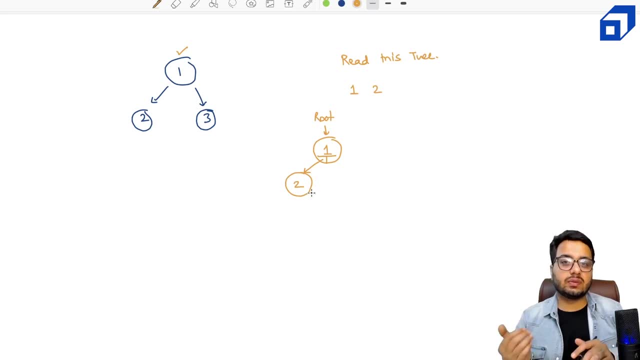 will read right now. it can happen that I have something in the left of two, or I have something in the right of two, or I have something in the right of one right, so I do not know. the way we are going to do it is. we are going to read now: what is there in the left of two. okay, so if the 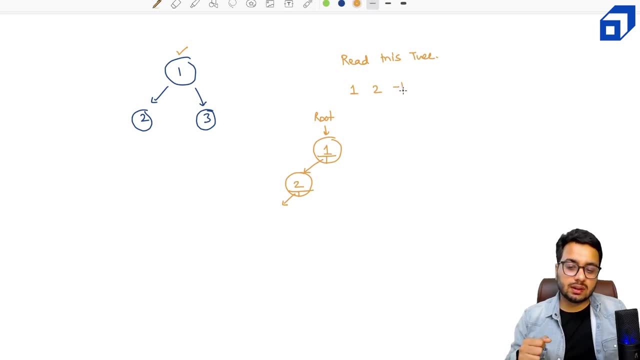 I will input minus one. so minus one in the input will denote that near is nothing here. so I will simply set this value to be null. right, what is right of two? I am again going to say it is minus one, so I will set this value to null right now. this option is gone. I have read it, this option. 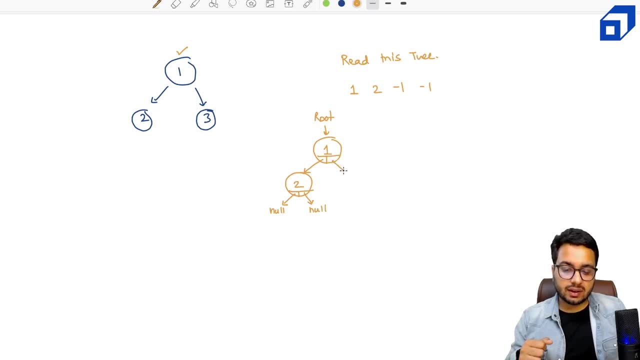 is gone now I can only read this, so I will come back here I will say: fine, this two is done. now try to read what is there in the right of one right. so it's okay. the next input is three. I will create a new node and I will attach it, of course, here, but before that I will read what is in. 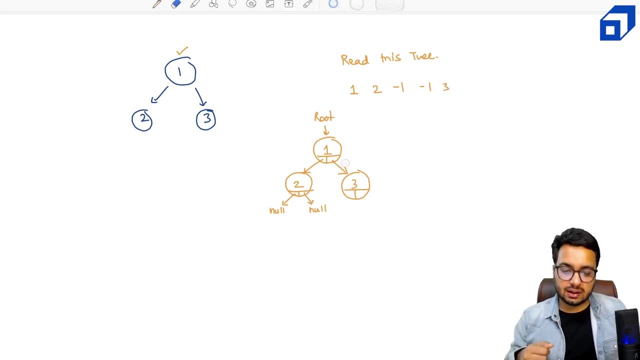 the left of three, right. so attach part will happen a little later right I'll read what is in the left of three. so this value would be minus one, minus one. what is there in the right of three? again I say minus one. now this node is constructed or in a way I can say this subtree has been constructed. 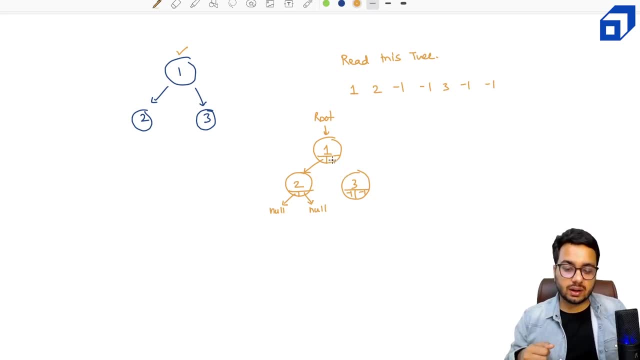 so once it is constructed I will return it back to the parent. so the parent is one, it will get connected here, right? so this will become more clear once I write the code. so idea is, I will of course do it for a bigger tree as well. this is little tricky, right? so the idea is: 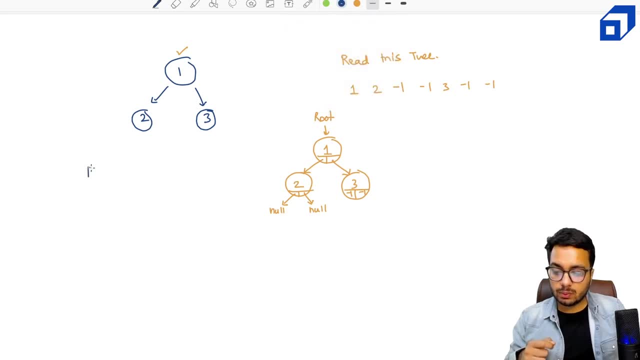 we are going to build a tree recursively. we are going to build recursively right now, how we are going to build a tree recursively, many tree operations. they are recursive in nature, right, so it's okay. fine, I will build the root node, that is one. then I will build the complete left subtree. 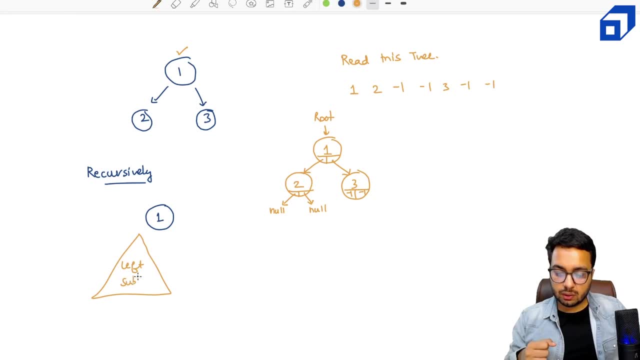 in the above example, the left subtree has only one node, so it looks easy. right, I will build the complete right subtree, right, okay, I will build the complete left subtree and I will attach it here. that is part one. I will build the complete right subtree and then I will attach it in the right of. 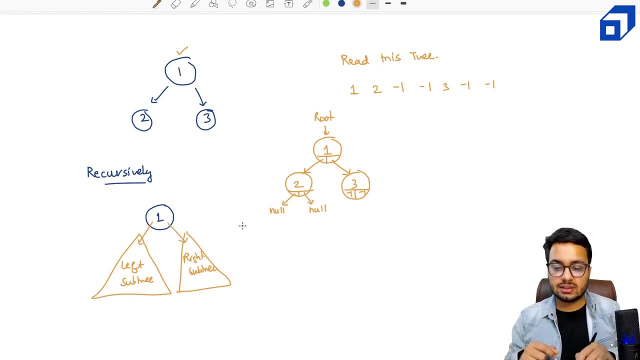 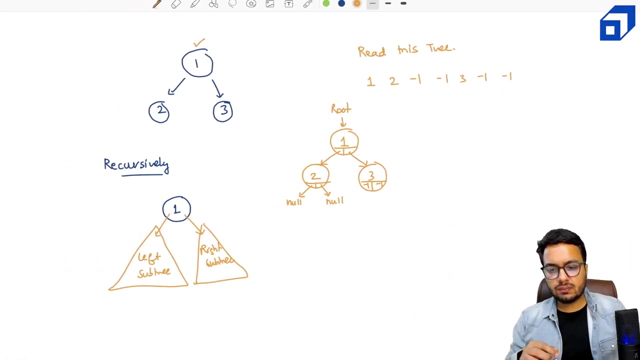 one right, so we will do it for a bigger tree as well. so let us jump into the code first and try to see how this can be written. of course, I will do a dryer and explain you how you can build a more complicated tree like this with the same code. okay, let us go into the binary tree. 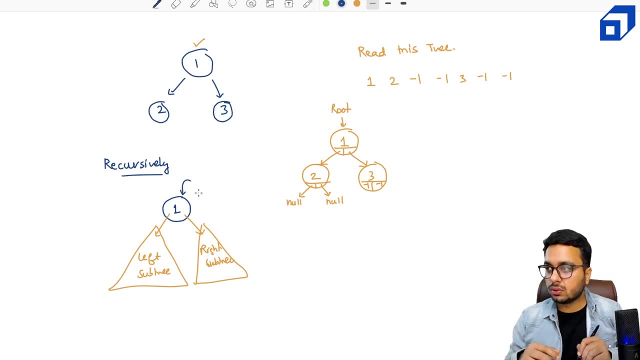 class. one thing is for sure: that every tree must know what is the root node. what is the root node. so this is something that will be the property of the tree. every tree must know what is the root node, just like in a linkless. every linkless knows what is the head of the link is what is the tail. 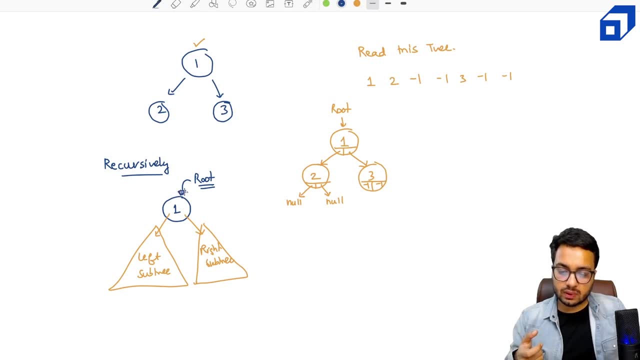 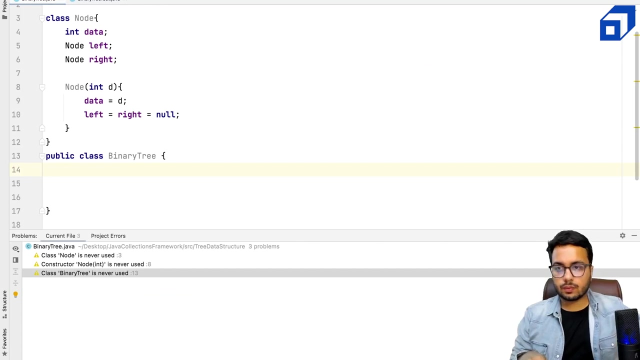 of the link list. so in in case of three, you must know that what is the root node, right? so one thing is there. I am going to read this tree. so user will, uh, input will come through the user, right? so let us see the tree construction part. so in this binary tree class, what I'm going 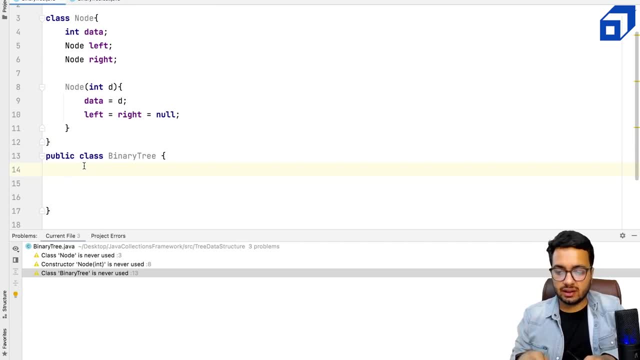 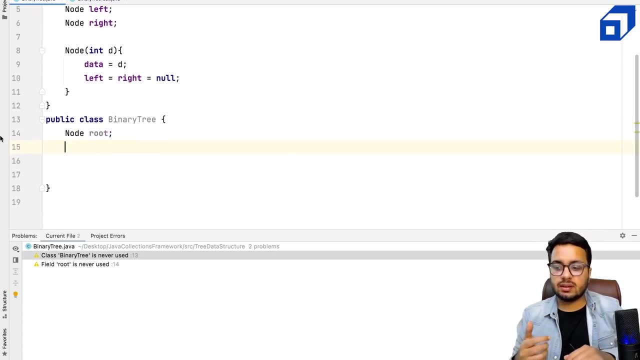 to do? I'm going to first define the data members of the tree. so I have only one data member. that is the root of the tree. right now, this root should be initialized where it should be initialized, of course, when the tree is created. so when the tree is created, it is created. 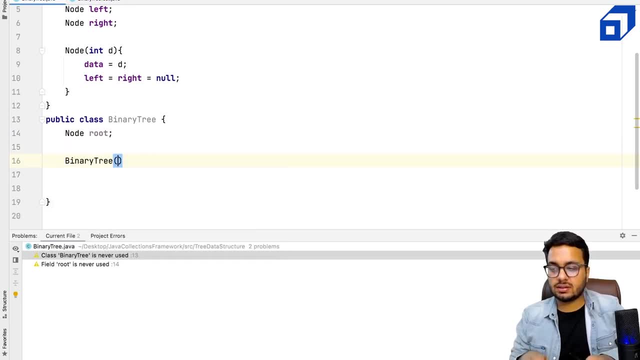 then the constructor is called. I need to define a constructor called binary tree. right now, in this constructor, what I need to do? I need to take input from the user. so in order to take input, I will need a scanner object. I will say scanner SE. this is equal to new scanner system dot in, so scanner. 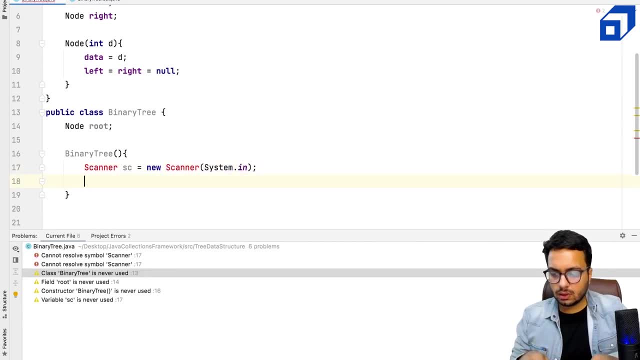 object is used in Java to read inputs. so I have imported the scanner right now. the building of the tree is recursive in nature, so I will create a helper function to do it. so I can define node, let's say create tree, and to this create tree method. I am going to supply the scanner. 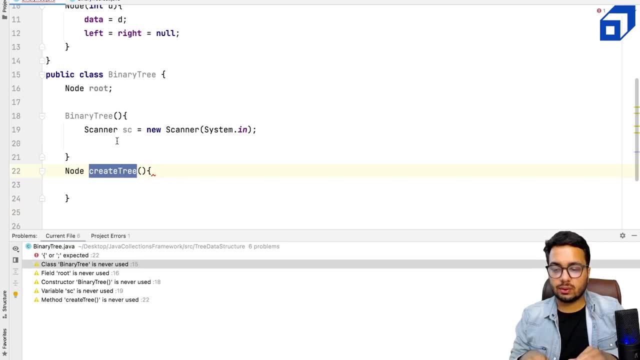 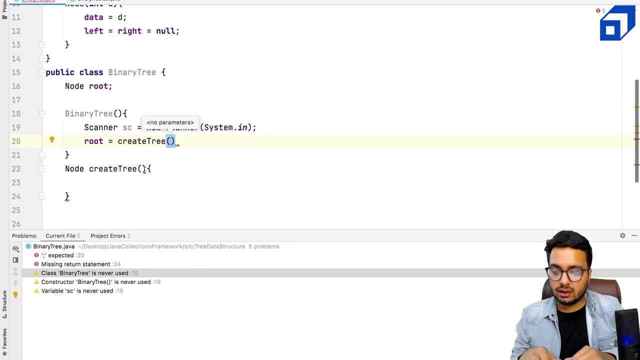 object so that this method will actually read from the user. okay, so I will define. the root should be initialized by calling the create tree method. so create tree is a helper method getting called in the constructor that will read the tree from the command line. right now I am going to pass the scanner object here so that I can use it to read. 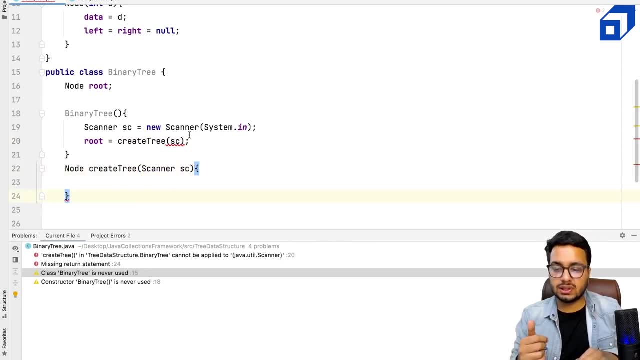 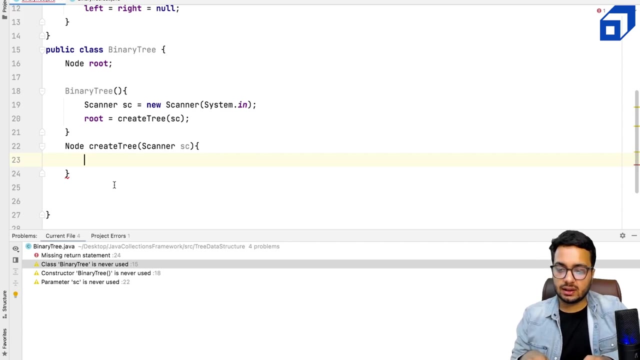 data from the user. right, I don't want to create this object again and again. uh, inside this method. okay, so I am creating it once and that object is being circulated across all the recursive function calls that are going to happen right now. suppose I read something I can say: okay, uh, data that I'm 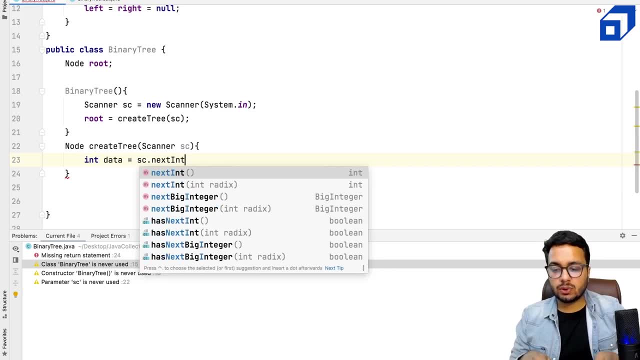 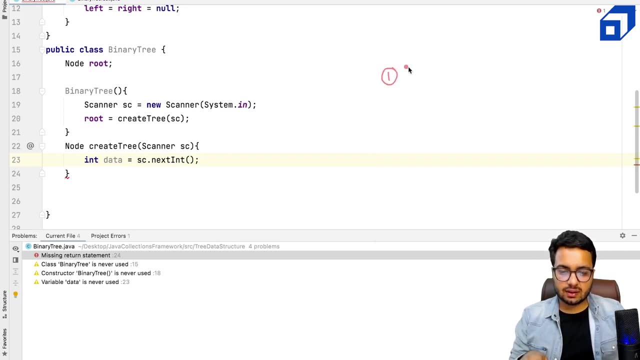 going to read is scanner dot next tent. so I'm going to read something. all right. now I have read something from the user. let's say this data is one right, what I want to do. okay, this data can also be minus one, right. I'm asking: okay, tell. 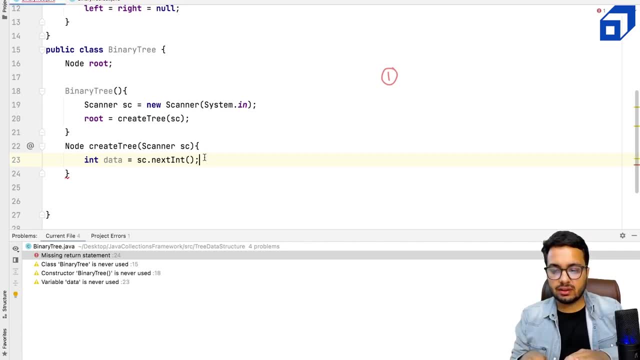 me what is the next data. so I will actually have a two, two types of case. one will be my base case. if my data is minus one, then what should I return? I will return a null. that means okay, I don't want to attach any node here. 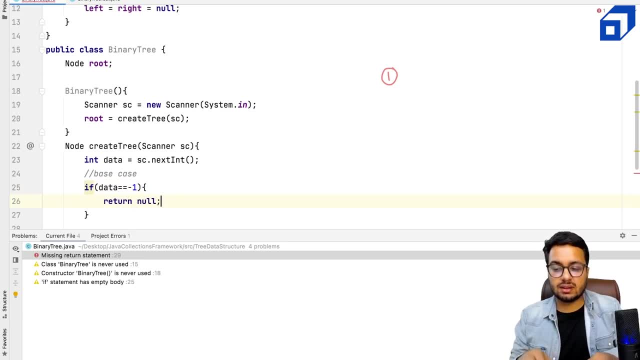 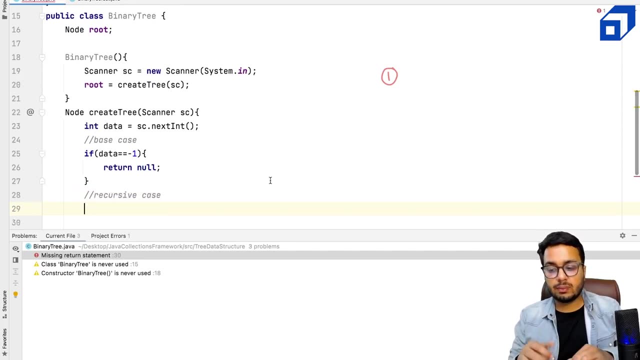 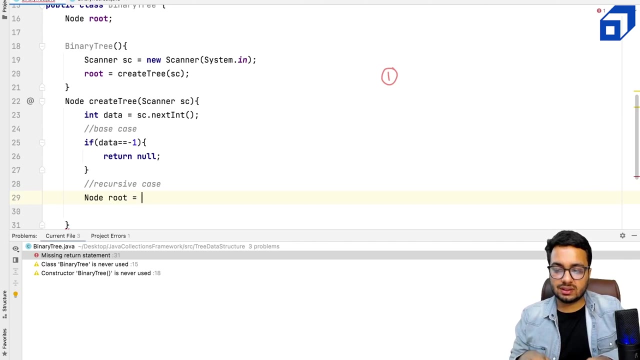 that sub trace just null. I will return null, but if it is not minus one, if it is something else, basically I'm talking about the recursive case. for example, if my input is one, what I will do? I will create a new node, I'll define, I'll call node root. this is equal to new node. 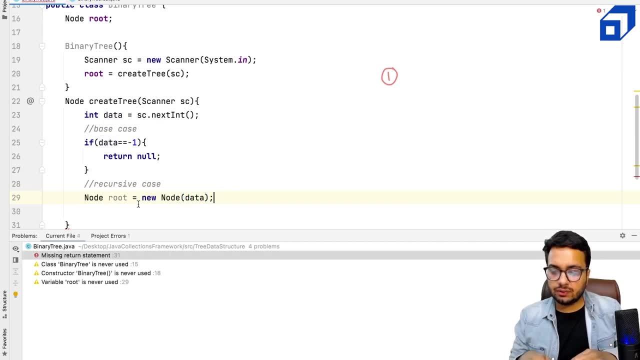 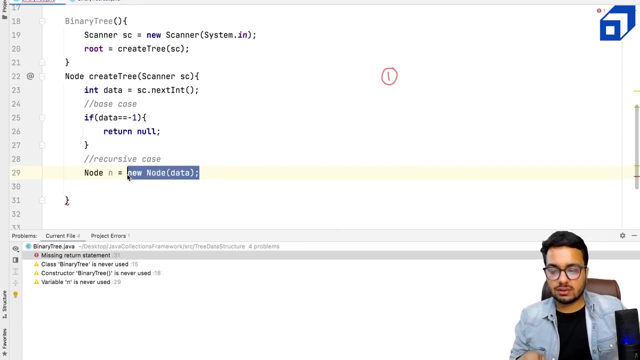 and I give it the value data, right? if root is confusing to you, just call it as n. right, I create a node called n, initialized with this data. so suppose my input is one, right? so I say, okay, n is a new node. now what should I do? I need to read the left subtree. basically, I need to create a left subtree. 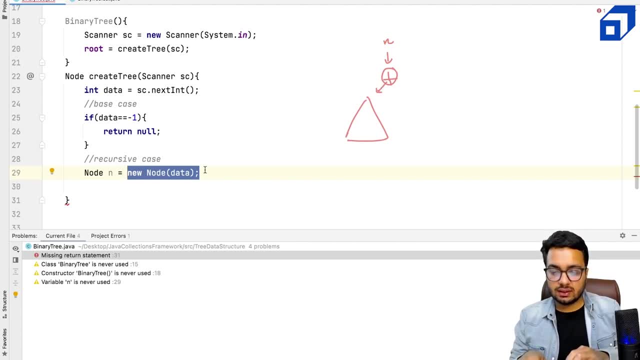 here and attach it here right. what I can say? that in the left of n, n dot left should refer to a new tree which is equal to create tree. again, scanner will get passed. what should n dot right point to? n dot right should also refer to a new tree called create. that is returned by the create tree. 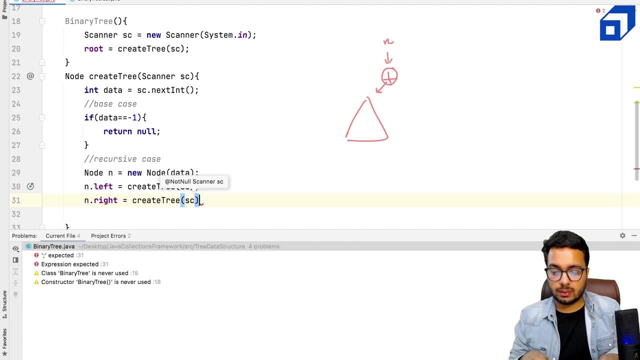 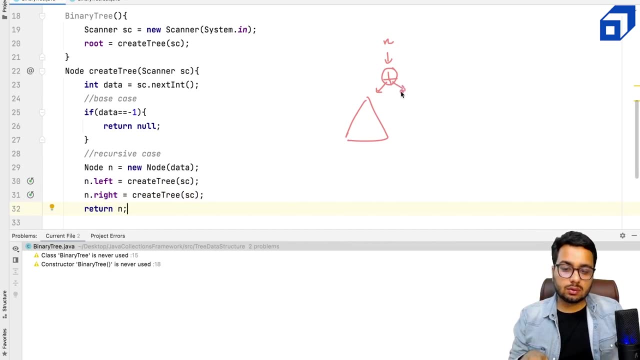 method and again, the scanner is going to get passed and then I can return n what I'm saying, that n dot right should also point to a new tree: left, subtree right, subtree right. this is the recursive way of constructing the tree. now you might ask: okay, how does this method will actually. 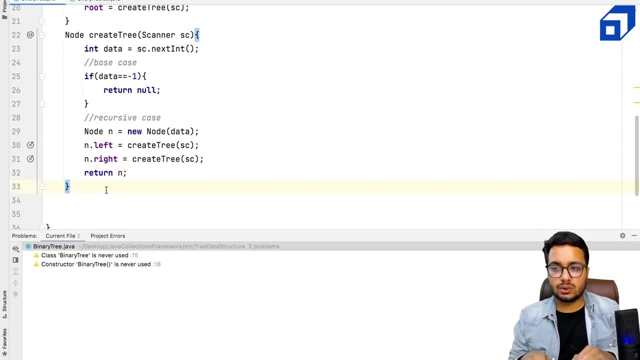 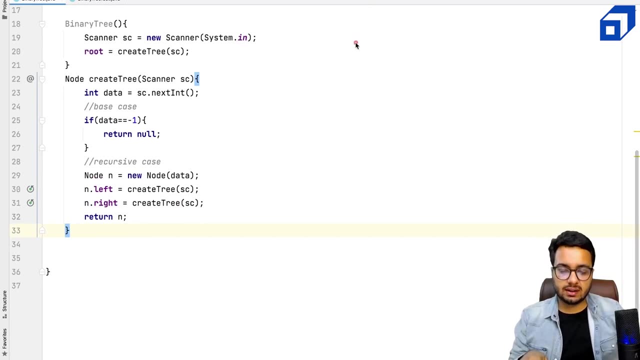 work. I will show you it will actually work. let's see how it's going to work, right? so let us take an example of a more complicated tree. or let's first start with a simple tree, right? let's say, I have a tree like this- one, two, three, right for this tree, what is my input going to look like? so input will: 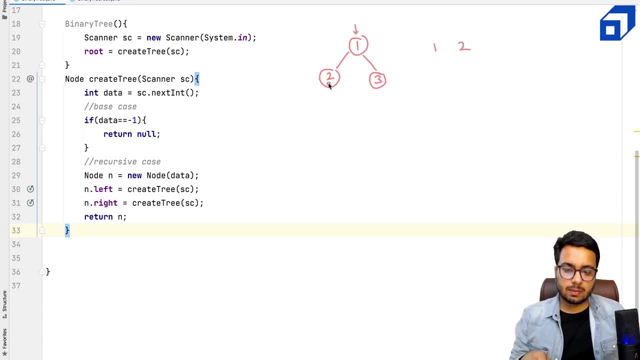 be one, then it will be two, then it will be left and right of two, which is minus one minus one, then it will be three and left and right of three, which will be minus one minus. so, given this input, I actually want to create this kind of a structure. let's see how it's going to happen. 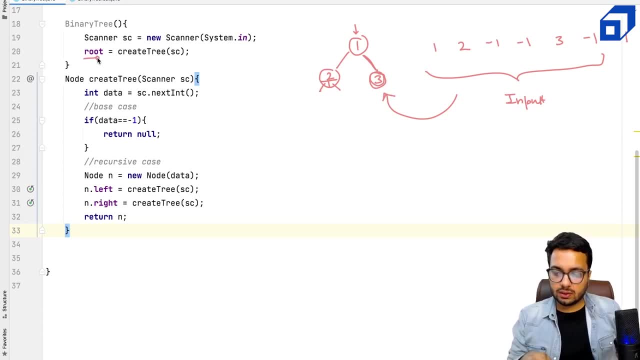 is it fine? uh, root is equal to create tree. I call this method create tree. it read something from the user, so 1 integer it's going to read. so it's going to read one. so data is not minus one. I come here node and this is equal to new node. so basically I have a node and this is equal to new node. so basically I have a string. so for continuous implementation I want as user these structures and predict area. it is going to one, so data is not minus one. fine, I come here. node, and this is equal to new node. basically I have a 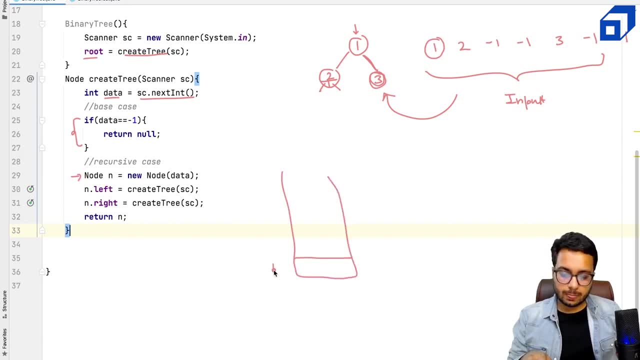 still requesting bot remove, move, because we have a staircase between the yawn's. and then come here, a crack there and come here. that's going to cause some 듣 Mang in the editor rather to use. or basically, I have a stack call in which n is going to say: n is a new node where the data 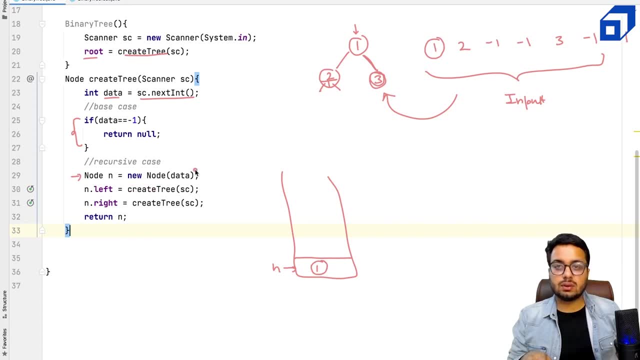 is one. fine. now n dot left. it makes a new call: n dot left, right. so I said fine, in the left of one I want to create tree. so again, create tree is called. if you come again in this function, you read something from the user. so you read two. fine, you said fine, I. 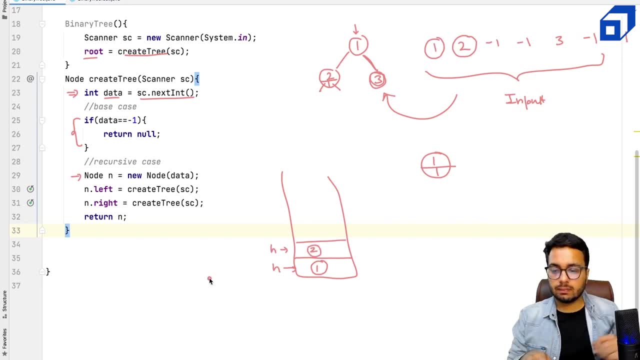 create a new node n. okay, a new node n is created. so earlier n was here. now the new n is here. right, it's a local variable. it is created in every stack call. right, it is here. this is equal to new node where the data is two fine n dot left. this is equal to create tree. 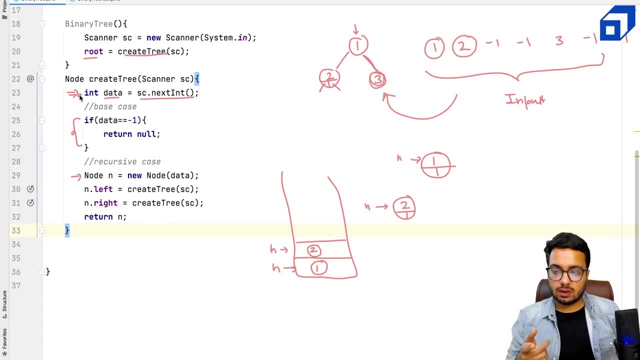 right. so again I call, I make a function, call create tree, go and do something- right. so I've made a call for here. right now, if I go and read what is the next number, it is minus one. so I return null. basically what happens? so twos left made a call and it got a value that is null. so twos left starts. 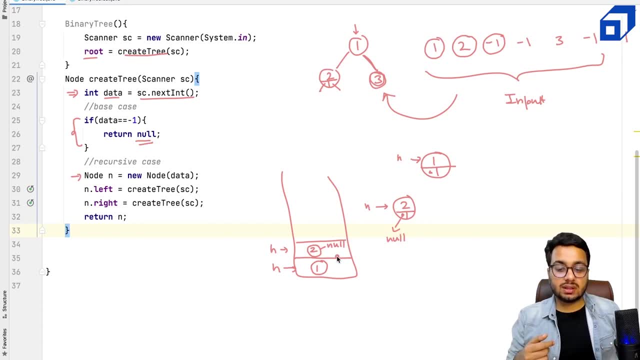 pointing to null. now what is the next call that is going to happen? we are in this stack and I make a call that twos right. this is equal to create tree. so I make another call here and this value is also null, right. once these two calls are over- this one and this one- I 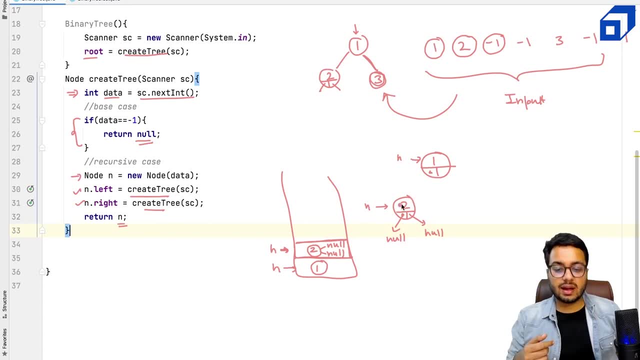 return n. so I return this n back where I return it to the place from where it was called. so who called it- one called it one- gets to know that my left should refer to this node. so by returning this n, this answer goes back to the previous function and once left is. 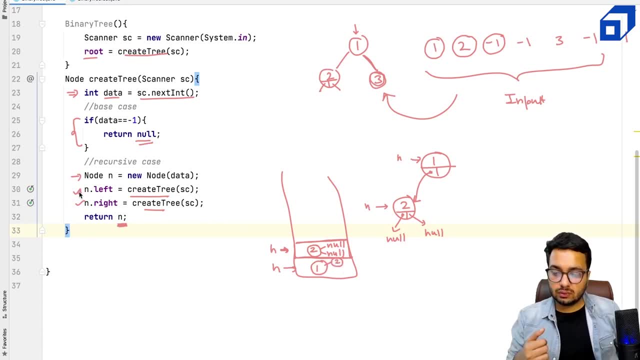 now connected with. now what is the next call we are going to make? so once left is now created. so this call is over. once left is now created, right now. once is okay. fine, my left is created. I'm pointing to two. I will make a call to update my right. so n dot right. this is equal to create a tree. 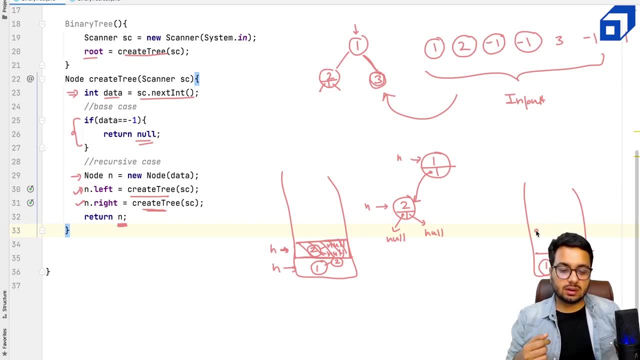 right, so this was already read again. a new function call is made. you read the next number, that is three. you create a new node from line number 29. you said the new node is three n dot left. this is equal to create a tree. so three is left. makes a call to the next number. 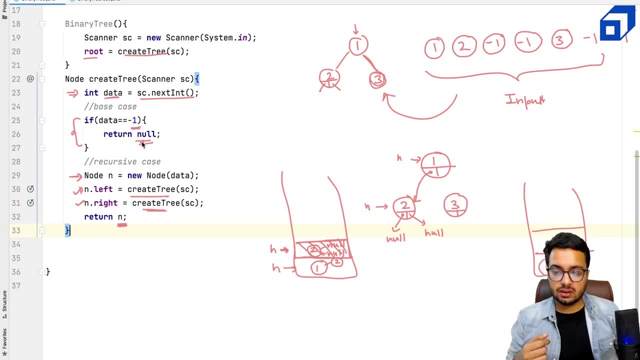 create tree, which again reads the data that is minus one. so you return a null. so three is left says okay, make a call. that call says i will return null. now three is right. says make a call to create tree. it goes and reads the number that is minus one. again it returns a null right. and then you 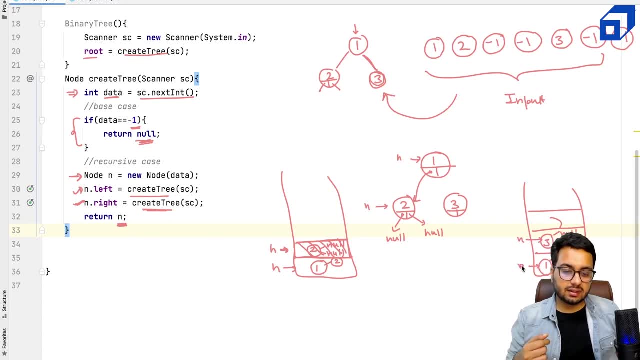 return n. so now n is this right? so it returns three back. when you return three back, what happens? who called three? so one's right made a call to create this tree, so one's right is now going to store the address of three, so it gets connected here from here. if you return n, where does it go? 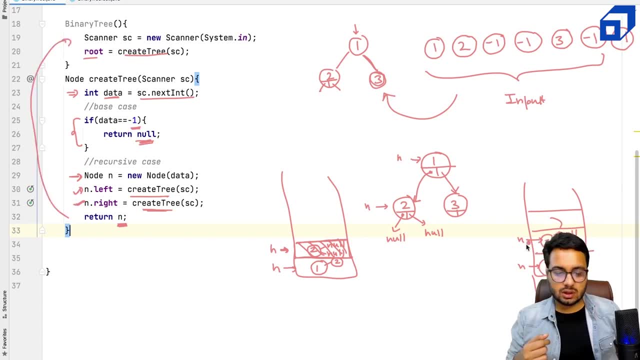 it goes back to the constructor, because this made a call to create t. finally, root is referring to the address of one, right? okay, i will hide myself so that you can see. the root is referring to the address of one right now. so i will hide myself so that you can see. 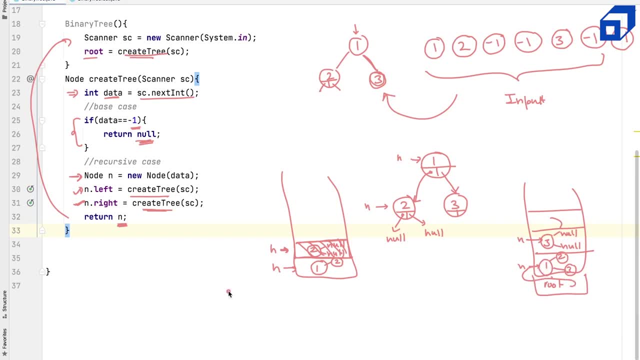 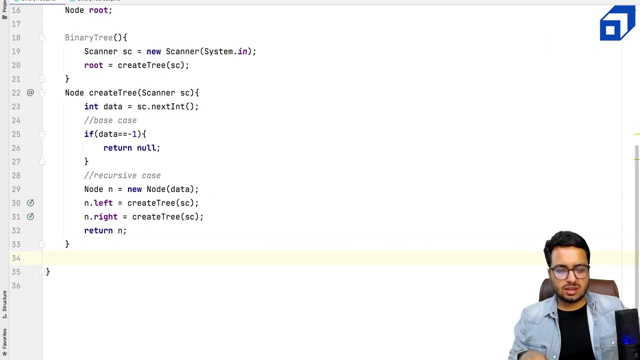 string to this one, right? so this is how it is happening, right? so this is a small example demonstrating how this small tree is constructed using this code. right now, i will run this example on a. run this code on a bigger example as well. now, some of you might not be convinced that whether 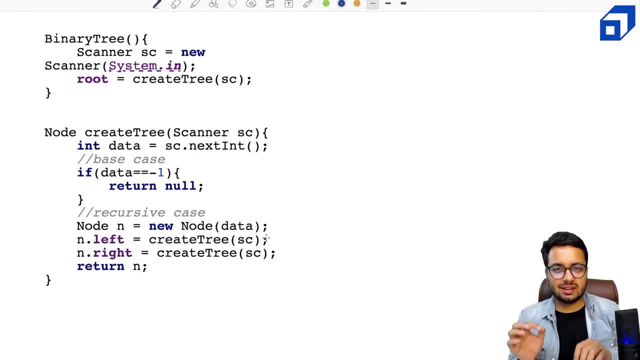 this code will work for a bigger tree or not, so let us rerun this code on a bigger example. okay, so this is the method: create tree. that again i am explaining with a big, big example. let's say i have a tree which is, which should be built like this. let's say i have one, i have two, i have three. 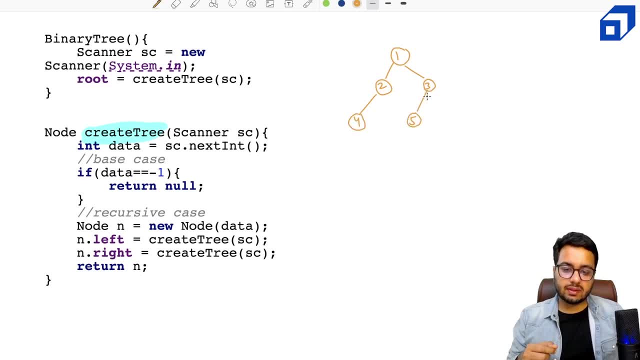 i have four, i have five and maybe i have six. now what input should i give? so, first of all, i will give the root node. okay, so input will be one. then i will give the root mode. okay, so input will be one and i will give the root node, okay. 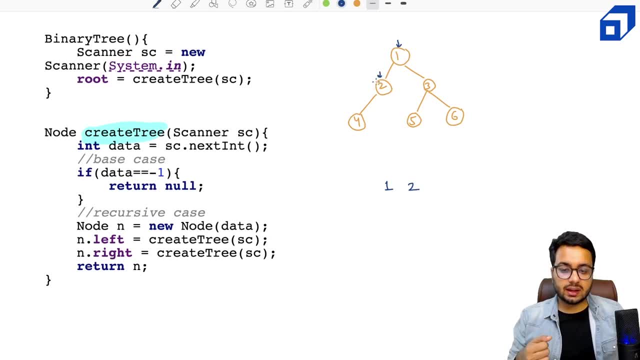 will go left, input will be 2. then again i will go left, input will be 4. then i will go left of 4, which is minus 1. i will go right of 4, which is also minus 1. okay, then i will come back. 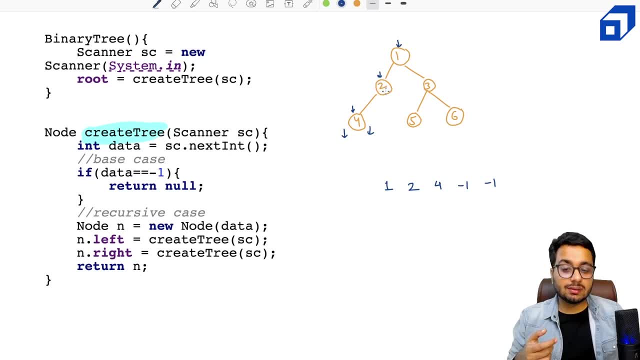 because 4 is done, i will come back. i will go in the right of 2, so right of 2 is again minus 1. then i i will go back. 2's left is done, 2's right is done. right, i'll go in the. 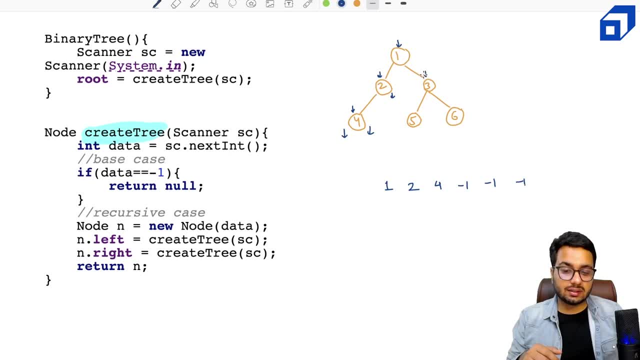 right of 1. so right of 1 is 3. then i will go in the left of 3, which is 5. i will go in the left of 5, which is minus 1, right of 5, which is also minus 1. then i will go back. i will go in the. 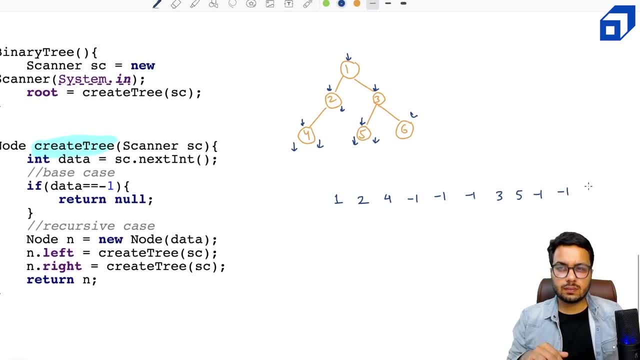 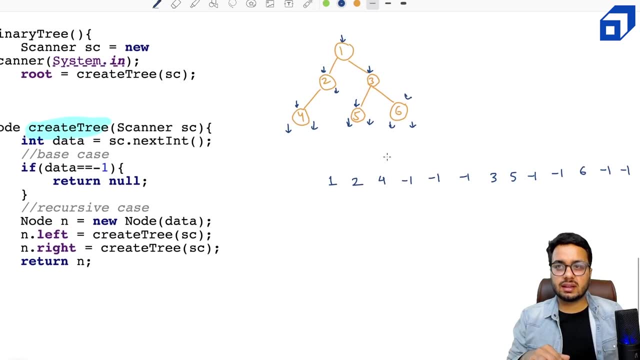 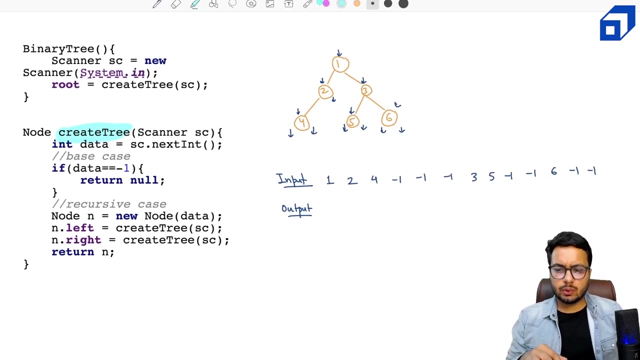 right of 3, which is 6, then left of 6, right of 6 minus 1 minus 1 right. so the goal is: given this input, i want to create this tree structure in the output from this input. i want to create this tree structure right now. let us see how we are going to do it. so, again, i'm going to read some. 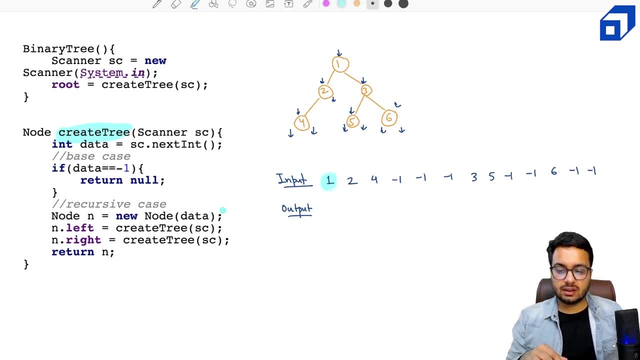 data. so i will read the first number, that is 1. i will say: find data is equal to scanner dot next to it. so i will read the first number, that is 1. i will say: find data is equal to extent. it's not minus 1. so i create a new node. n right, so fine, let's create a new node. 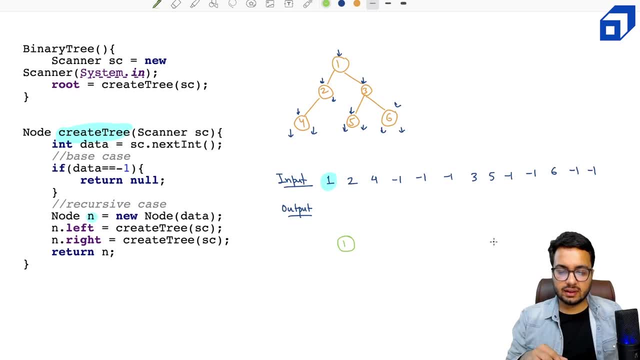 n, that is having data 1. let me draw the stack as well, side by side. so n is referring here right now. what so, if you want to learn key, what is the function that is currently executing? so that is at the top of the stack. so n is created. now you make a call. n dot left equal to create tree. so 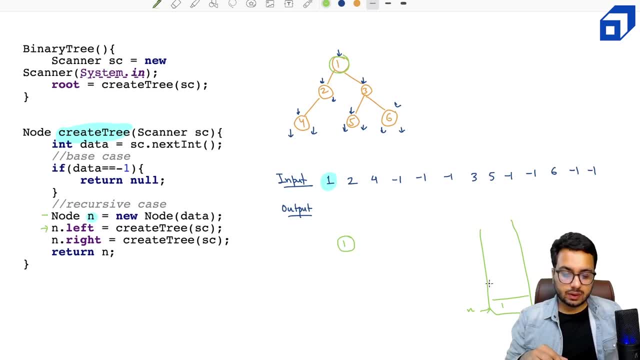 you are making a call to create tree. so you are making a call to create tree. so you are making a something in the left of one right, so one makes a call for the left part. so again you go call this function. you read data. so data is the next number, that is two. fine, you again create a new node. now 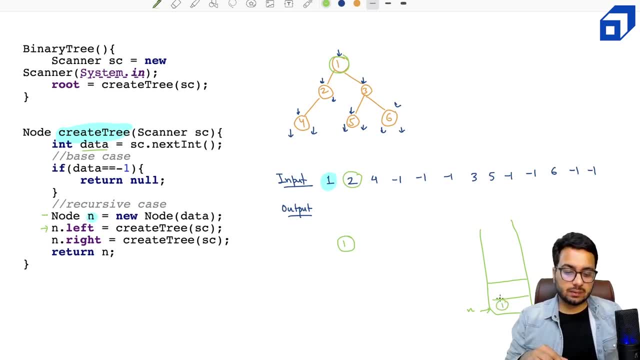 this function is paused. this function is paused. here you said: fine, i'm going to create a new node and that node is two. that node is two right now it is not connected. it's not connected with one right. and again you say: i want to connect something in the left of two. 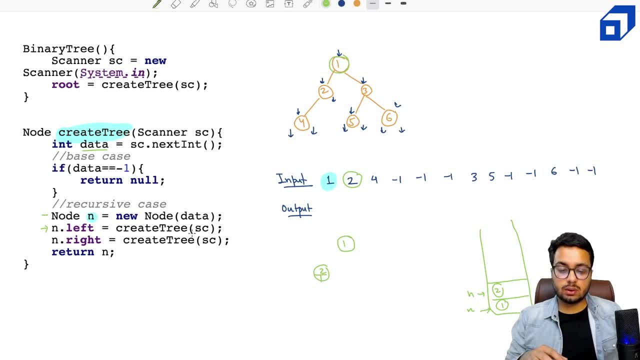 what will be that something? again you make a function call to create tree. so again this is paused and it is expecting to build its left tree. so you again call the function create tree. you read the data. so now you are going to read four. so you read four. you read four. now four says okay. 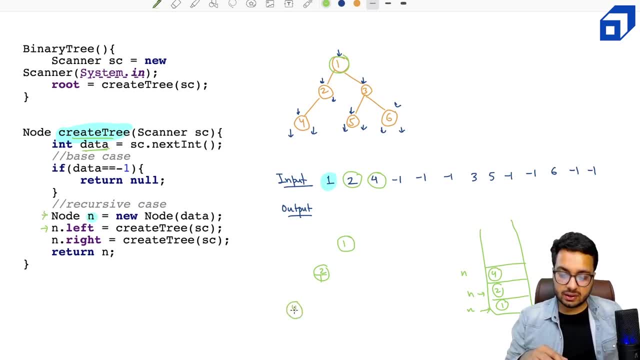 i am. i am a new node and i will create something in my left. a force left makes a call to create tree. the force left again makes a call to create tree. so now you are going to create a new node and in this case you read data. the data comes out to be minus one, and if the data is minus one, you 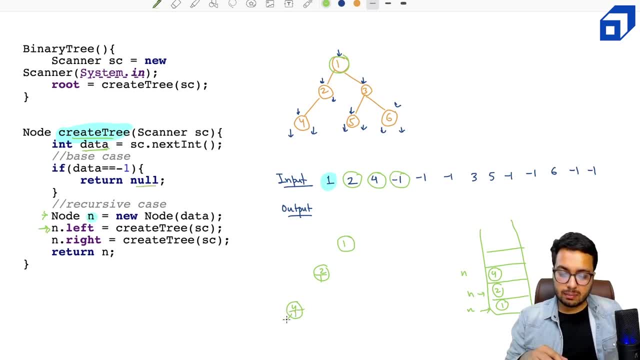 return null. the force left gets to know that my value is null. so a null is returned from this function which is attached with left of four. and then you hit this line for the first time in this function: call right, end dot right. this is equal to create tree. now you say, okay, i will again. 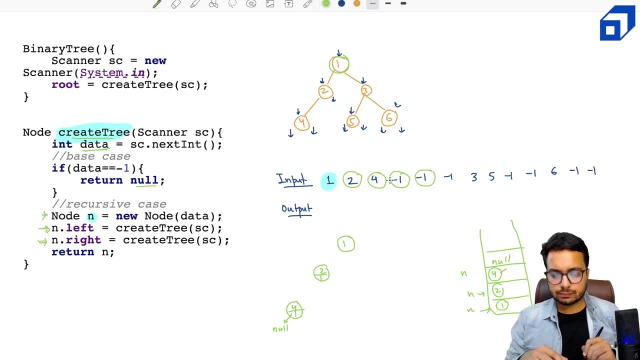 call create tree. i will read this line for the first time and then you hit this line for the second time. this number, this number, is again minus one. it returns a null in the right. also force. left and right they are null. that means the subtree of four has been created. this subtree is finished. 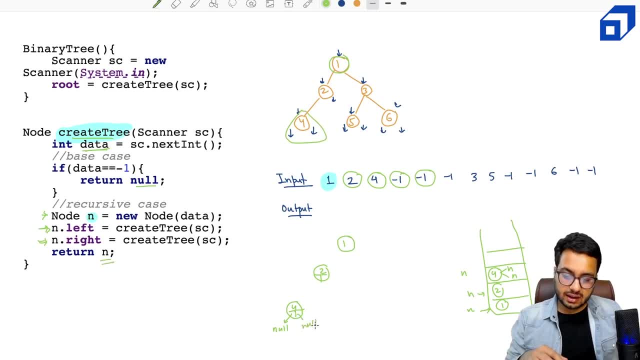 i will return n. this is null and i will return n. n. is this aware? this return value will go. it will go back to the place from where it was called. so who called it? two is left called it. so two is left is now connected with four, and this function will return to the place from where it was called. so 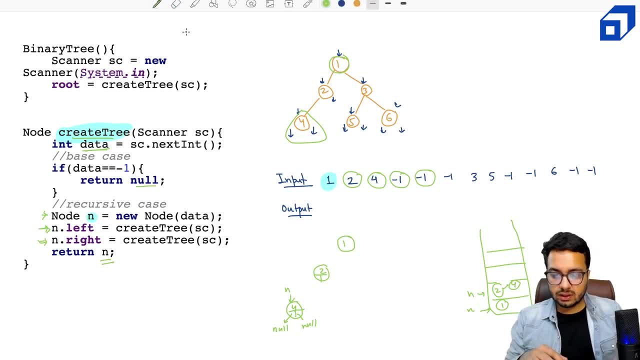 call is over. right, so two is left is connected with four. right now, this is the point where this connection has been established. right, so two made a call to four. four said: okay, i will build myself. i will build my left and right, which are null, and now i will return myself. right so two's left is. 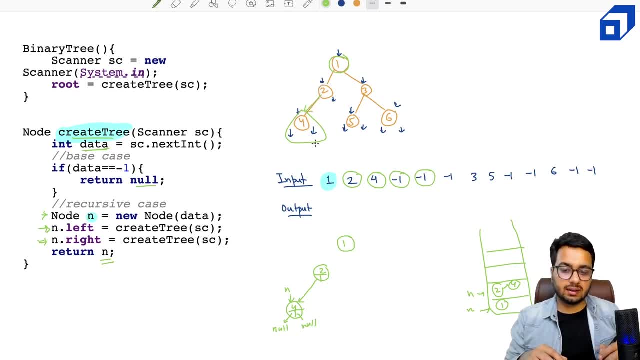 over. now what will happen? two will make a call on the right: the right subtree. so two makes a call here: n dot right. this is equal to create tree. now what will happen? two will make a call on the right. what do i read next? again, it is minus one, so i return a null. i return a null from here. so two's. 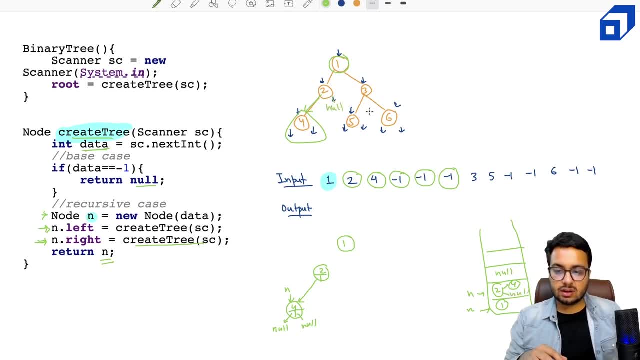 right is null, the two's right is null. it's not referring to anything, right? so this value is null. now two's left is done, two's right is done. i read. i say return n. so return n means what is the function that is at the top? at the top, i have this function. i'm going to return this subtree. 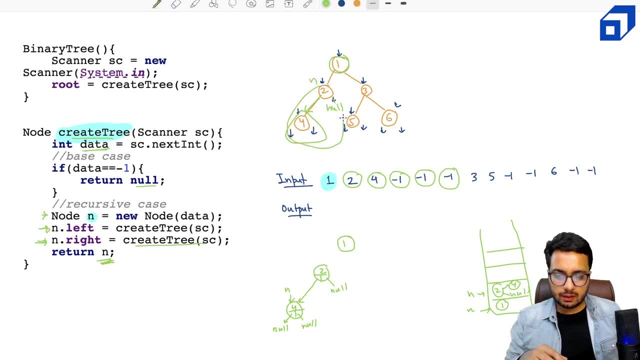 this whole subtree back to one. so basically one will get to know that my left points to this end and hence the left subtree of one has been built. now i will build the right subtree, right, okay. so one will say, okay, fine, my left subtree has been built. this is over from the call stack. so once one is now 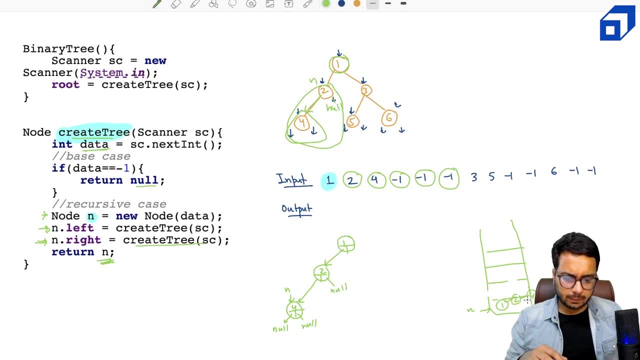 connected with two and four. right this tree, a one will say: okay, now it is my turn to call the right. so once left is done, it will execute this line: n dot right. this is equal to create tree. now you again make a call. next number you read is three. so you create a new node called n. 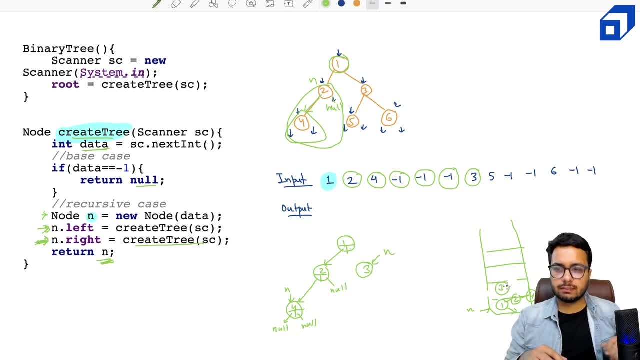 this is the new node. so three is created. and then you again make a call to the left, so you read a number: five is created- this is new node- and you again make a call to the left minus one, so five left is null. again you make a call on the right. 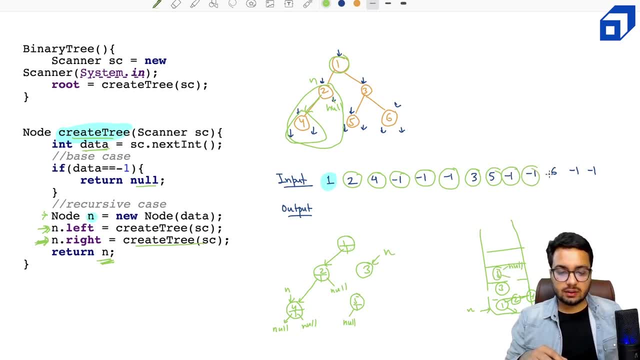 so five left is null. again you read minus one, so five's right is also null. then you return n, so you return five. five gets attached in the left of three, so five is returned. it gets attached in the left of three, so five goes here. then again, what's going to happen? you'll say: okay, i want to build something on the. 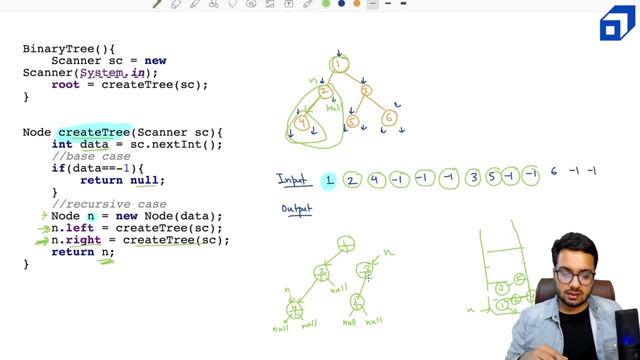 right of three. so three is left is done, three is right's turn. so i'll again make a call. it will read six. a new node will be created, six, okay, and again you say okay, i will read the left, which is minus one, i'll read the right, which is also minus one, and then i will return n when you. 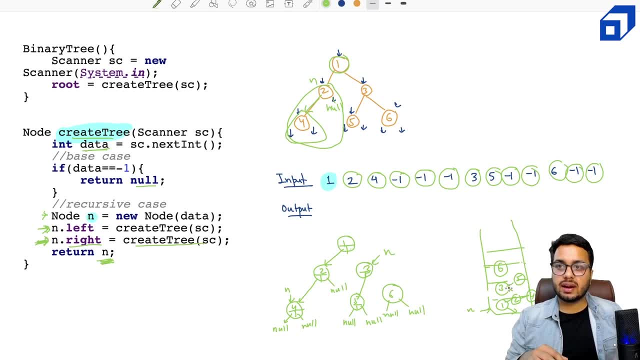 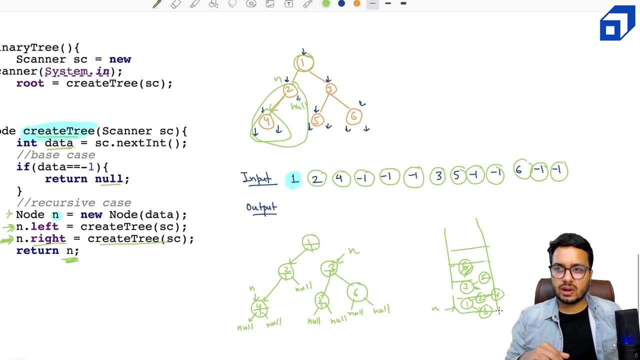 return n, this six is returned back to the right of three. so this six is being attached here, okay. and then you say, okay, i'm going to return n. so when you return n, you return this three back to 1. so once, once, right is going to point to this subtree 3, 5, and this subtree is attached. 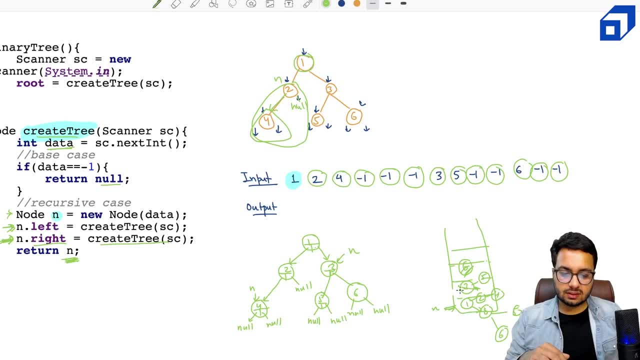 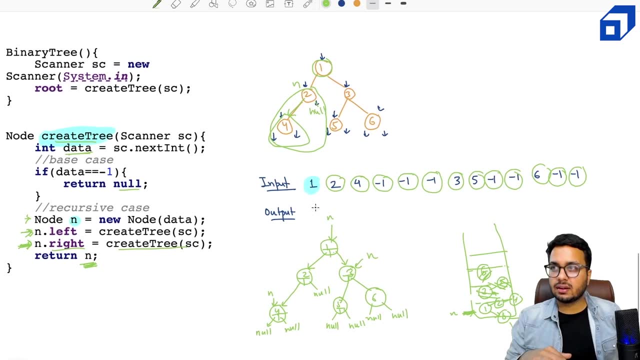 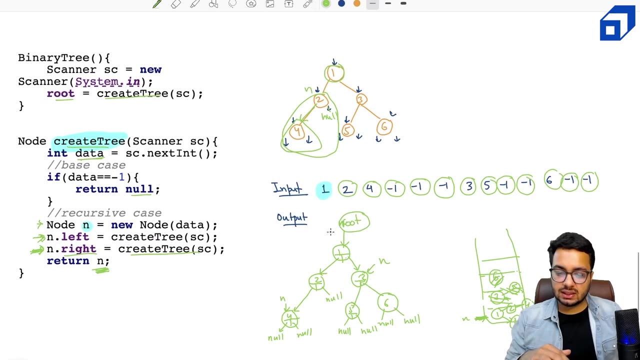 with 1. so finally, when you are here, this call is over, right, so you will return n. so n will be this node and it is returned back here. root equal to create tree: this: this becomes the root of the tree. so root is a data member of the class and hence root of the tree gets updated. 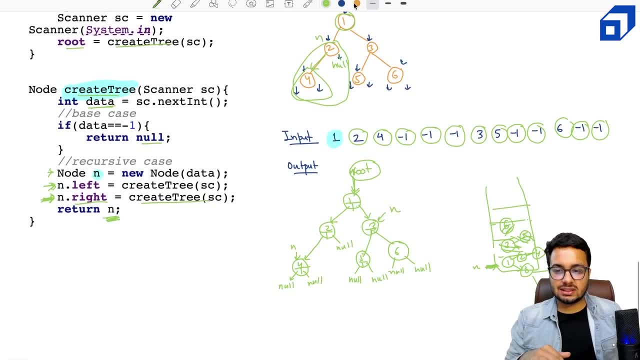 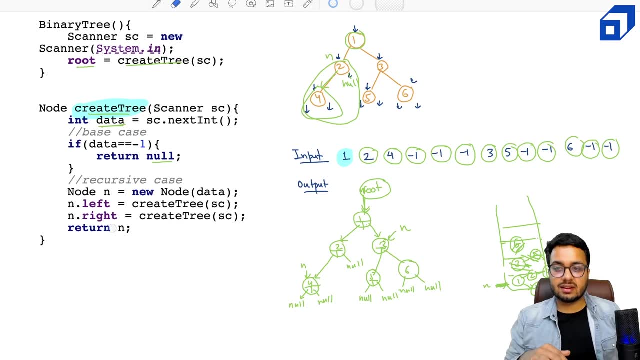 i hope you are now convinced that how this structure can be made so easily with this recursive function. okay, with this recursive function. okay now this way of building the tree. it is called as pre-order. right pre-order means first we are building the root node, then we are building the left subtree. 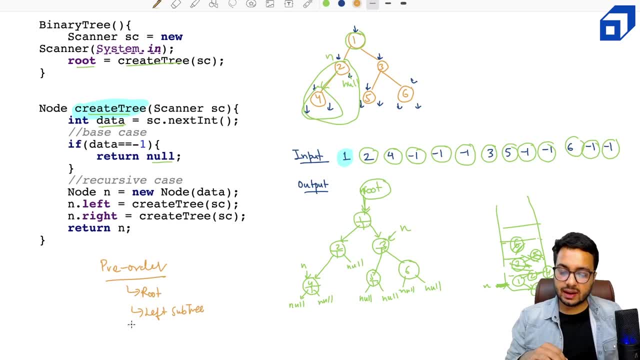 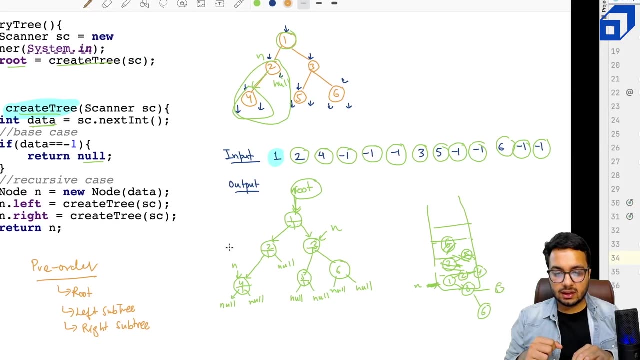 and then we are building the right subtree. then we are building the right subtree right now. we have built the tree using a pre-order recursive build tree function right or create tree function right. next we will look at how we can print this tree in a similar way. now let us talk about tree. 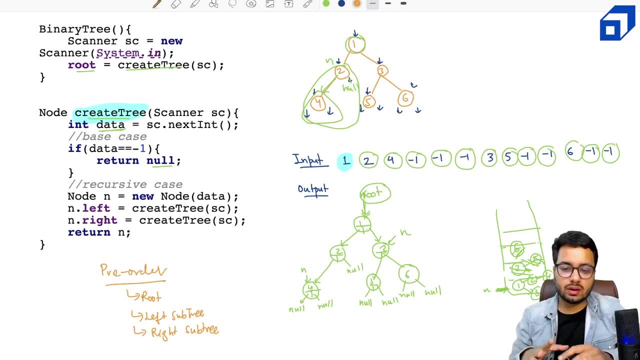 traversals. okay, so tree traversal is a way to iterate over all the nodes of the tree. right now, this traversal can be helpful if you want to perform operations like counting the number of nodes, searching for a given node, updating a given node, right. so in order to do all these operations, we must know how to. 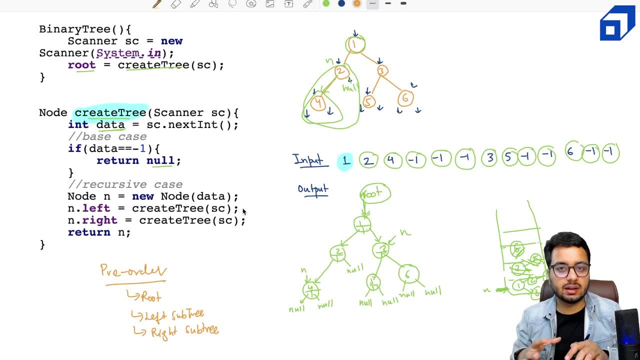 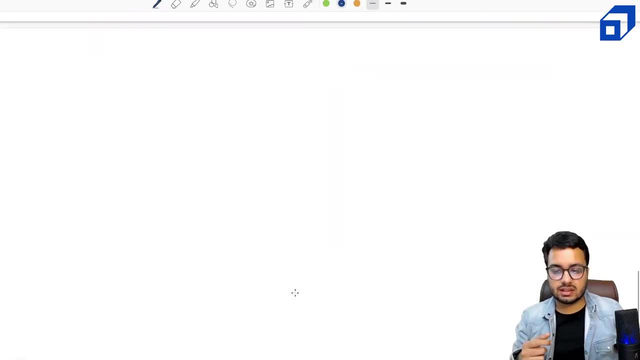 traverse a given tree, right so? a tree has been built, a tree has been created. we want a way to go to each and every node of the tree, right? so, as I discussed, if you want to do a tree traversal, there are two broad techniques. right so, tree traversal, right so one is your. 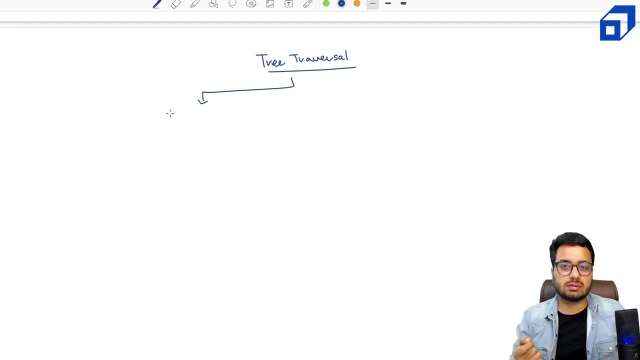 recursive technique that, okay, you start with the root node, then you iterate recursively on the left tree and the right tree, right. there is a recursive way of doing it, there is a iterative way of doing it, right. so we will discuss all these ways now, right. then recursive way again, there are 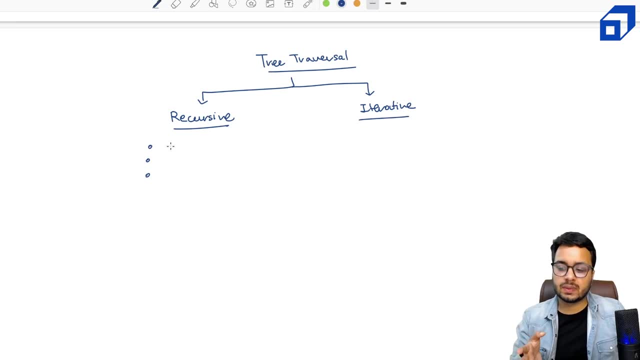 it depends upon the ordering. okay, the way is same. we basically recursively iterate on the left and right subtrees, but based upon ordering, there are three different ways. one is called as pre-order traversal, one is called as in order traversal and one is called as post order reversal. you will be. 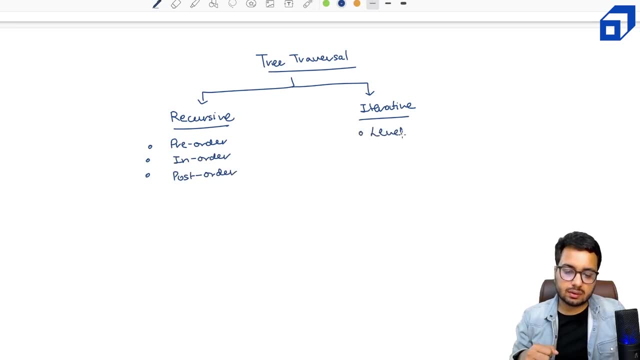 looking at all of them in iterative, there is only one way. that is called as level order reversal- right? so all of these traversals, they are going to travel all the nodes, but the order in which you will see the output it will be different. so let us start with the pre-order traversal. given this, as 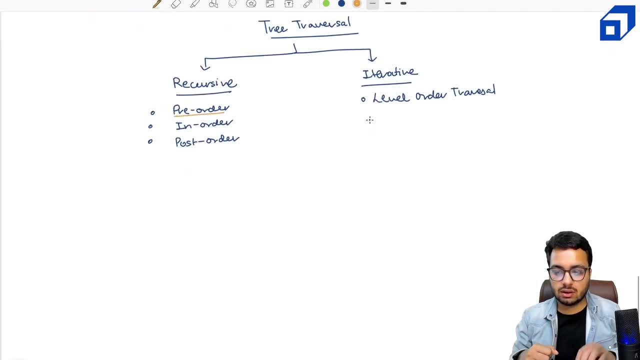 the tree right: one, two, three, four, five, six. so I will just redraw this tree: one, two, three, four, five. now what is this pre-order traversal says that. fine, what I will do? I will travel the root node, then I will recursively traverse the left sub tree. okay, 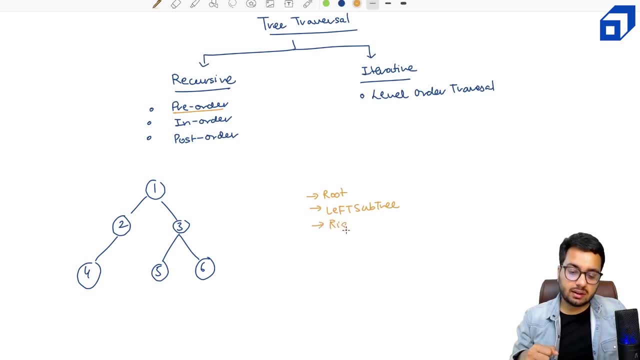 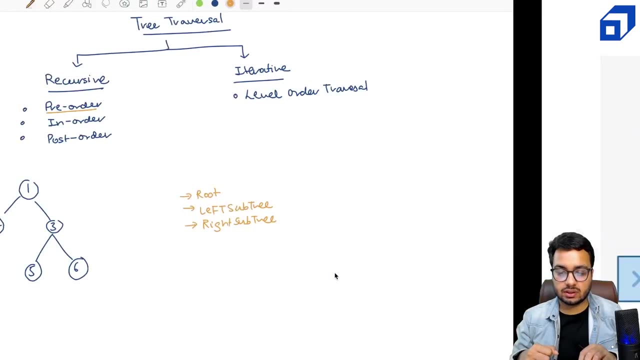 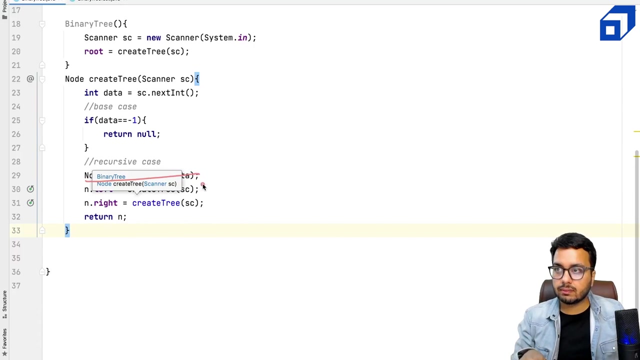 this will be a recursive call and I will recursively travel the right sub tree- again a recursive call. okay, it is very similar to the build function. what we are doing in the build function also, if you look carefully, we are first building the root node and then we are recursively building the left tree and then we are recursively building the. 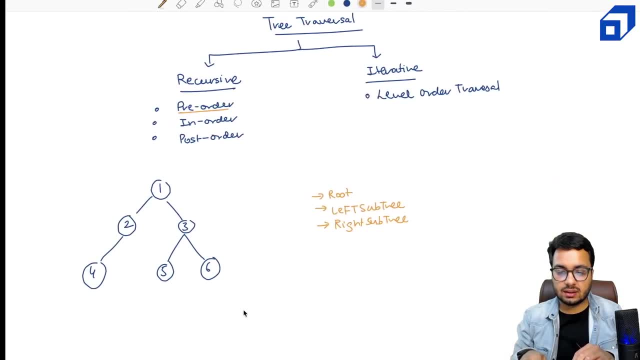 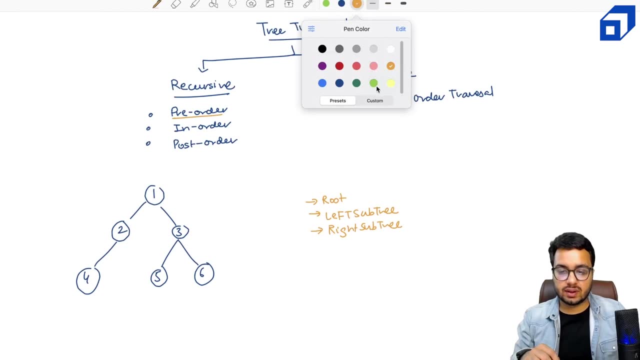 right tree, right. if you see, in this case the output will be very similar to the order in which you have built the tree. so if you start traversing, you will say, fine, I will start with the root node, I will print one, I will go to the left sub tree. so this hole is my left sub tree, so I 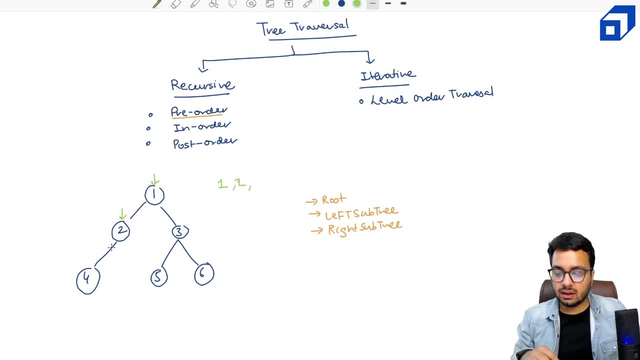 will print the root node, that is, two, and then I will go to the left sub tree. so left of two is four, I'll print four and I will go to the left. now left is null, so I come back. I will go to the right. right is null, I come back. a four is done. this whole tree has been printed, so I come back to two. 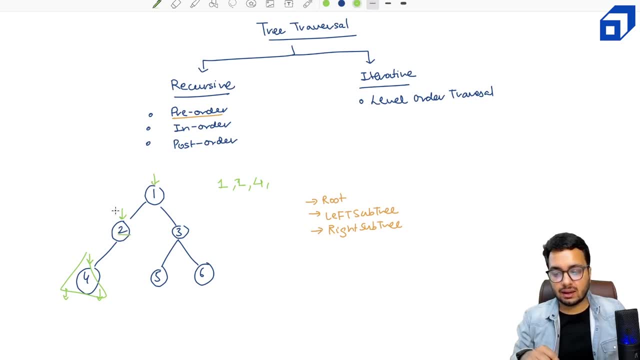 I'll go to the right of two again. it is null. I'll come back. so this whole tree has been printed. I go back now. left of one has been printed, so I go to the right of one. so I come to three. I will print three. I will go left now. I'll print five. I will go left. I'll print right of five- again null, so five. 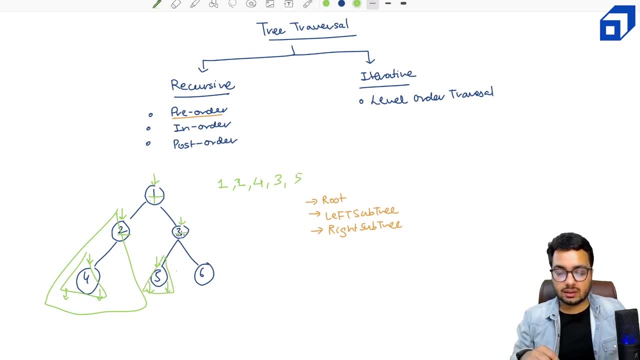 is done, so this whole tree has been printed. I'll go back, so add three, else okay, let's go right, I'll print six, I'll go left, I'll go right, nothing happens. this whole tree has been printed. I come back now. three has been printed, so root has been done, left of three has been done, right of three has been done. 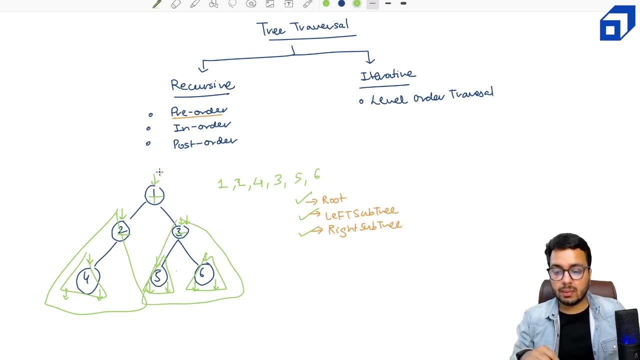 so I'll return. so this whole tree has been printed. I come back and at one I see one has been printed already, because before printing left and right I print one. this output is called as pre-order output, in which before printing left and right nodes I print the root node right. so one, two, four, three, five, six- this. 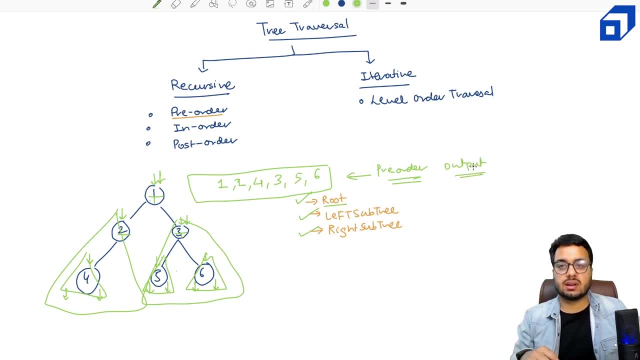 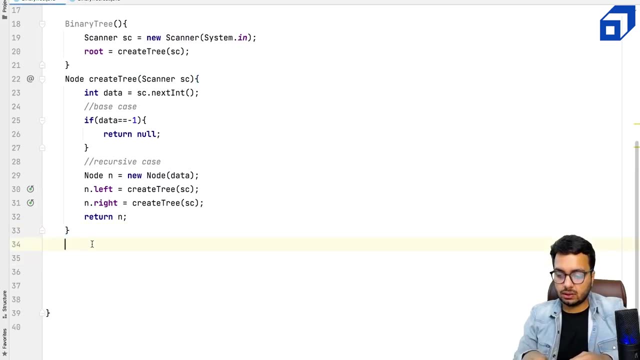 will be the pre-order output for this tree. right now. let us see this thing in in our code as well. let's write a pre-order print method, let's write a method called void display, and this is going to be the method that will display the tree right inside. this logic can be changed. I can display. 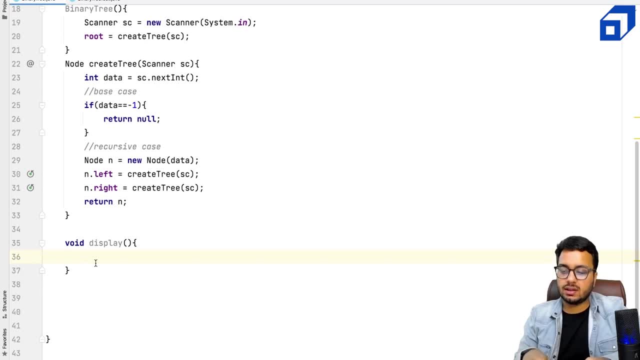 a tree in a pre-order way or in a level order way or any other way, right? so I'll again create one more helper method. so I will say void pre-order. so void pre-order print. now this is a recursive function, so I have to tell at what node I am. 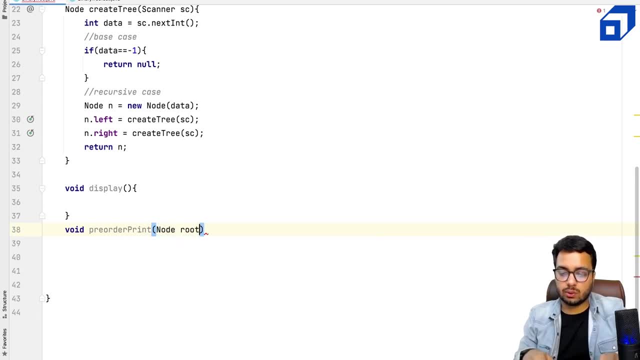 currently at. so I will start with the sum node, that is, root node. okay, so what I will do? I will say: fine, I will have a base case. what will be my base case? what is the smallest tree I can get that? the tree is null. the root is null. in that case, I don't need to print anything. I will simply return. 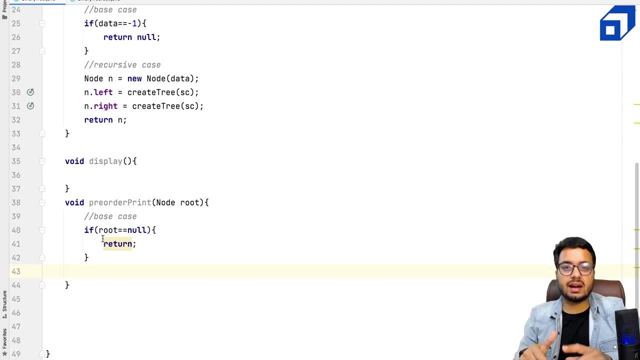 otherwise what I will do? I'll print the root data and I will go on the left and the right tree. so I will define s out root dot data. go and print the left subtree recursively, so pre-order print root dot left, then pre-order print root dot right. that's it. 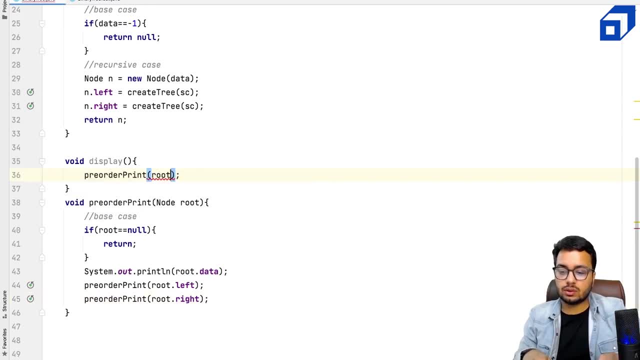 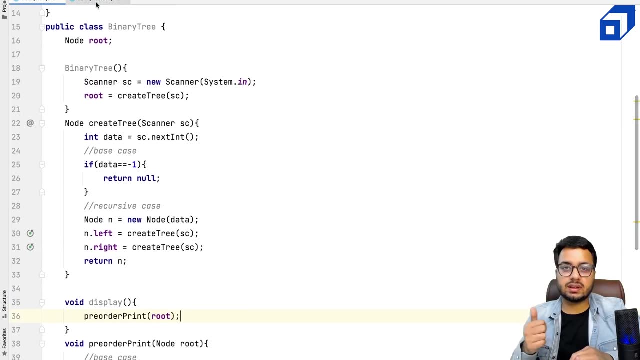 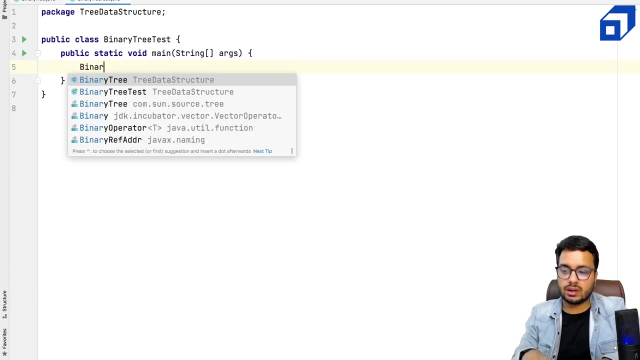 I can call pre-order print with the root of the. now let's do one thing. let us test our binary tree, because we have the create method, we have the print method. now I can create a binary tree and try to print it. so I can define: I want to create a binary tree object. this is equal to. 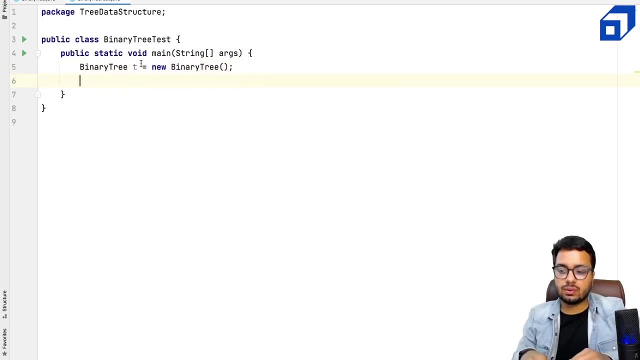 new binary tree. I have defined the class. now, as soon as this constructor is called, your tree will start getting built, because we call the create tree method here right now. I can call t dot display. now think of any tree that you want to make. we will give it as an input here. sorry, I should run. 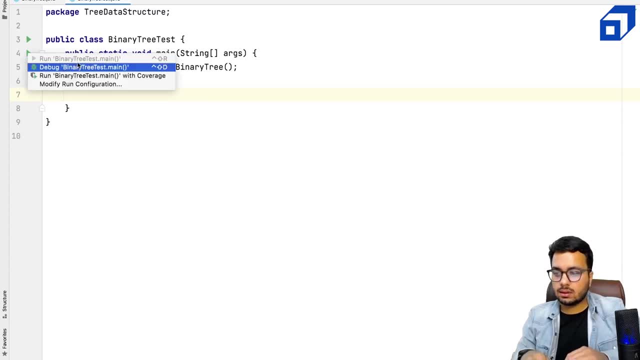 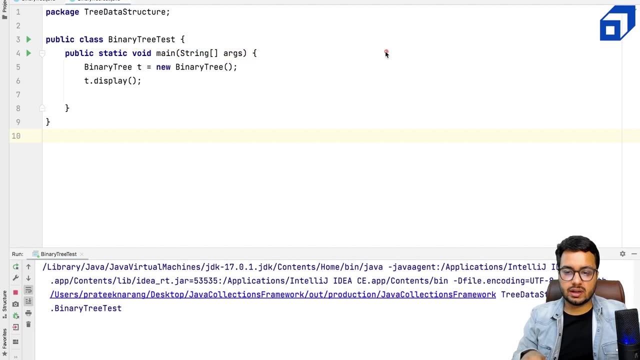 this file. now this is waiting for the input, right? so let me draw a tree. let's say tree is one, two, three, five, six, eight. now how this entry will be given as input. so you will input one, then two, then four, then left of four minus one, right of four minus one, right of two minus one, then three. 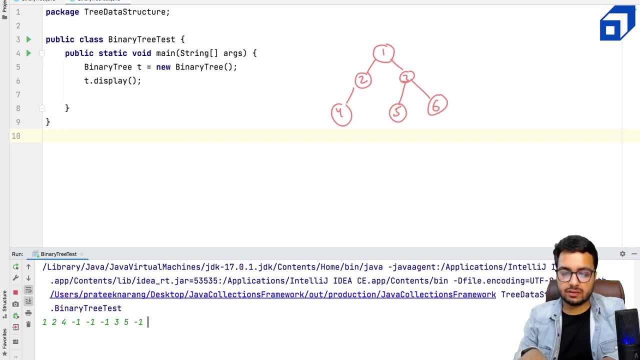 then you will input five left of five, right of five, right of six, right of three. that is, six left of six and right of six. okay, the same input that I have shown you in the example. example also, this input is given. and now I'm saying that let me print this tree, what I'm. 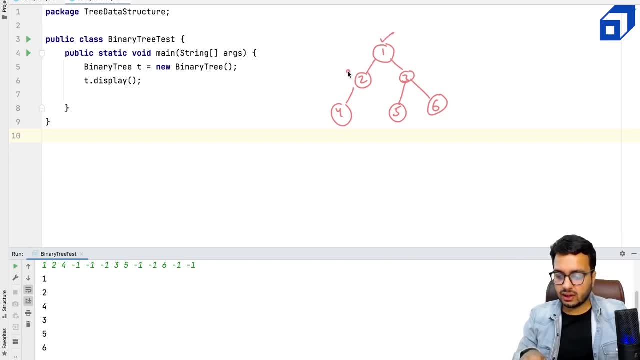 getting. I'm printing one, I go here. then I go to two. fine, then I go to four. fine, then I go to three, I come back, I come back, I go here, yes. then I go here five, then I go here six. absolutely correct, right? so if you look at, this was a pre-order build, right, and this is actually a pre-order print. 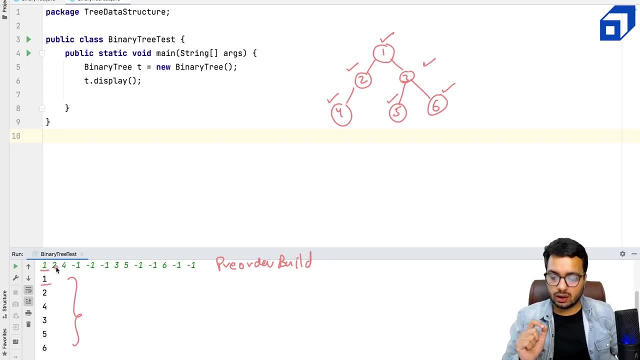 if you see, the output will be exactly same: one, one, two, two, four, four minus one. I'm not printing skip, skip, skip. then three, five, three, five, absolutely correct, minus one. I'm not printing six, six, right, that means my both functions are working fine. tree is getting built correctly and 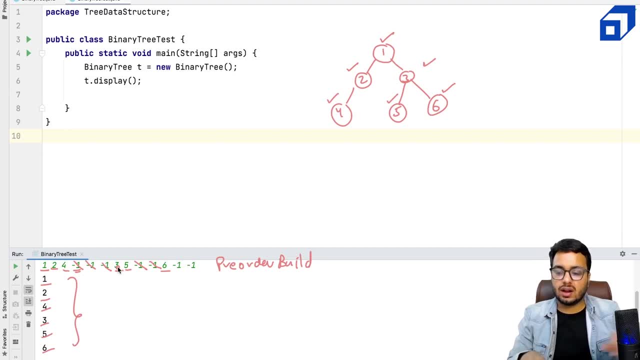 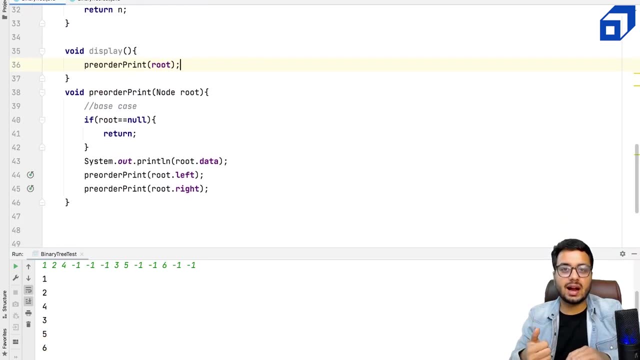 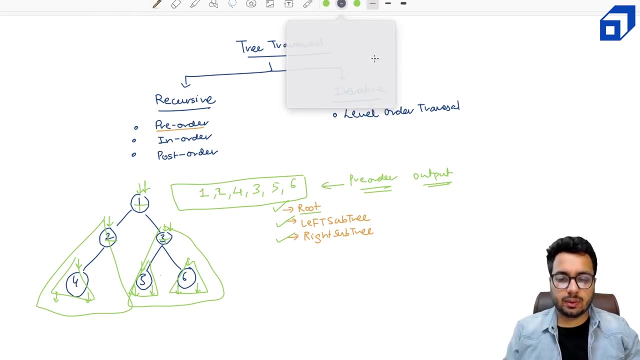 tree is also getting printed correctly as well. right now I will show you two more variations of this print method. that is called in order print and post order print. so now let us discuss the next type of recursive printing that we call as in order print. okay, so I hope pre-order is clear. now we are moving to in order, so nothing is going to. 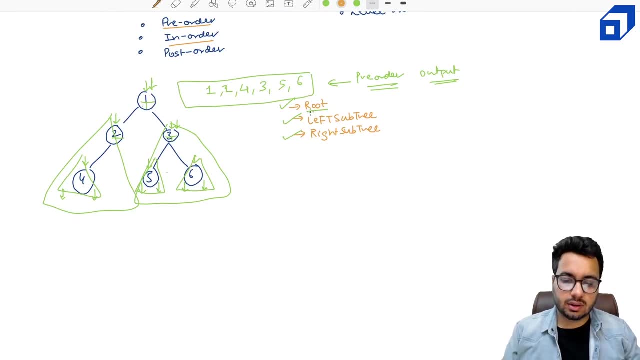 change. the order of printing is going to change. okay, so earlier it was root, left sub tree and right sub tree. now what we are going to do in order means root will be printed in between. so before you print the root, you will print the left sub tree, okay, and after you print the 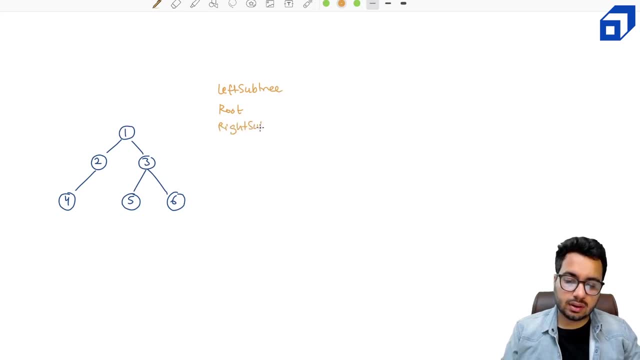 left, you will print the right sub tree. that is what the in order printing would mean. let us dry run this logic on our uh code and see what do we get in order. so what I want to do. so I will start from the root node. I want to print this root node, but before that I will have to print. 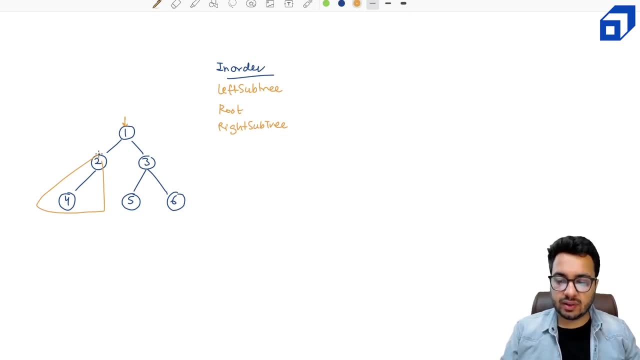 the left sub tree right now. add the left sub tree again. if I am at two, I have to print the left sub tree, so that means I will have to print four. so four will be the first output that I will get. now I will print the root. so what is the root? the root is two. all right, then I 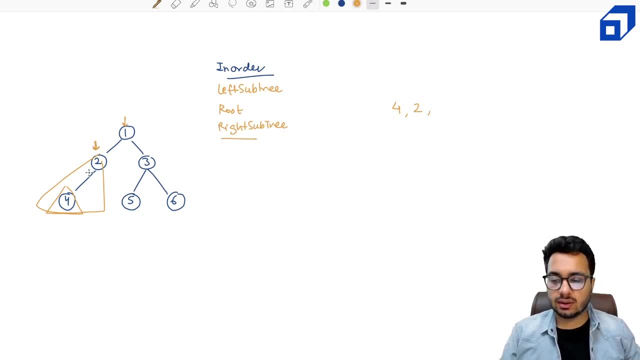 will print the right sub tree. so right sub tree of two is null right, then I can go back to one. so for one, I have seen the left sub tree is already printed. then I can print the root. so I will print one and then I will print the right sub tree. now I am at three right before. 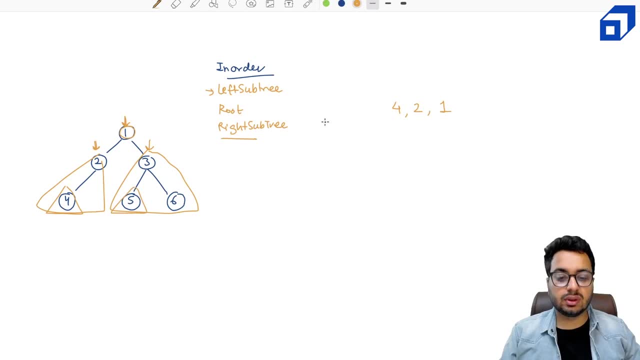 I print three, I will have to print the left sub tree, so only one node. I will print five. then I can print the root node, that is three. then I can print the right sub tree, that is six. right, this will be the output we can expect by traversing this uh three in a in order fashion. so let us jump into 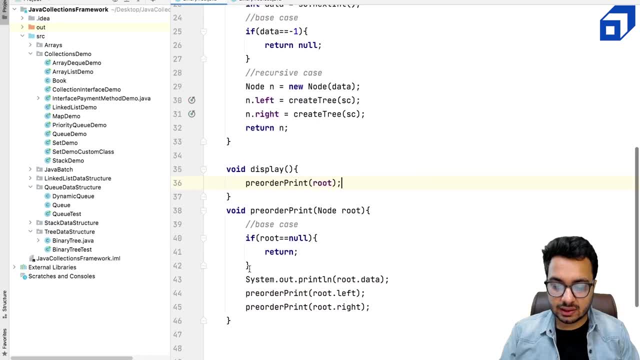 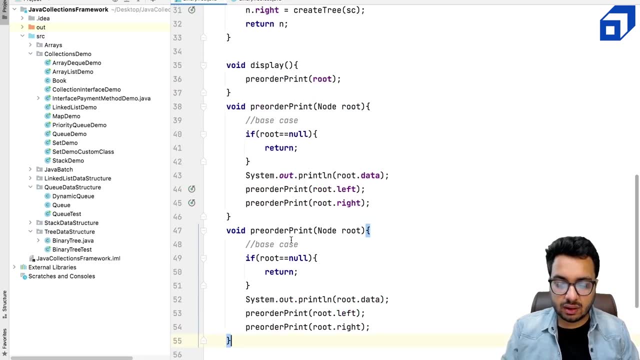 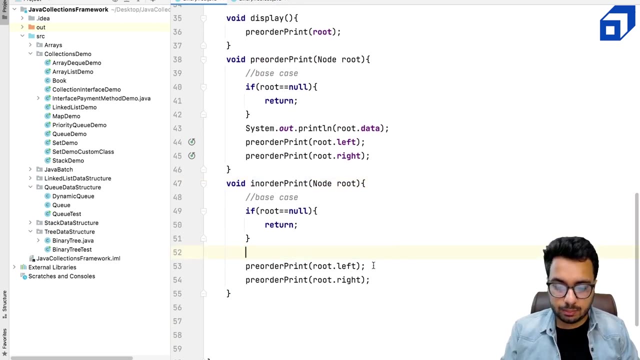 the code and see what we will change. right, just like the pre-order print method. what I will do. I will create one more method called as in order print. so in this case the root will be printed in the middle and this call will be now in order print. 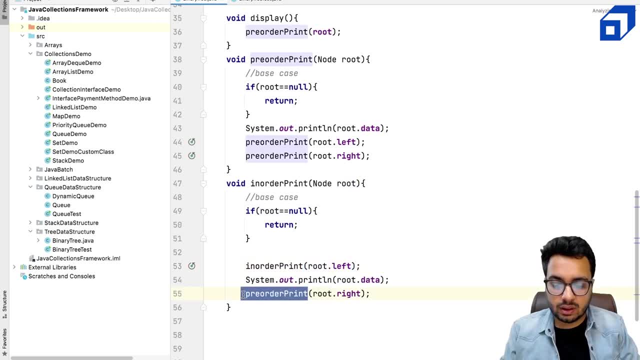 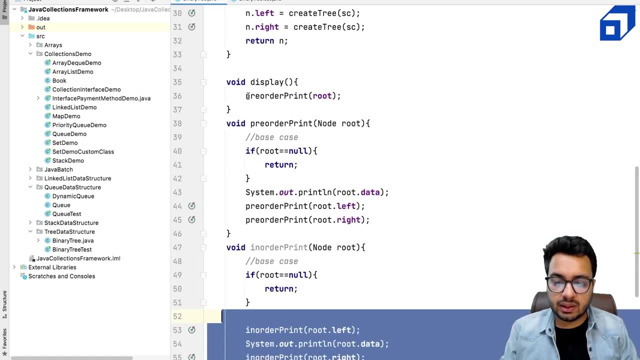 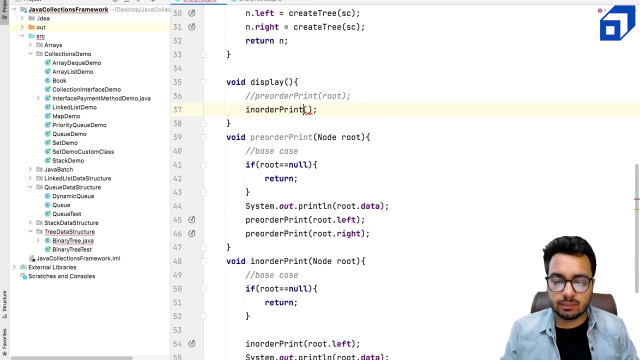 root dot left. and this will be now in order print: root dot right. okay, now in the display method, instead of calling pre-order print, maybe let's just call in order print. this time I want to display the tree using in order print. I will pass the root of the tree as a parameter here. 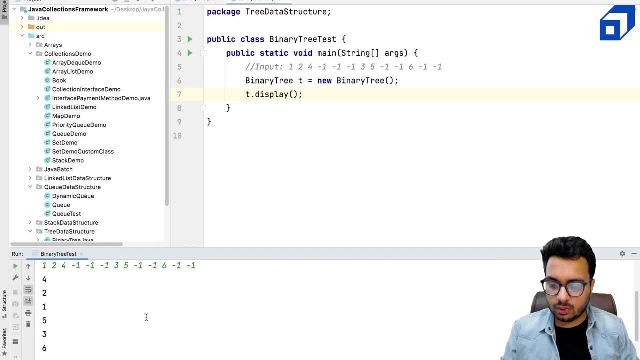 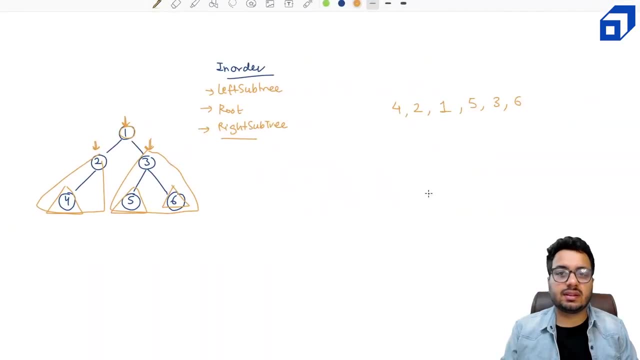 let us give the input for this tree and see what output we get. we are getting four, two, one, five, three, six. is it the expected output- four, two, one, five, three, six? the answer is yes. right now, you might be interested in doing a call stack analysis of this, right? so let us see how we can do the call stack analysis as well, right? 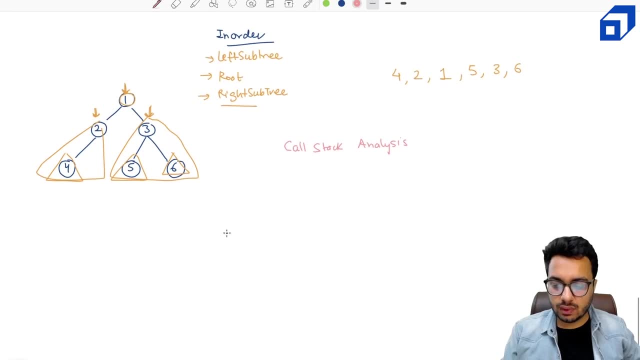 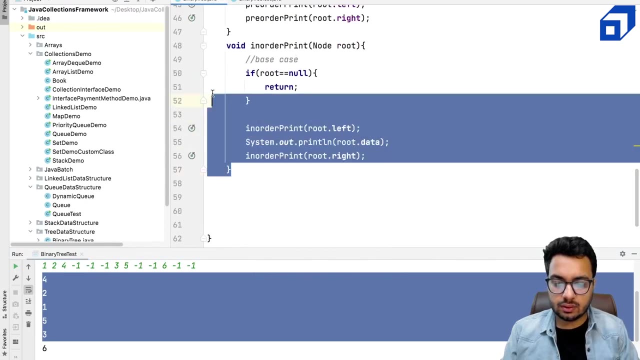 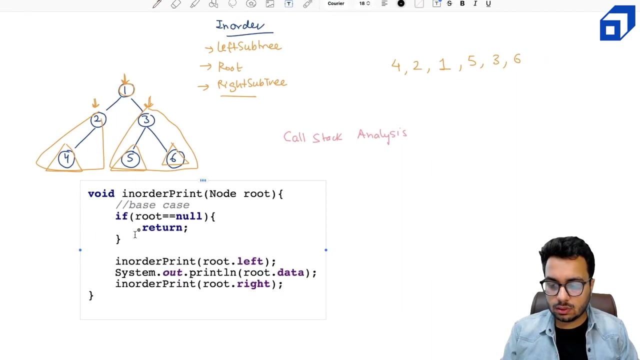 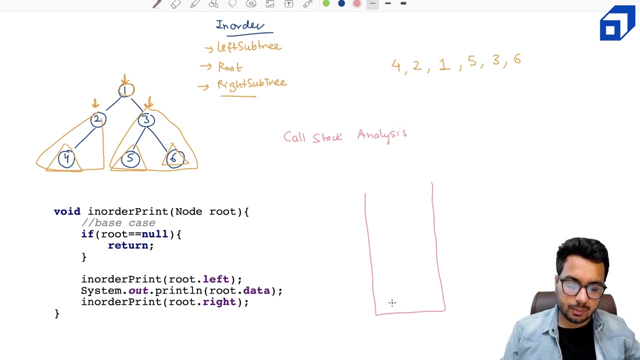 in the beginning. what is happening? uh, let me also copy paste the code. this is the code, right? let us do the call stack analysis. this is the method that we are calling, right? so the call stack is empty. so we called in order print where the root node is one. so I say root is. 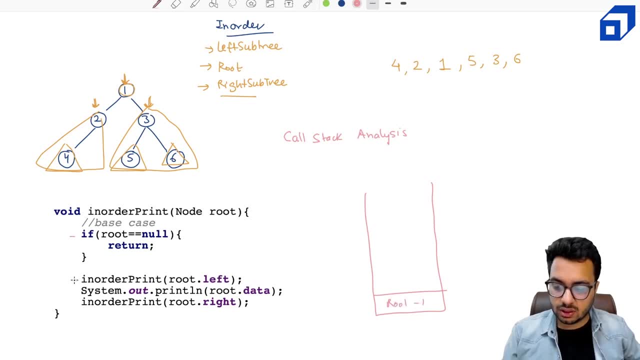 one, but I'm not going to print it. so root is not null. I will just call on the left. so I make a call here. right? so that means root is now two. I am at this node, but I'm not going to print it again. I make a call on the left. that means root is four. okay, I'm not going to print it because root is. 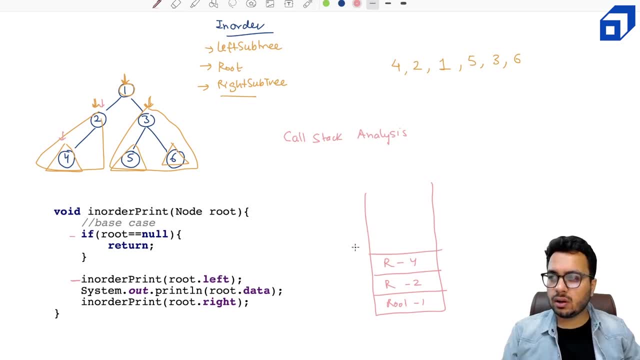 not null. again, I make a call on the left. when you make a call on the left of four, you actually come here. this is null. so if this is null, you return. okay, so you return, then you make a call, then you print the root data. so that means you print four. this is the top of the stack and this is the root. 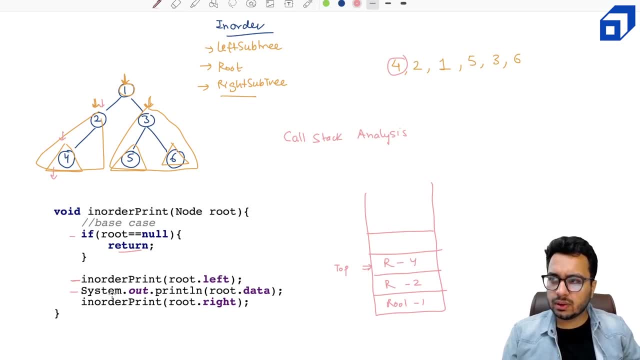 that we are talking about. so you will print four. then what's going to happen? you will say, okay, I'll go right. so right is null. again, you make a call to null and you return. so you come back. so again, you are here now for four. you. 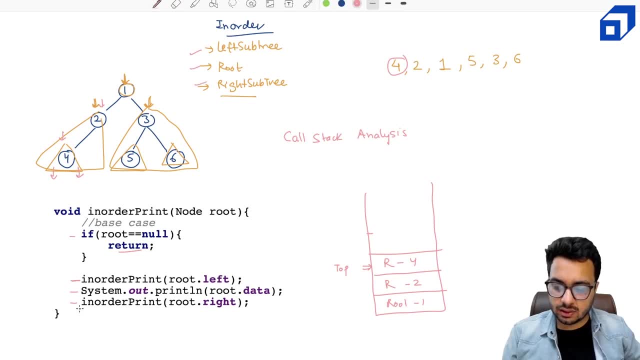 have done all the three things. left is done, root is done, right is done. so you return. so from here you go back and this is gone from the stack right now. what is the new top right? how do we come back to two? this is how we come back to the two. so the new top is this: now, this is the root node. 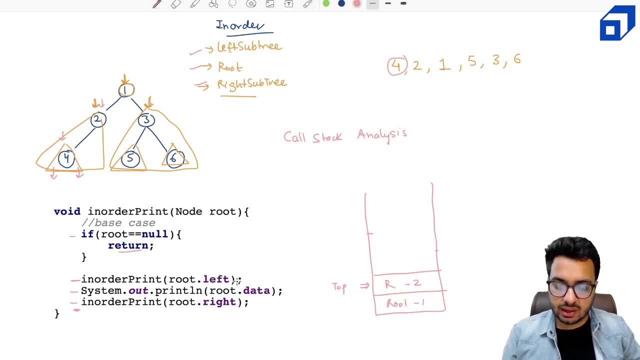 that is currently we are talking about. have I printed the left? yes, have I printed root dot data? no, I will print it now. have I printed the right? no, so I make a call on the right of two. that is null and I again return. then this is done. so I come back now. what is the top node? the top node is one. 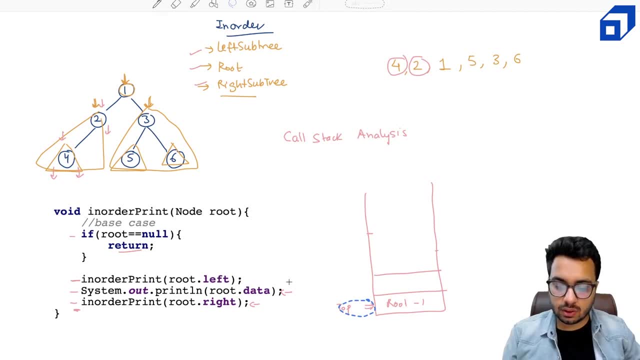 so have I printed left? yes, have I printed root dot data? no, I will print one and I will make a call on the right. so I make a call on this tree right. so again you do a similar process. you come at three right, so root is three. then you make a call on the left. that is, root is five, so five left is. 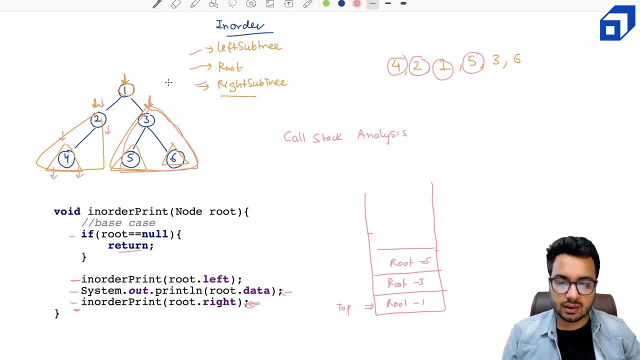 null. so you print five. five right is null. you come back, so five is done. then you go back. the new top is now three. right, it was five, now it is three. so three says okay, my left is done, I will print myself and then I will go right. so root will be six. so you come here right. so you went here then. 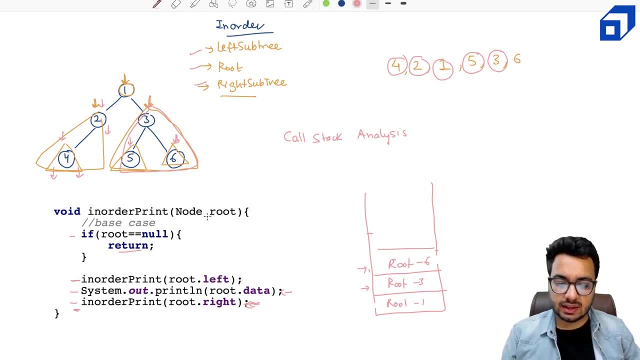 you claim here six. now root is six. left and right they are null. so six will get printed. right is null, right, and then six will be popped off, right then. so for three: right is also done, so this call is over and you come back at one. so for one: left is done, root is in. right is done, so this call is also over, right. 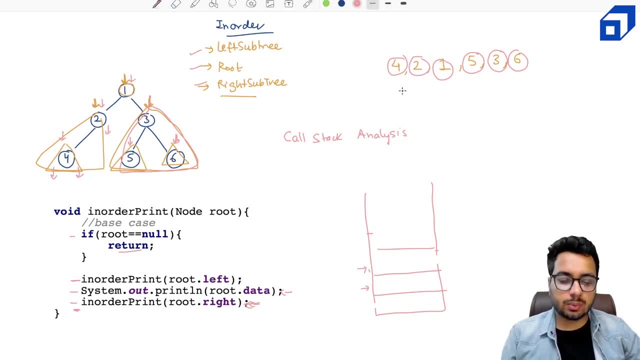 finally, the call stack will be empty and this is the output that you will get right. so I hope you have understood the in order traversal. now make a bigger tree and try to uh generate the output for that particular tree, right? and next I will discuss post order traversal. let us talk about post order print, so, as the name 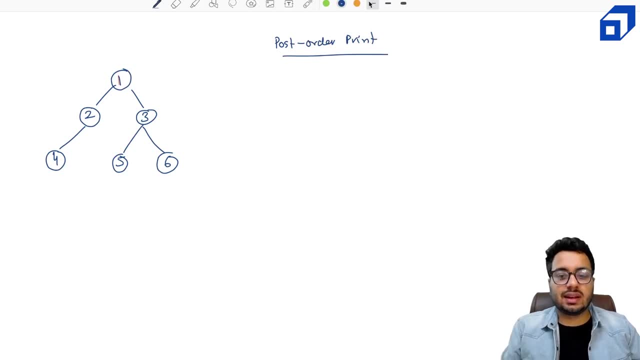 suggests. post means the word after. okay, in this case, what we do? we print root in the last. so first we print the left sub tree, then we print the right sub tree, recursively of course, and after then we print the root, right. if this is the tree, once again, what I will do? I start with one, but I have 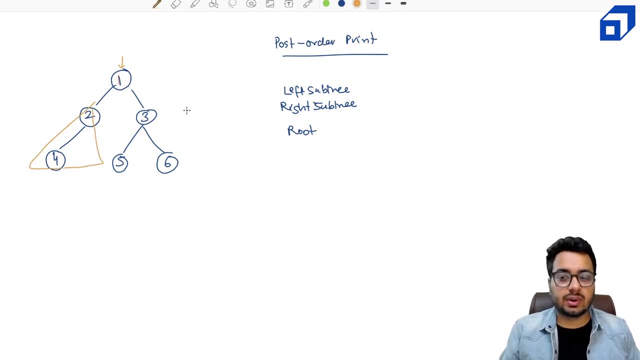 to first go in the left sub three. then I have to go in the right sub tree and then print one right, back two. I again have to print left sub tree. that means I will print four right. then I will print the right sub tree. so write of true is null, then I will print two. so I will print two then at 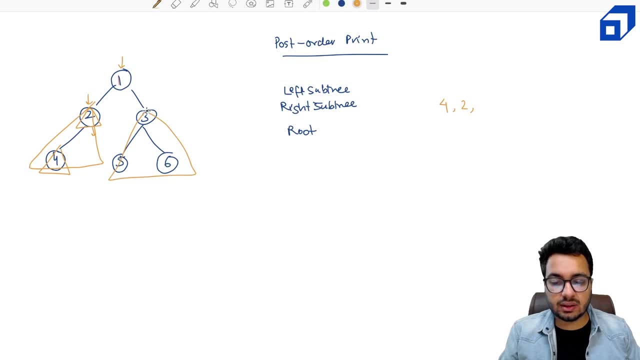 one. I have to print left, which is done. I have to print right sub tree and then print root. so at 3 I will print left sub tree, which is 5, then print the right sub tree, which is 6, then print the root, that is 3. 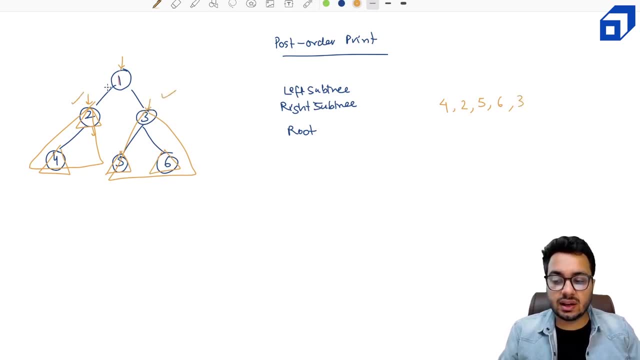 now for 1. left sub tree is done, right sub tree is done, then I can print the root, that is 1. this is what the post order output would look like. you might be asking: why do we need so many traversals? for example, what happens in certain problems is: 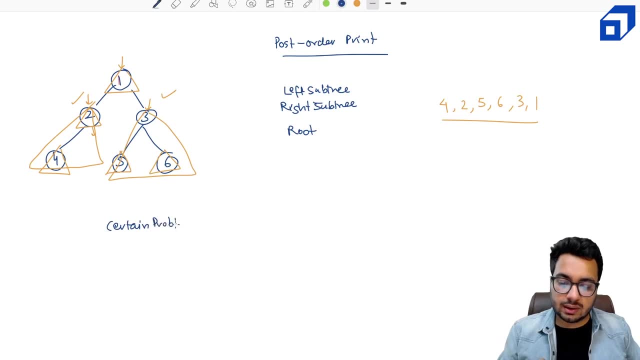 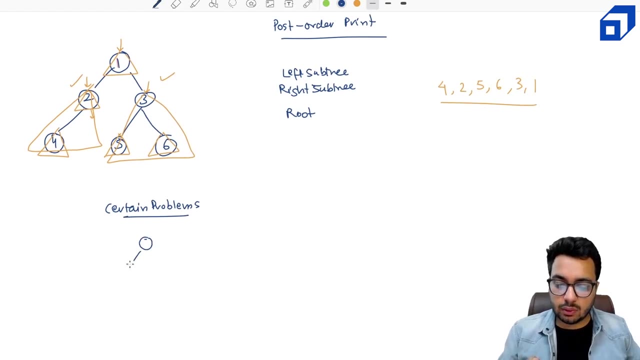 in certain problems. you are expecting that. you are expecting output from the left and right sub tree. for example, given a tree, I want to calculate the height of the tree. for example, I want to calculate what is the height of this tree. so, in order to calculate height, what you will need, you will need. 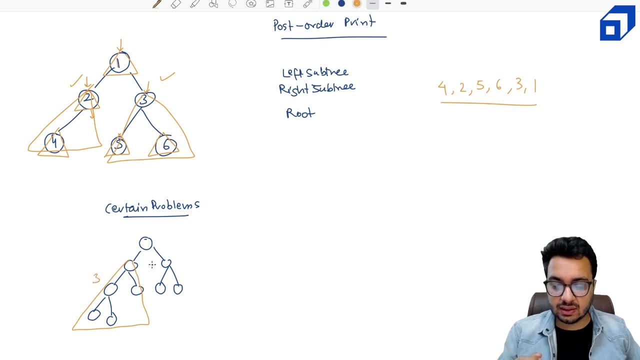 to know that. what is the height of the left sub tree? let's say this height is 3. what is the height of the right sub tree? this height is 2. then can you say recursively: at this root node: the height is nothing but it is the maximum. 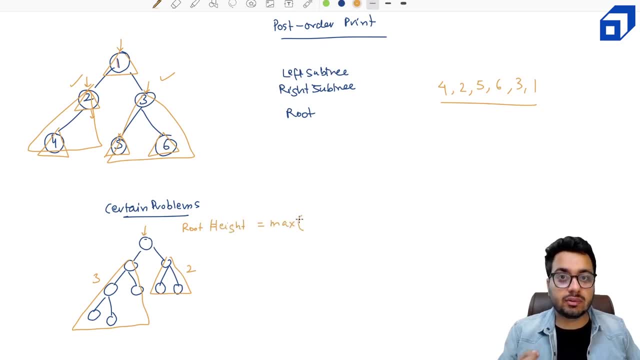 of left and right. ok, maximum of the answer that you are getting from left comma right and 1 more than that. so can I say the height will be 4? what is this? this is the answer from the left sub tree. what is this? this is the answer from right sub tree. so what I am. 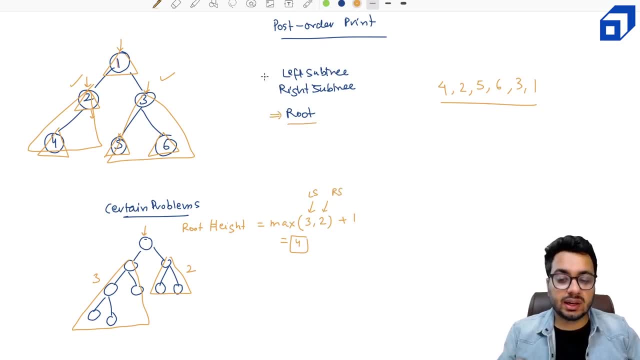 trying to claim is, in order to build the answer at the root node, you need the answers for the left sub tree and right sub tree and hence, in problem like these, you would of course need a post order reversal right. so that is the idea. when you need answer. 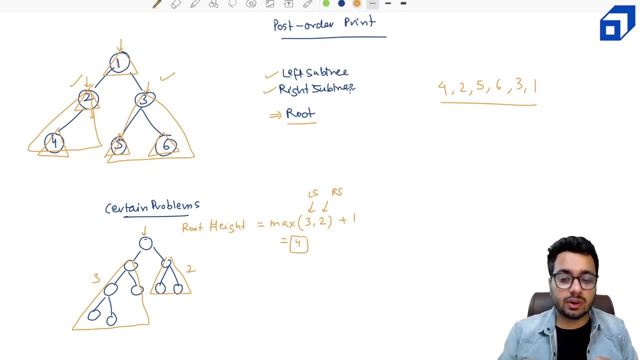 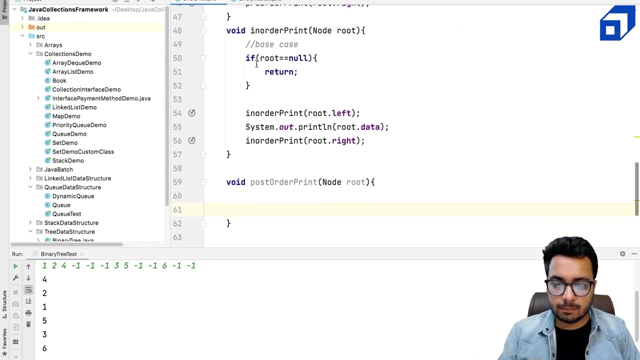 from the child sub trees to calculate the answer at the root node. you will definitely need post order reversal there, right? so now let us write the code and then we will do the dry run of that code. writing code is very easy, so I am in the in this class. 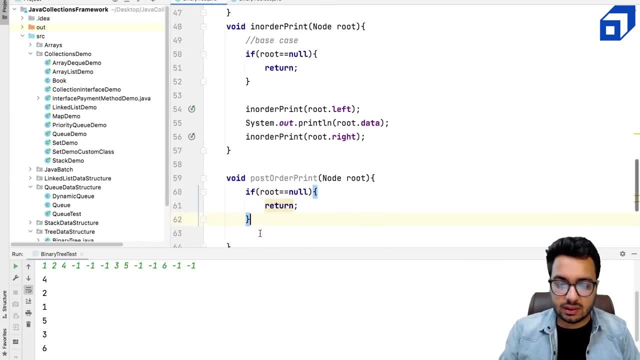 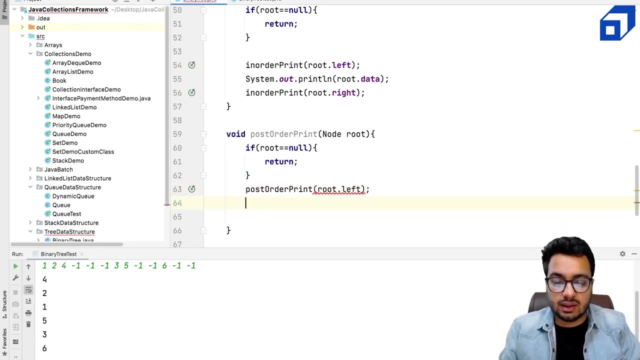 if root is null, I will return right. then what I will do? I will go on the right left: post order, root dot left. then I can say post order: print root dot right and then I will print the root node. so sout root dot data. right now let us go and 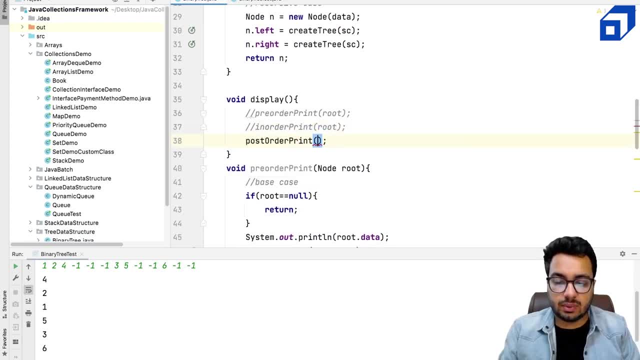 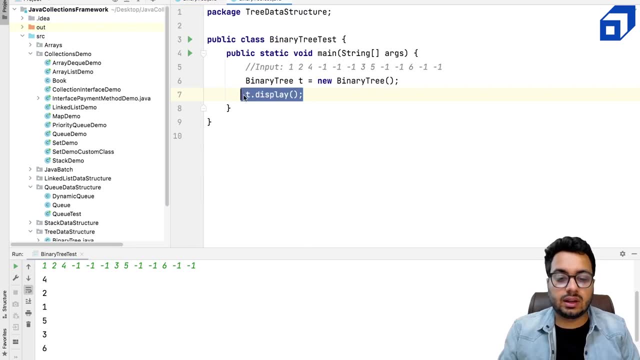 call post order print in our display method. so I can just pass the root here. so t dot display. it is calling the post order print method. now for the same input. let us copy this input and we will see what output do we really get? now we have given the input. 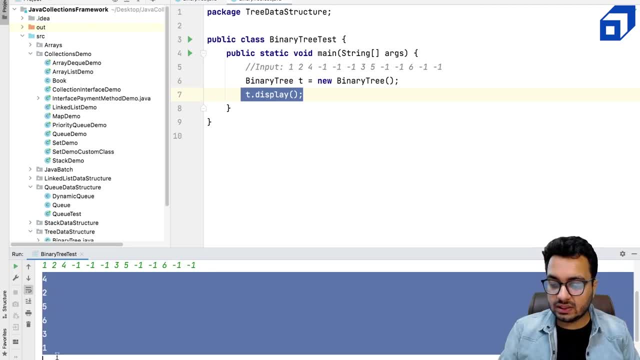 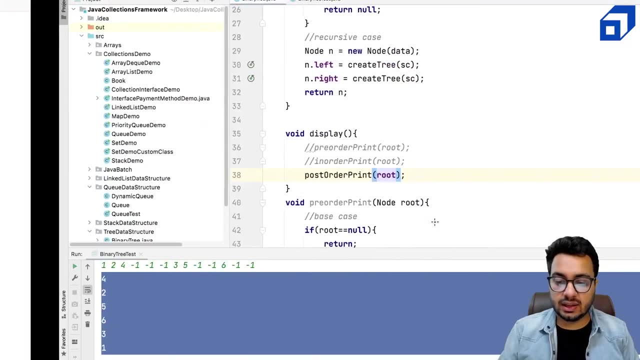 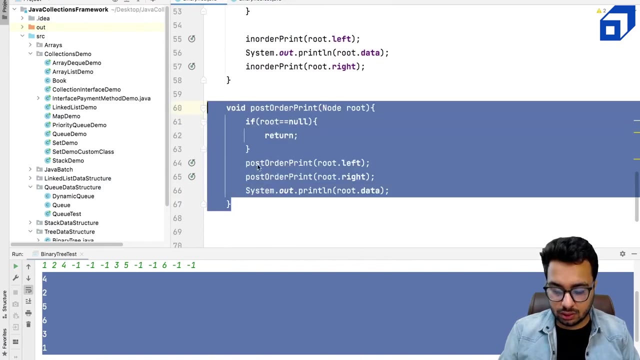 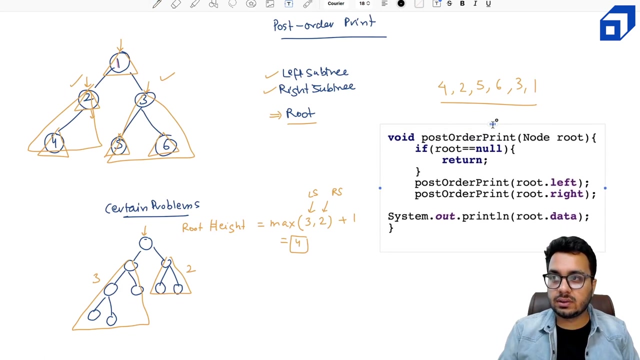 I am getting 425631. is it the same output as we have got 425631? absolutely, yes. now let us do a quick call stack analysis of this method as well. so I will copy the code, I will put it here and let us do a quick. 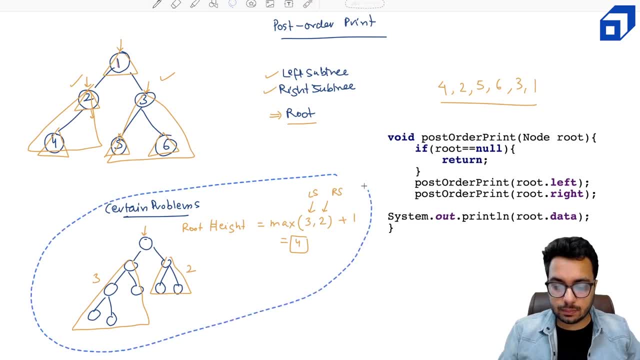 call stack analysis. let us say this is my call: stack. in the beginning I give 1 as my root node. root is 1. then I say, ok, make a call on the left. my root is 2. I make a call here now. code is paused. right call will happen later. 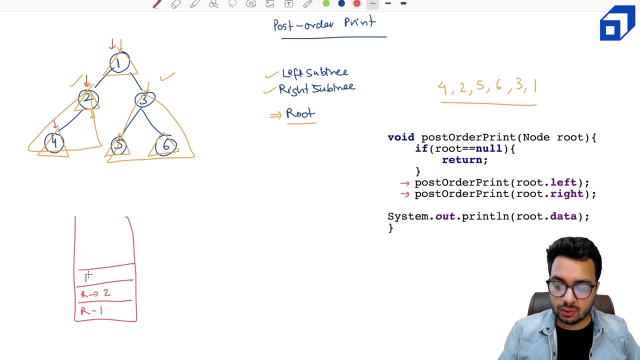 again at 2. I make a call on the left. I come here. root is 4. 4 makes a call on the left. left is null, I return. then 4 makes a call on the right. right is null. again I make a call and return. now I can say print root dot data. 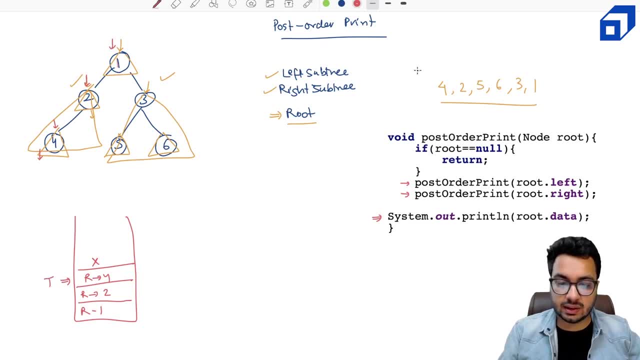 I will print root dot data. this is the top of my stack. I will print 4. then if 4 is gone from the stack, what is the new top? the new top is 2. that means I am in this function. I am at 2, so I am printed. 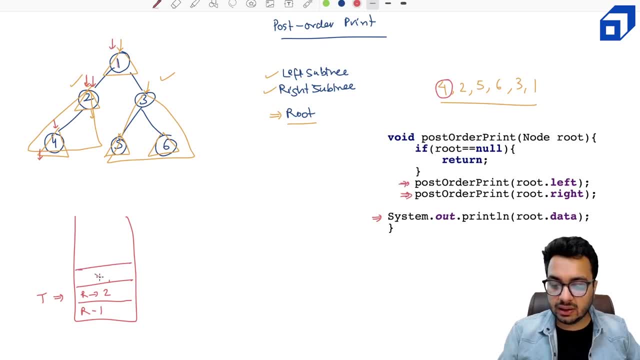 the left. I make a call on the right, so 2 says ok, go and print the right. right subtray is null. I return. then what happens? left and right? they are done. I will print root dot data. that means I will print 2. now. 2 is also gone. we are done. 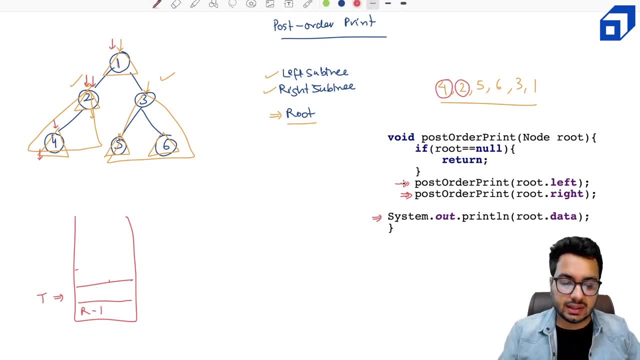 1 is at the top of the stack now. at 1 I said ok, go left, which is already done. left is done, go right, I come here now. 1 makes a call to 3. now 3 says ok, go left. so 3 makes a call. 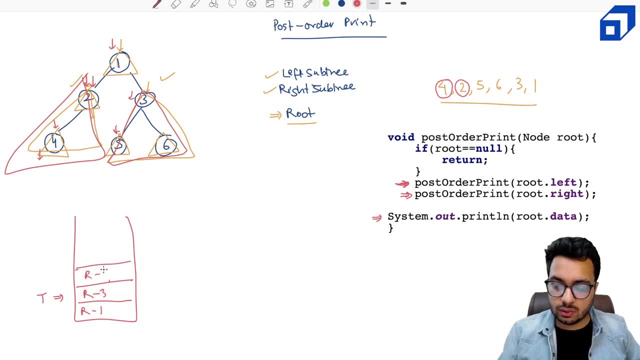 to 5. R5 goes here and R5 says: ok, go left, which is null, go right, which is null, and hence you print 5, so you will get 5 as the next output. now, once 5 is gone, you are back again at 3. 3 says ok. 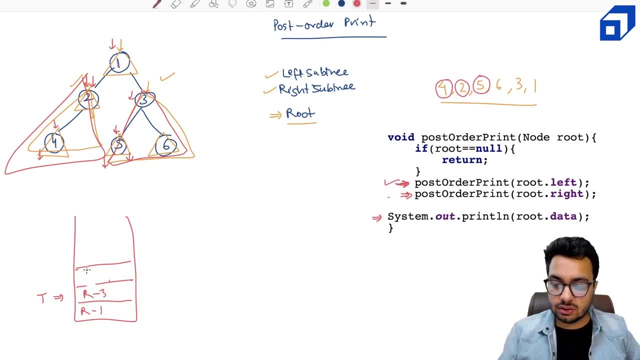 my left is done, this is done, I will go right. so I go to root node. that is 6. root becomes 6 in this call. so this is the top 6 says go left null, go right null, and hence you will print 6, and then 6 is also. 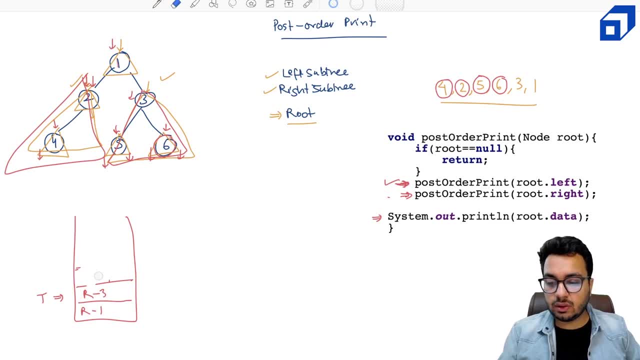 gone from the call stack. then what happens? you are at 3. 3 says ok, my left is done, right is done. I will print root dot data. so I will print 3. I will print 3. 3 is also gone from the stack and now top is. 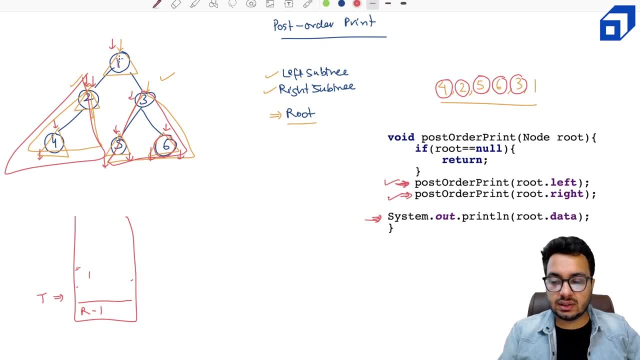 at 1, so for one, left is done, right is done and hence you will print the root dot data, that is: 1- right. this is the output of the post order print. I hope you have understood post order traversal. next we are going to discuss the level order. 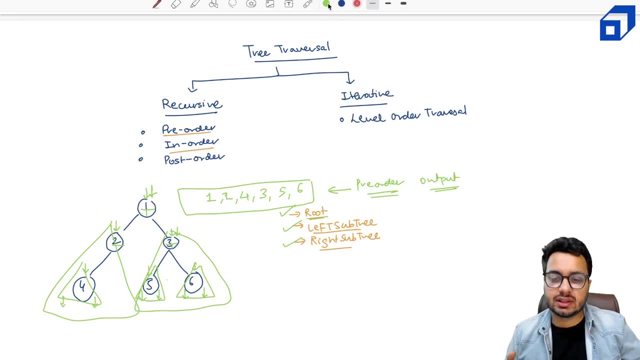 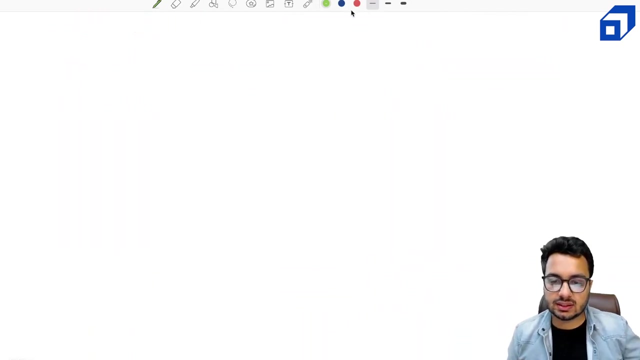 traversal. ok, let us jump into the iterative traversal, which is also known as level order traversal. ok, so that means we won't be using recursion. we would be using some kind of iteration to iterate on the tree. ok, some kind of loop, ok. so let us take this example. 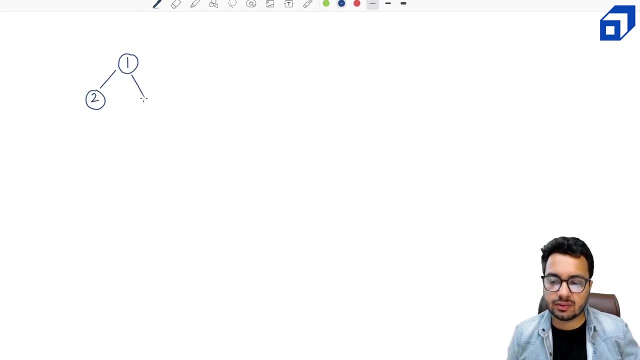 of tree once again, and idea is, instead of going in a depth, first manner: ok, so in all the traversals that we have done so far, what is happening? we are starting from the root node, we are going here, then we are going here. so all these traversals, 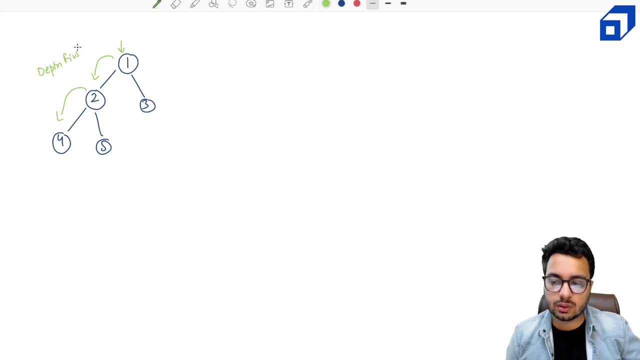 they are depth first traversals. that means you first go deeper into the tree and then that's how you iterate, ok, your pre order, post order, and, in order they are: depth first traversal- right, but now the traversal that we are going to do. now it will be a breadth first. 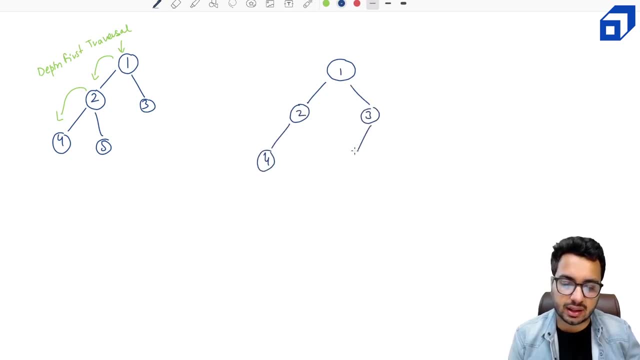 traversal. that means if I have a tree like this, I will be going across the breadth of each level, this level, this level, this level right. that means I can expect an output that is 1, 2, 3 and 4, 5, 6 right. so level order traversal. 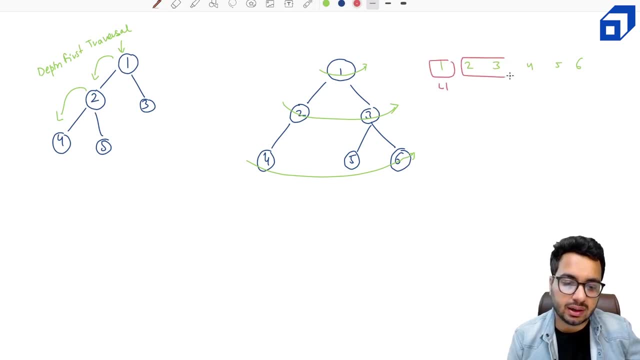 so this is my level 1, then I am printing level 2 and then I am printing level 3. ok, what is the level? all the nodes which are at same distance from root node. so level 1: all the nodes are only one node. it is at distance 0 from the root. 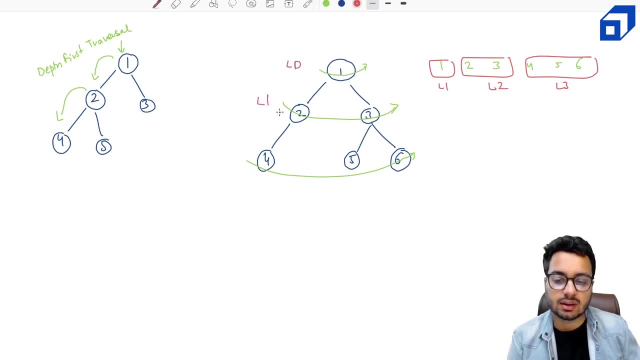 node, or let's say level 0, level 1- all the nodes are distance 1 from the root node. and this is my level 2- all the nodes are at distance 2 from the root node. ok, so this is also known as breadth first traversal. 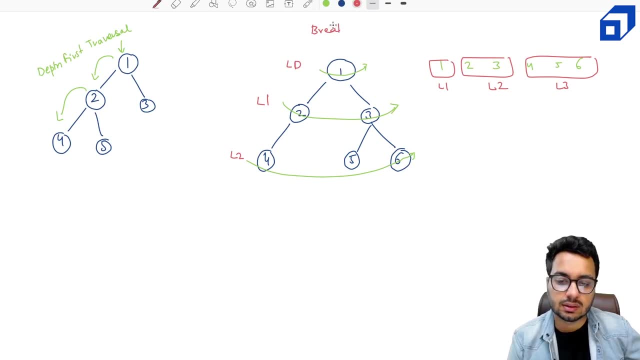 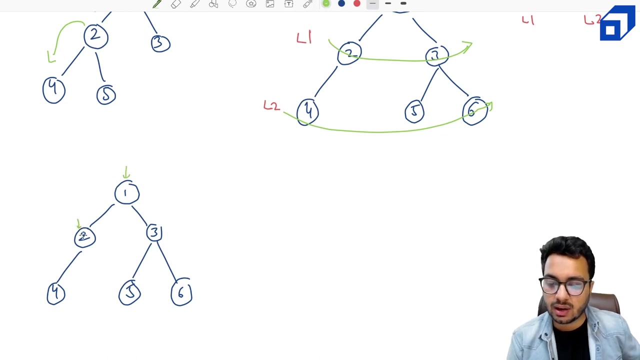 right breadth. first traversal: right now let us see how we can achieve this kind of a traversal right. let's draw this tree once again now. if you look carefully, if you start doing any traversal, that is a recursive traversal right from 1 you come to 2 right and at 2 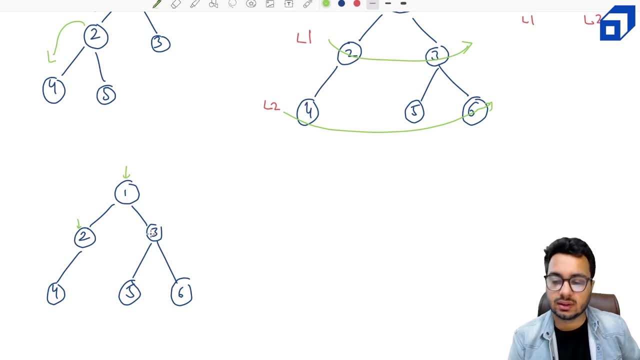 you do not have a direct way of going to 3 right. so that means with recursion it will be very difficult for us from 2 to go directly to 3 right, and if we go to 3 we don't know a way to come to 4 right. so 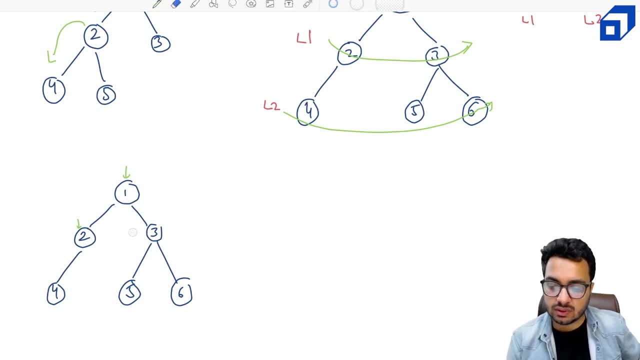 we cannot go back and forth, right. so how this is achieved? this is achieved by using a concept of a queue data structure. ok, what we will do, we will create a queue queue. you know, it is a p4 data structure: first in, first out. so in the beginning I will push this node. 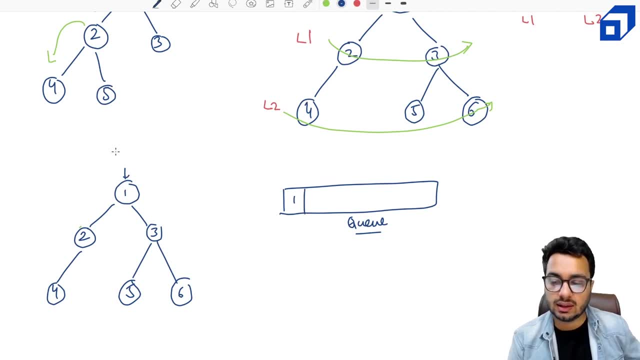 in the queue. fine, right. and then I will say, ok, like queue dot, push root. now I will pop one node from the queue, so I will pop this node and I will push the children of this node into the queue, so I will print it. output will be 1. this is: 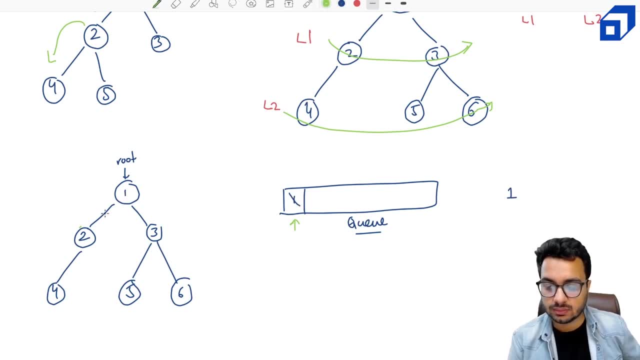 popped. and what are the children of 1? children of 1 are 2 and 3 right now. how do I know the children? because I am not going to store an integer value here. I am going to store the reference of this node, right. so I am going to say: 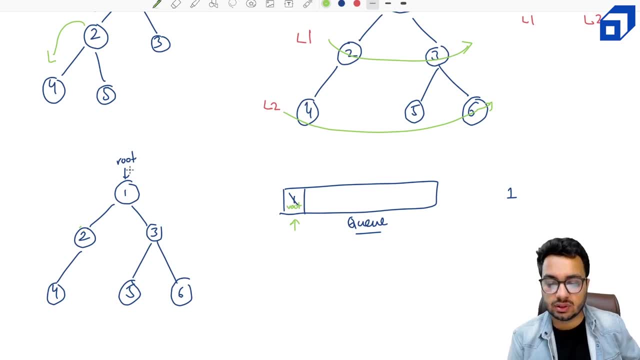 ok, this root is the address of this node is stored here. so if you know the address, you also know the child values, right? so you know the children are: root dot left, root dot right. I will push the reference of 2 and 3 in the queue right next. 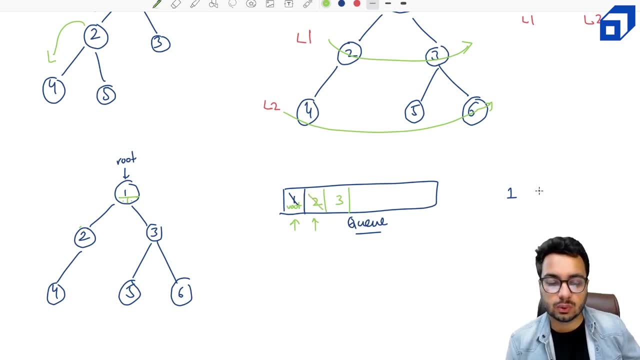 I will again pop one node. I will say, ok, let's remove 2, let us print it and let us push the children of 2 in the queue. so 2 has only one child. so 4 will be pushed into the queue right again. repeat this. 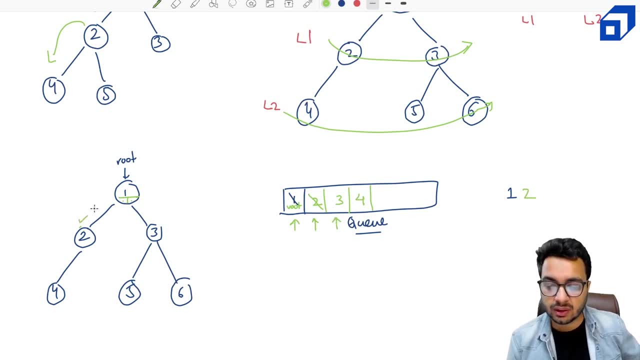 process: pop one node. so now you are going to see that, ok, 1 is done, 2 is done, the next node is coming. is 3? right? so I will pop it, I will print it and I will push the children of this 3 ok into the queue. so I will push 5. 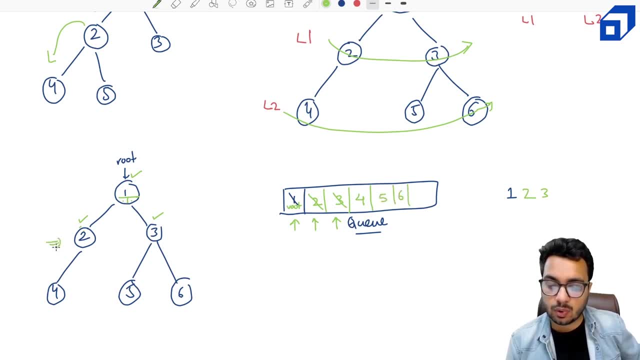 6. so you look carefully when the second level or the first level is popped. the next level is already in the queue, right? the next level is already in the queue. let's say I have some more nodes. let's say I have 7, 8 and 9, right, so let us just 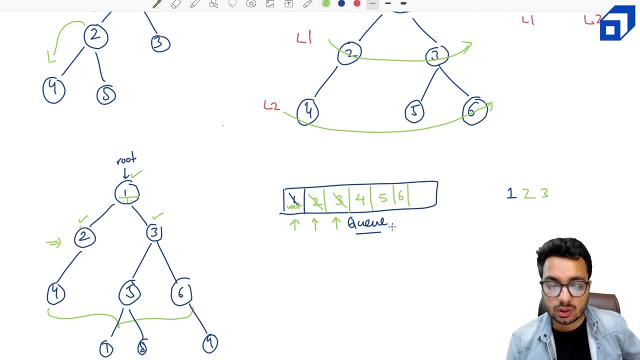 extend this example a little bit now. I will pop 4. I will print 4. this will be removed. 4 does not have any children, so nothing will be pushed. next I will pop 5. I will print 5 and I will push the children of 5 into the queue. so I 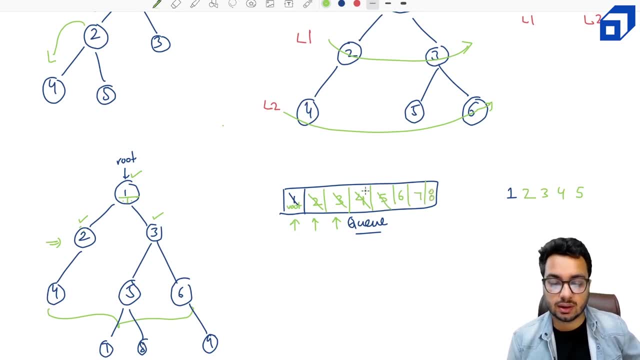 will push 7 and 8 into the queue. right next I will pop 6. I will print 6 and I will push the children of 6 into the queue, so 9 will get into the queue. next I will pop 7. I will print 7. 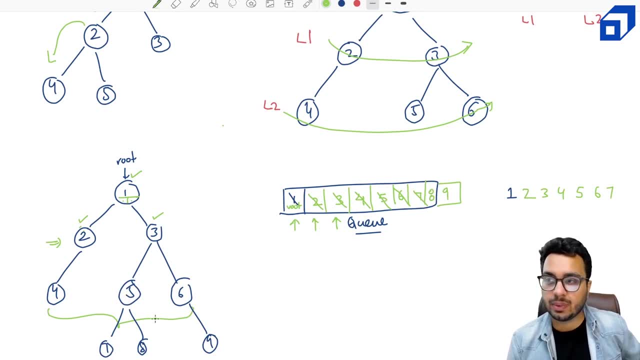 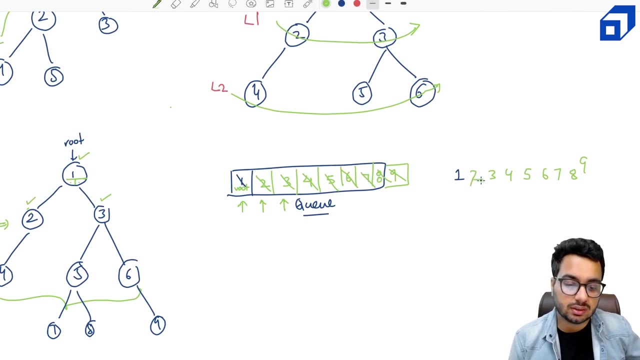 and no children, so nothing will happen. next, I will pop 8- print 8- no children. nothing will happen. I will pop 9- print 9, and the queue is empty, right, so no children. so queue is now empty. this will be my output of level ordered reversal, right? I hope you are. 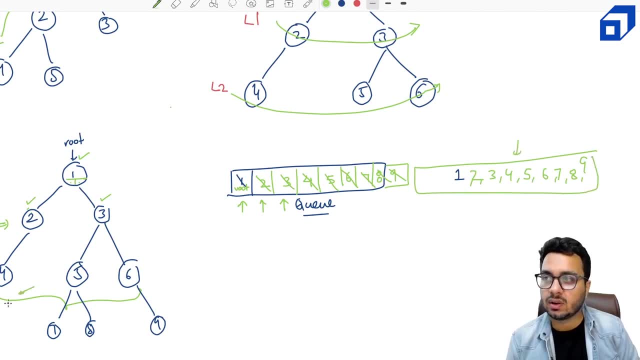 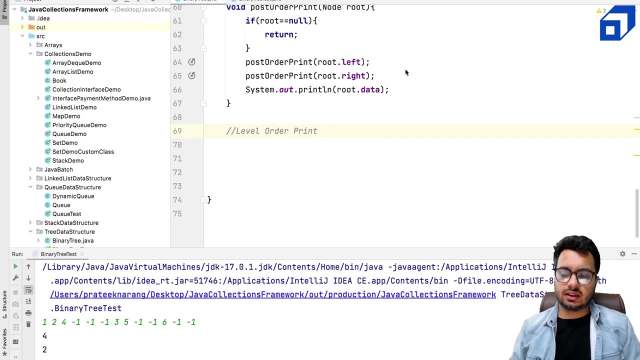 convinced that this is the correct output for this tree right now. let us look at this implementation in our code as well. let us discuss the implementation of level order print. so I am going to create a method called as void, level order print, and first of all I will need a queue object. 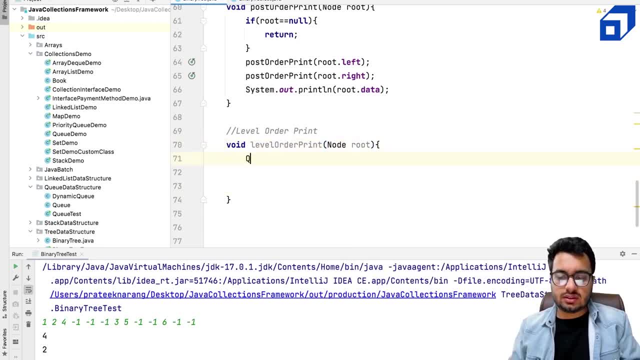 right and I also need to pass the root here, so I will say, ok, fine, I will need a queue of node called queue. this is equal to new linked list. so in java, queue is a interface and linked list is a class that implements the methods of the queue right. 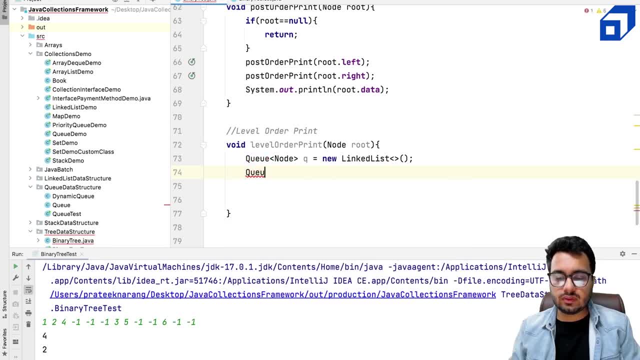 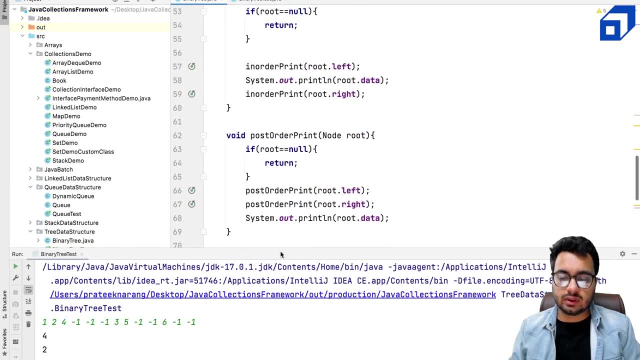 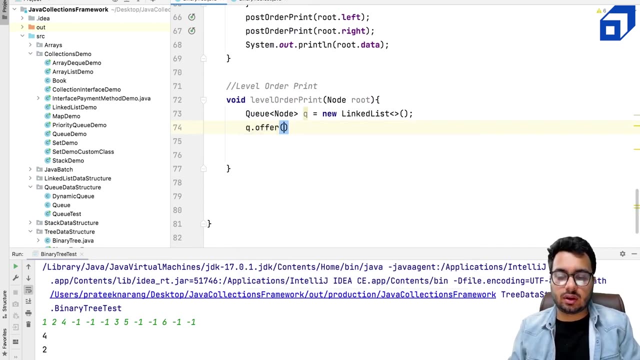 we need to import this from the ah util package. ok, so linked list is imported. queue interface is also imported. so to start with you can say, ok, queue dot offer. that is your add operation right. and I can offer root inside the queue. that means I can add queue right. 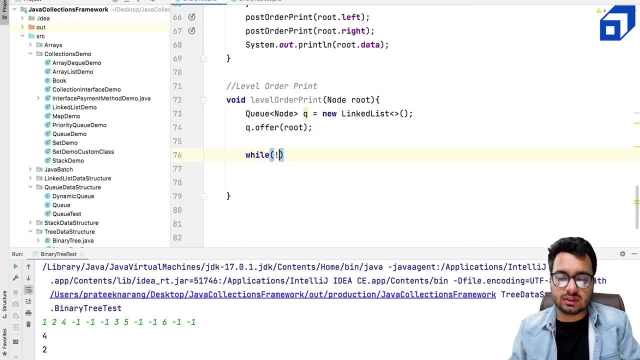 now, I said you will do some work while the queue is not empty. so, while the queue is not empty, what you will do? you will pop out something. you will say: ok, give me the node which is at the front of the queue, node f. this is equal to: 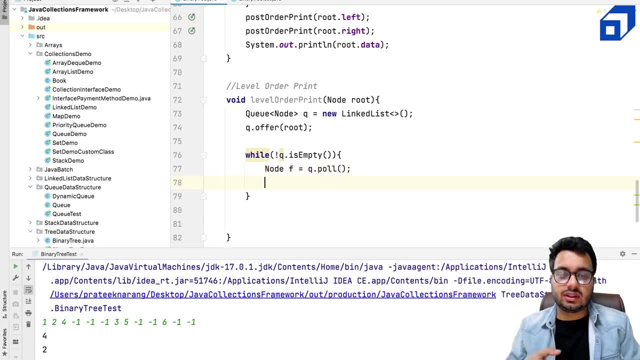 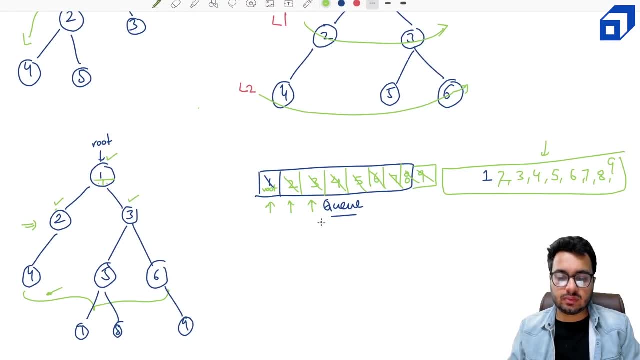 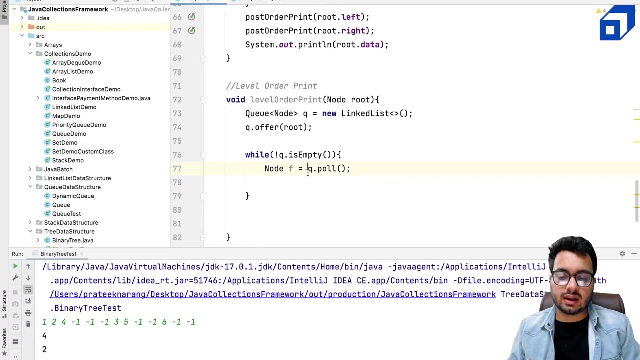 queue dot whole right. so this removes the first node. like we have seen in the diagram, we are always removing the node at the front of the queue right, so this is going to remove it and return it. right now I can print the data of this node so I can say: s out. 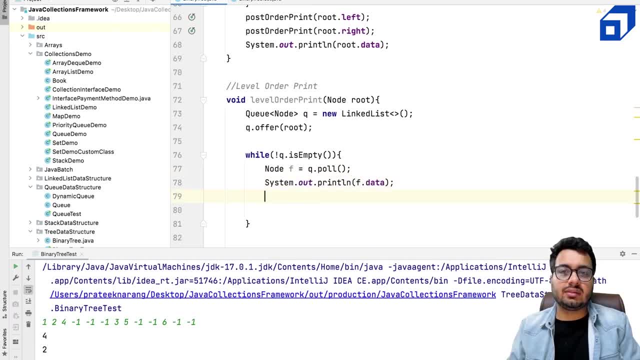 f dot data. and now I can check if the left and the right side. if they are not null, I can push them into the queue. if f dot left is not null, I will say queue dot, push f dot. sorry, queue dot. offer f dot left and if the right. 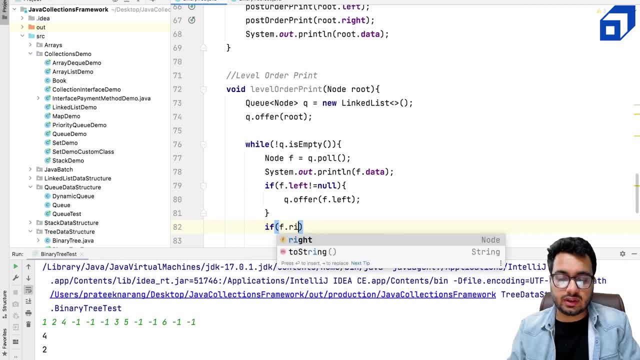 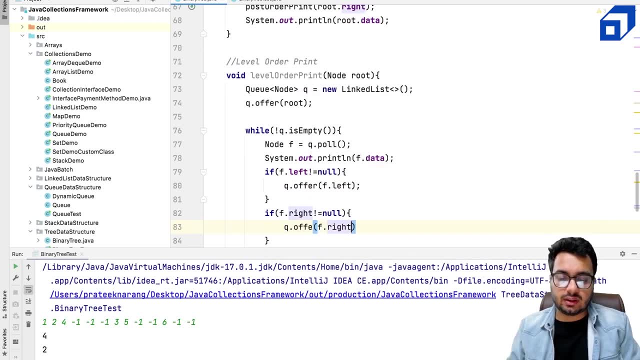 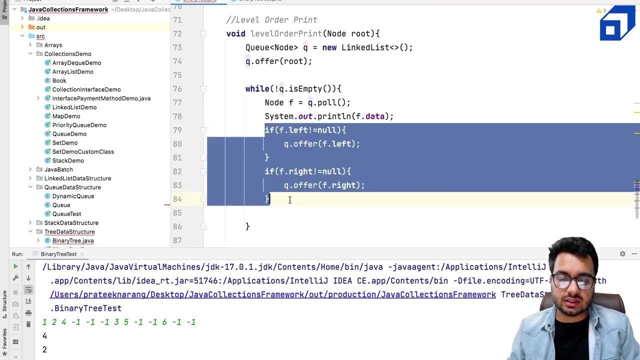 child is not null. sorry if yeah, if the right child is not null, I can say: queue dot, offer f dot, right. so in this way, queue is getting filled using these if conditions and it is getting empty from the front using this whole operation. right, that's all that. 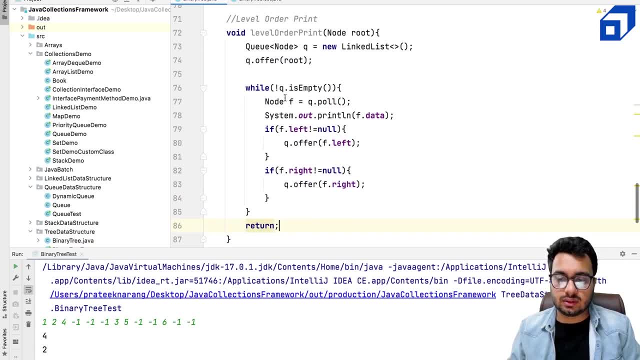 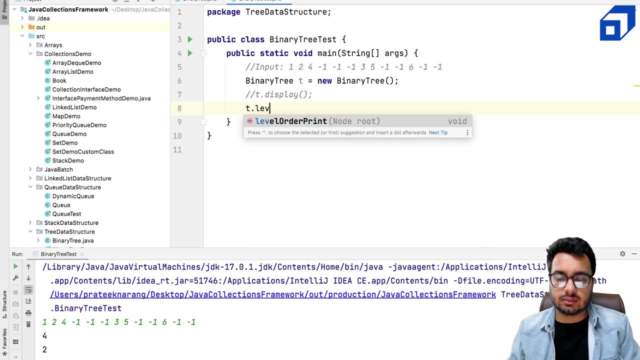 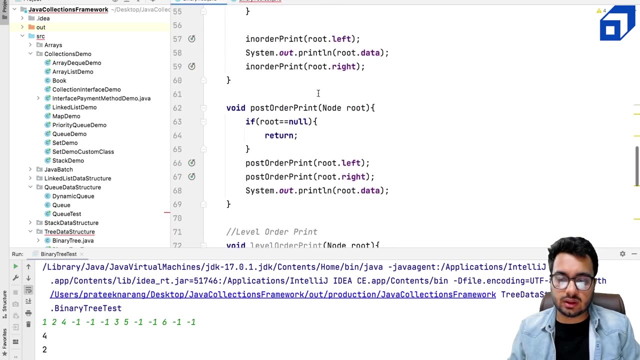 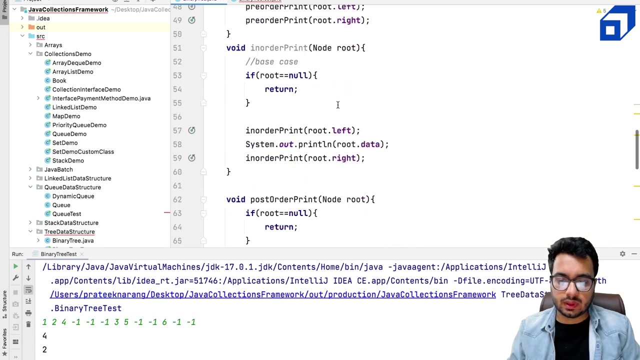 is the code. and now I can just run this code in the display method. or here I can say: t dot level order print: ok, root. so it's better to call it internally because root, I don't want to access it outside, so, ok, I will just call it from the. 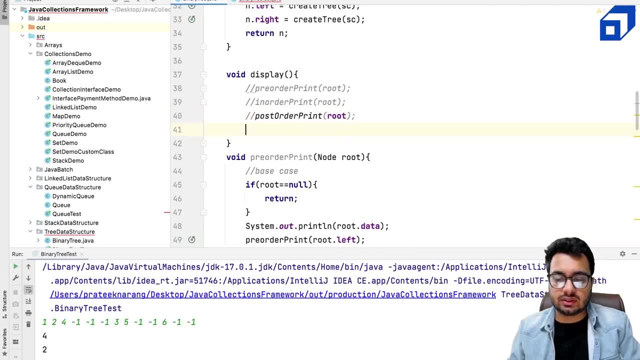 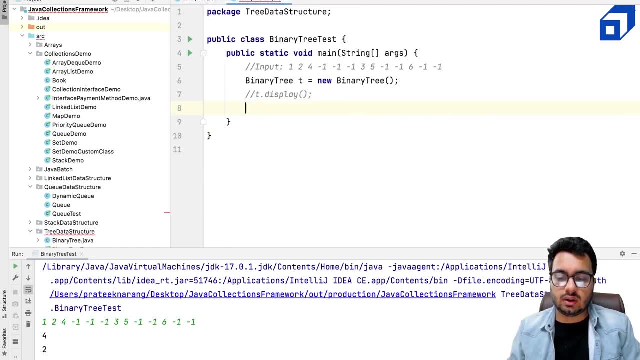 display method because we are testing the functionality so I can say level order print. so here I can just call t dot display. so now my tree will be displayed in a level order fashion. let's see what output do we get for the given tree. I am getting one, two, three, four, five, six. 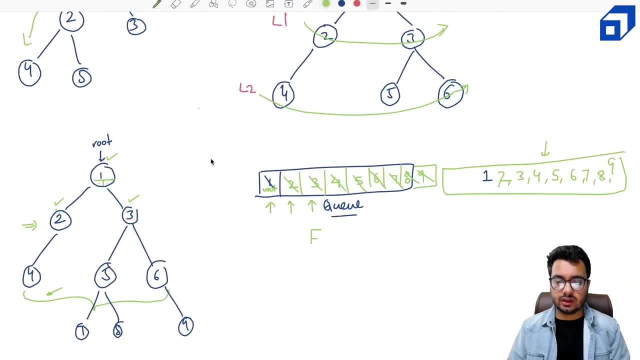 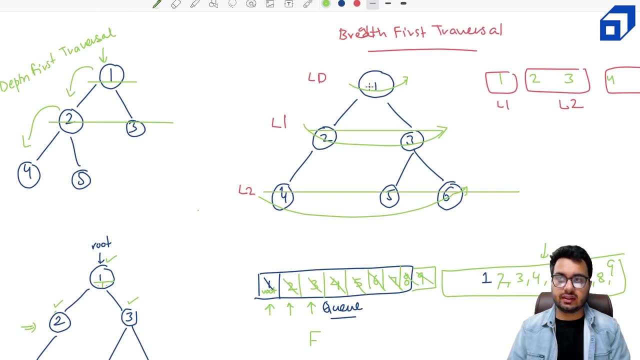 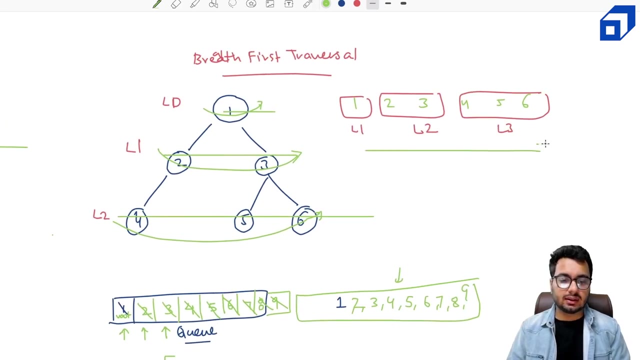 which is correct. and if you look carefully here for this tree, I am getting one, two, three, four, five, six. yeah, this is the tree actually, so I am getting the correct output, which is this. so I hope you understand the level order traversal and how it is achieved using the.